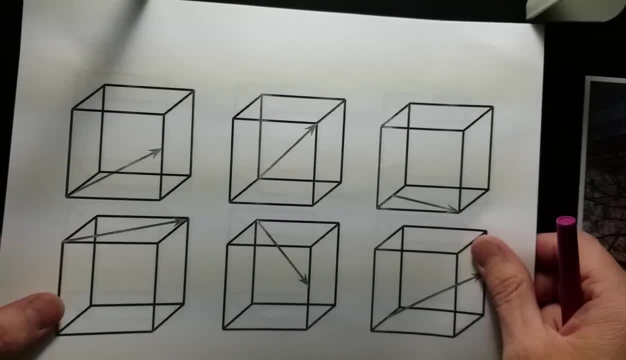 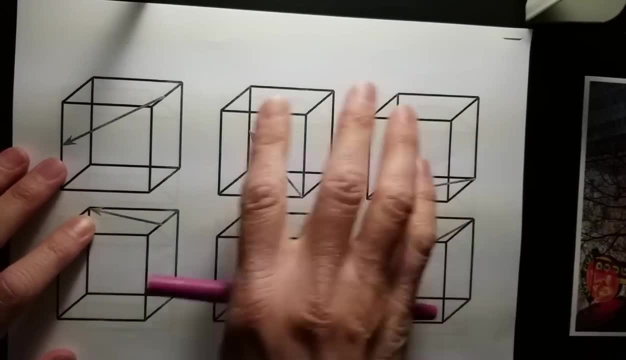 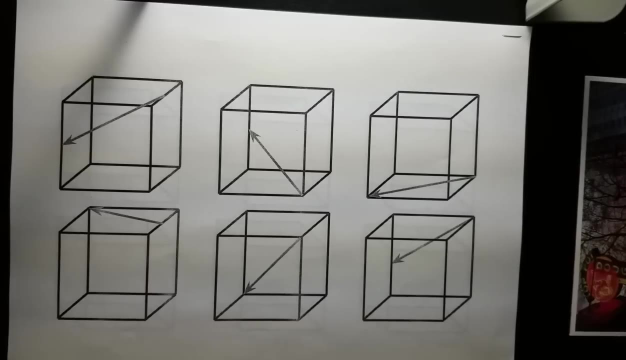 might hold it like this instead. It's all good. You can always, in fact, turn the sheet upside down if you want to have more problems to solve, but this is the way that I'm going to be working with them. So, on this first page, our job is to identify the directions. 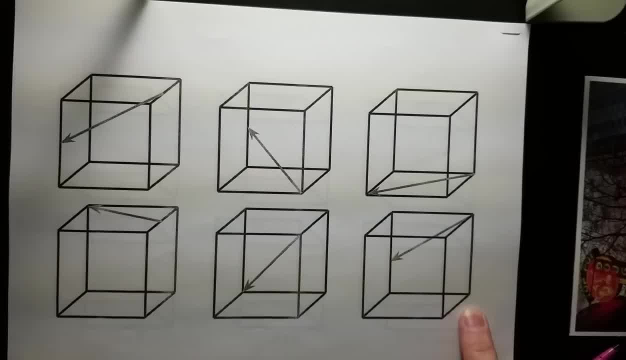 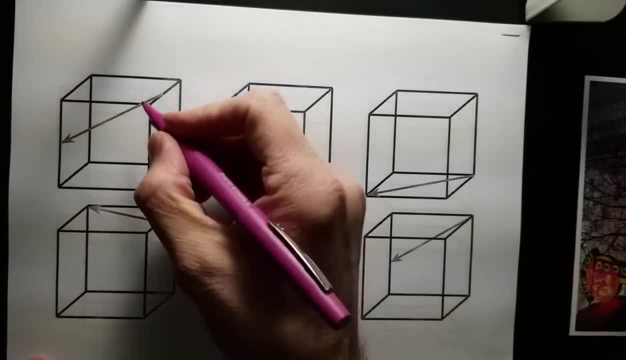 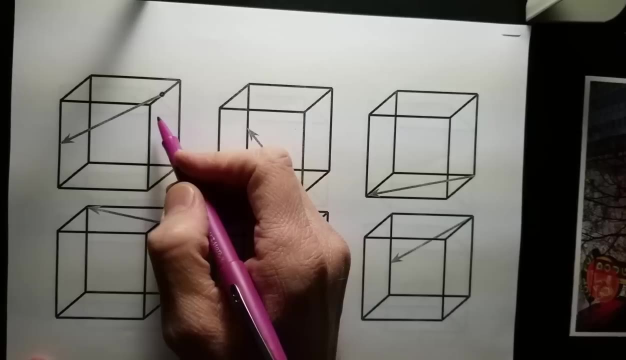 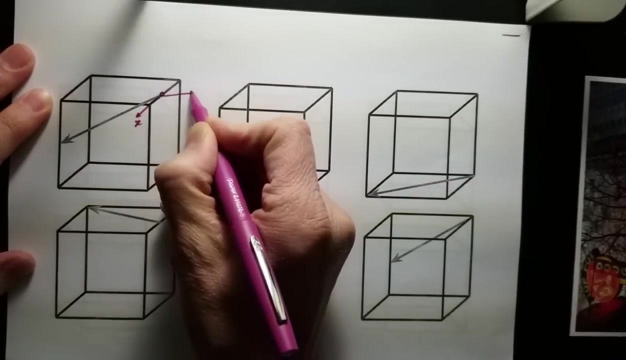 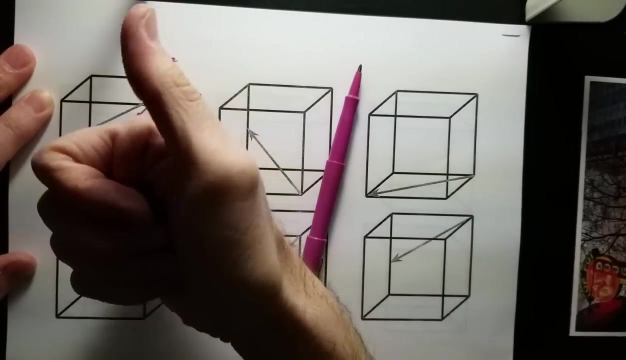 that are shown here, And the way you do that is: you look at the direction that's drawn, you identify the tail and that's where we're going to put our origin. So x, y, y, y, y, x, y and z. So we got a right-handed coordinate system. 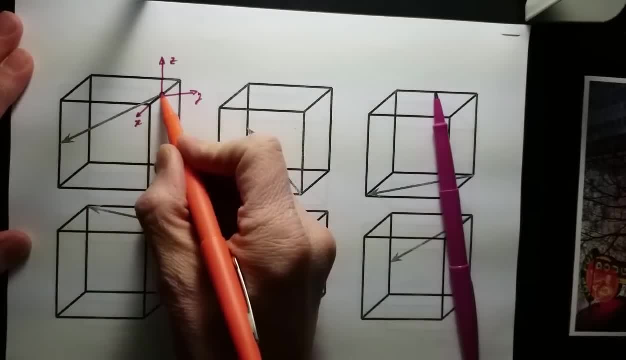 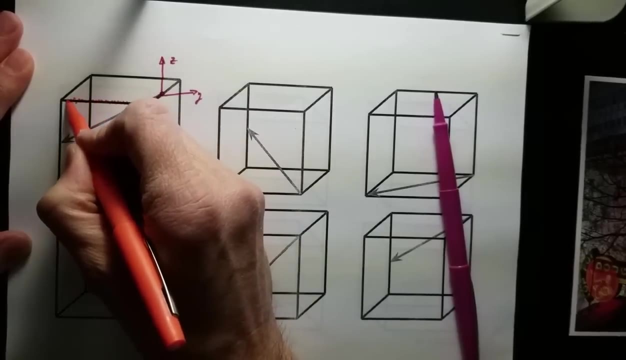 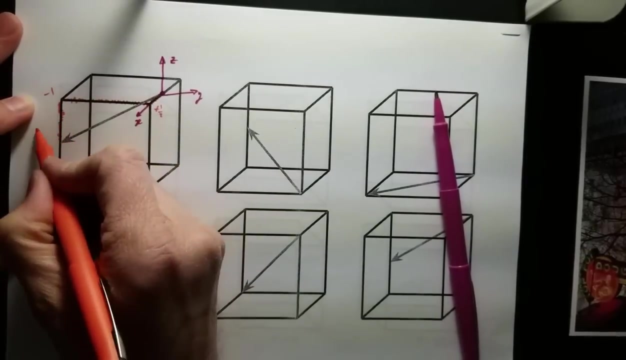 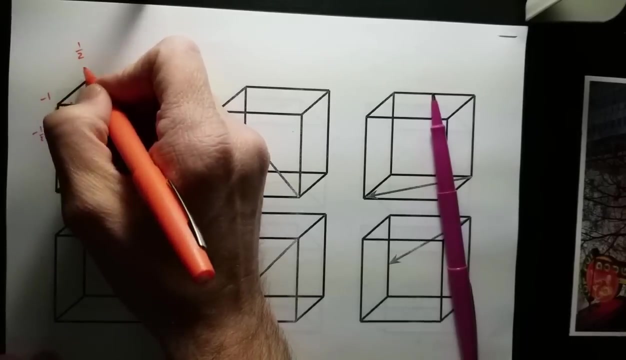 And then, in order for us to get from the tail to the tip, we're going to go by plus x, minus x, 1y and minus 1 half z. So we went 1 half minus 1 minus 1 half. 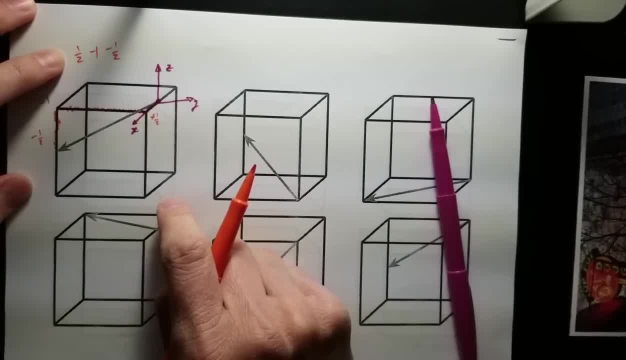 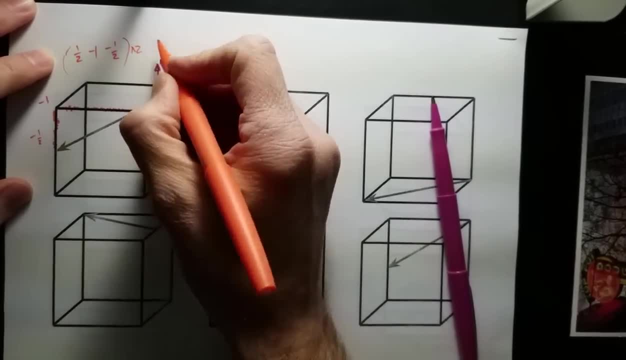 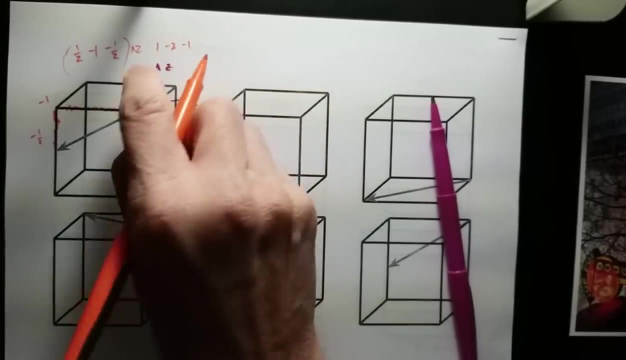 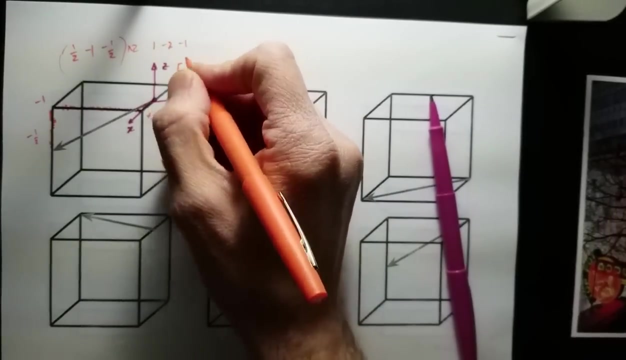 And we can't have fractions. so we multiply this all by 2 and that gives us 1 minus 2 minus 1.. And then we put this in the correct form. So the correct form is going to be, in square brackets, 1, 2 bar, 1 bar. 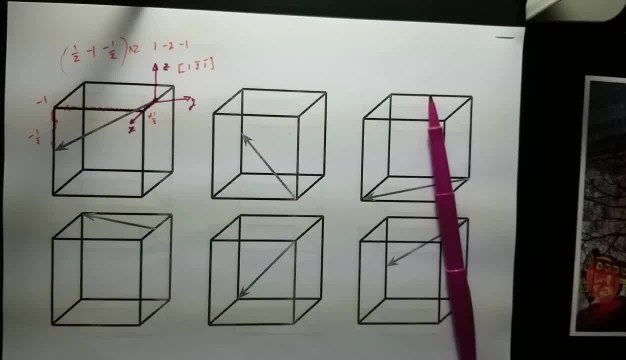 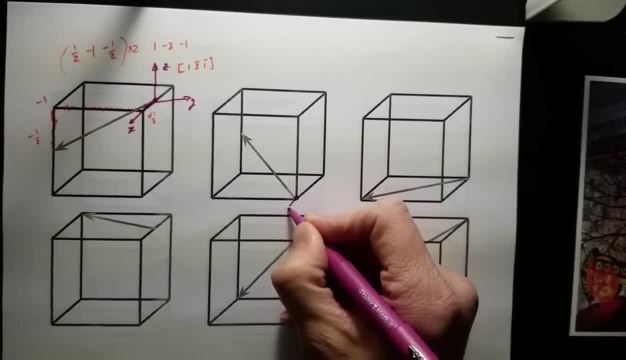 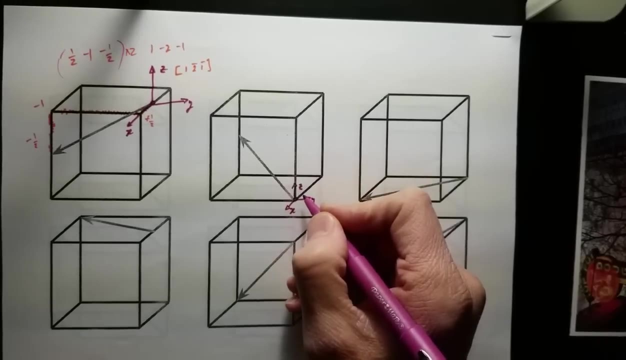 And that is the first vector. So going to the next one Again, picking this as our the tail, as our origin: x, y, z. To get to the the tip of the vector of the arrow, we have to go minus 1 x. 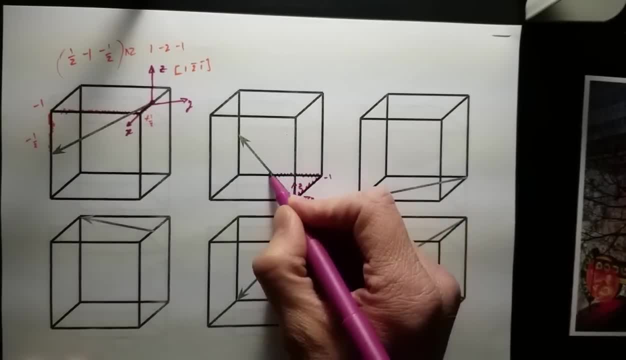 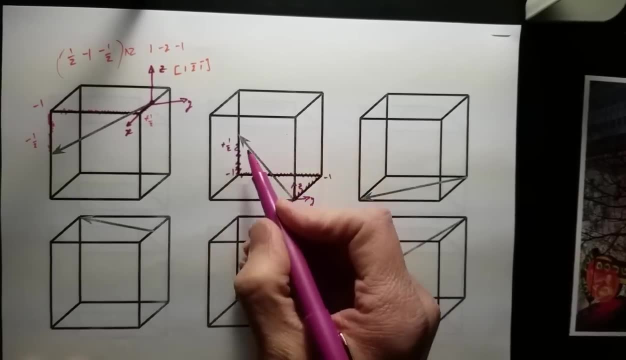 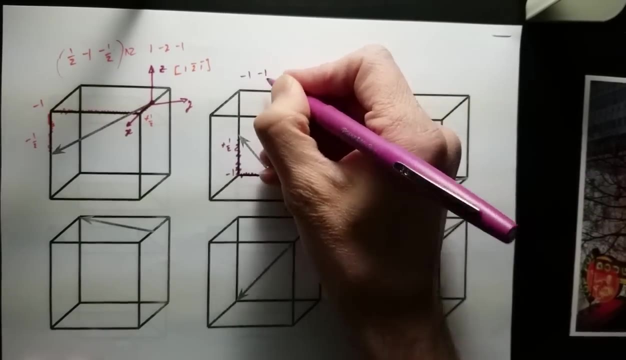 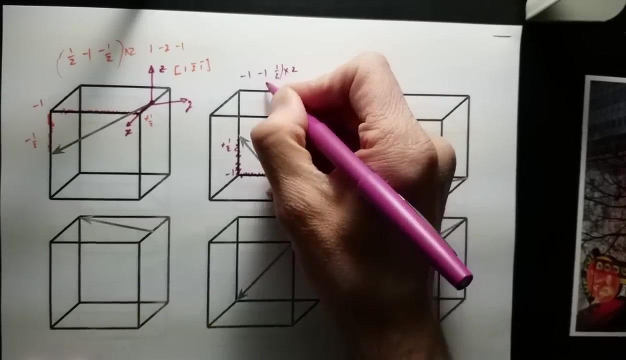 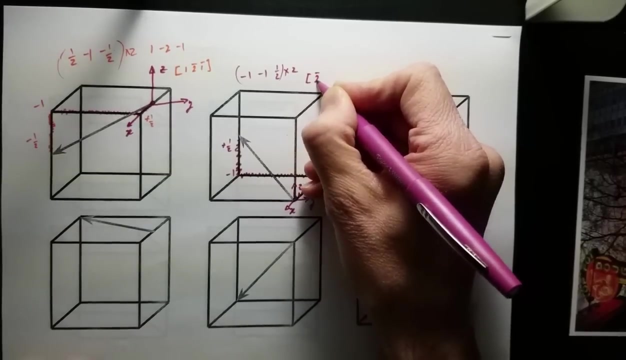 minus 1 y plus 1 half z. So that's going to be minus 1 minus 1, minus 1, 1 half. to get rid of the fraction, we multiply by 2 and that's going to give us 2 bar 2 bar 1.. 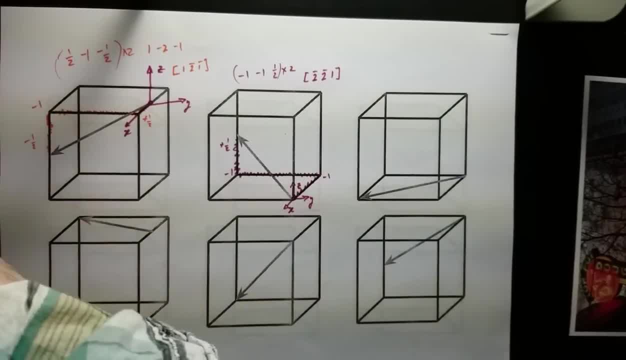 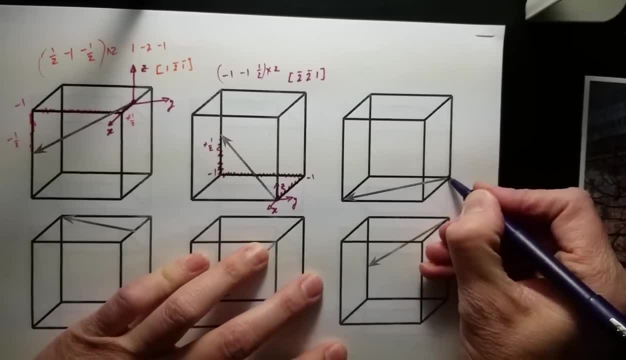 So we have 2 bar: 1.. 1 bar I, 1 bar z, x, 2 x, x2.. Okay, let's go to the third one, picking the tail as the origin: x, y, z, to get to the. 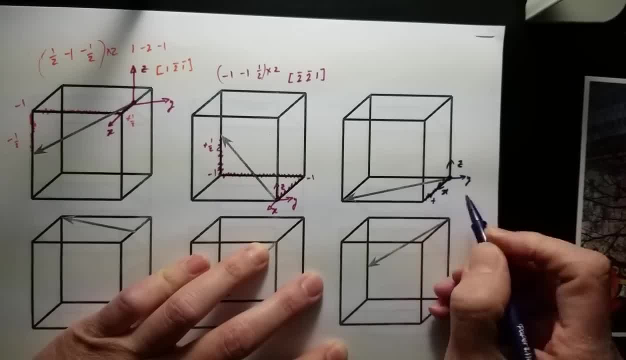 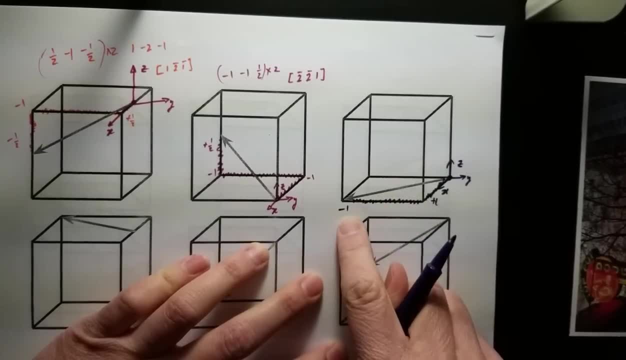 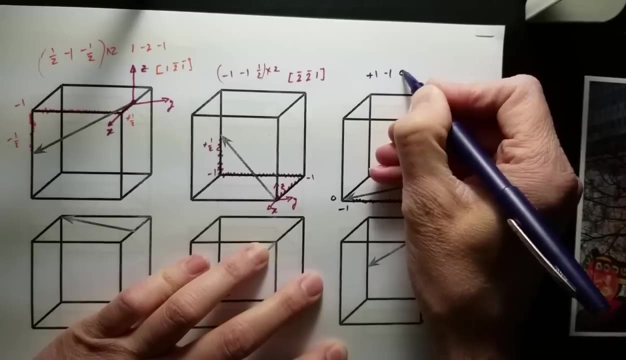 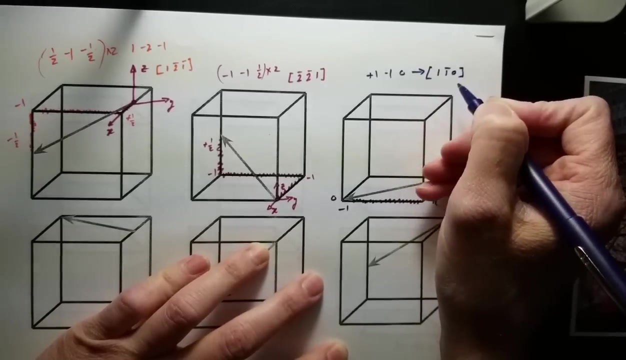 tip: we go plus 1, x, minus 1, y and 0, z, So plus 1,, minus 1, 0, which is 1, 1 bar 0.. Okay, going to the 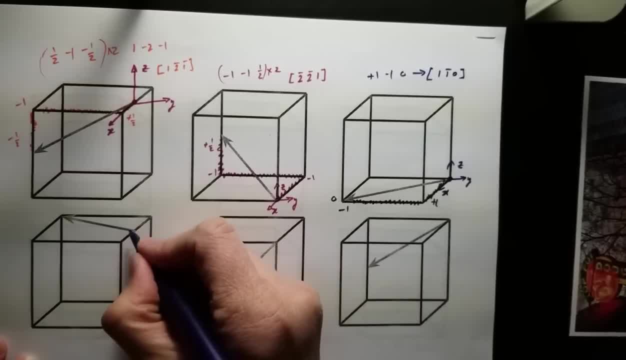 fourth, defining the tail of the arrow as our origin- x, y, z- we have to travel minus 1 half x, minus 1 y and 0 z. So minus 1 half, minus 1, 0,. multiply by 2 to get rid of the fraction. 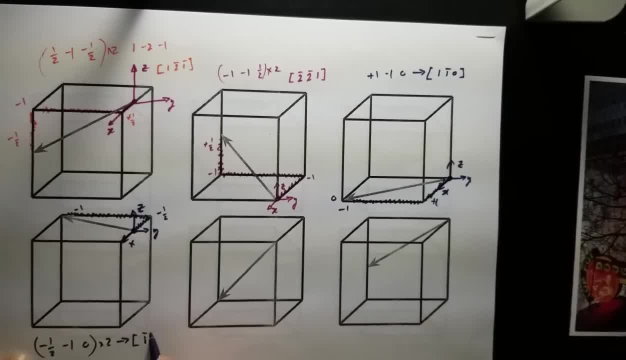 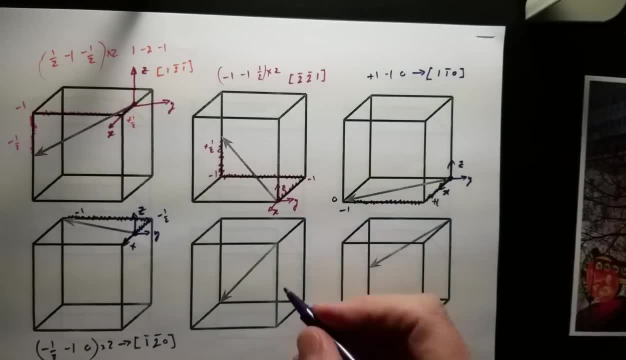 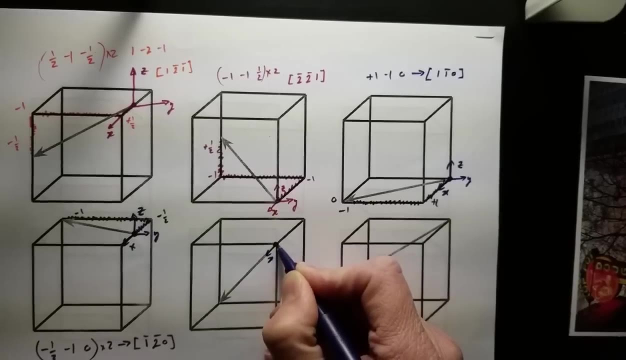 and that gives us 1 bar 2 bar 0.. Okay, the fifth vector, fifth arrow, setting the origin x, y, z. to get to the tip we have to go minus 1, x minus 1 y. 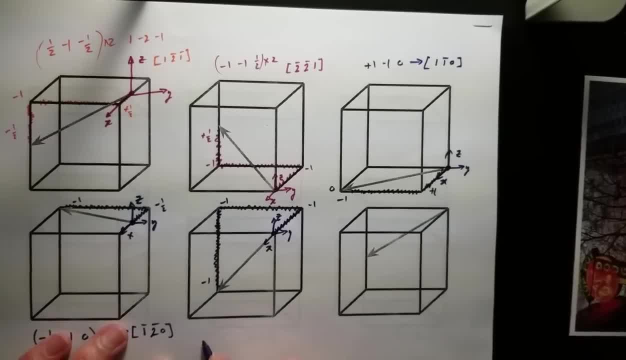 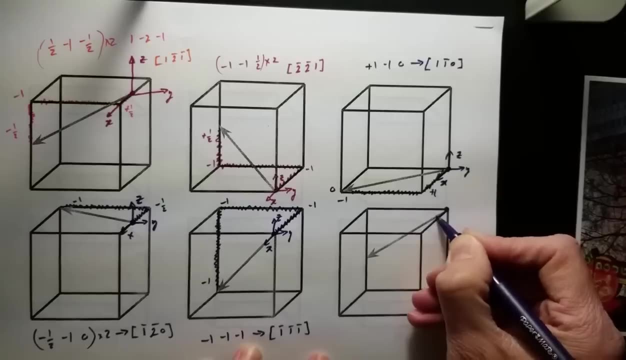 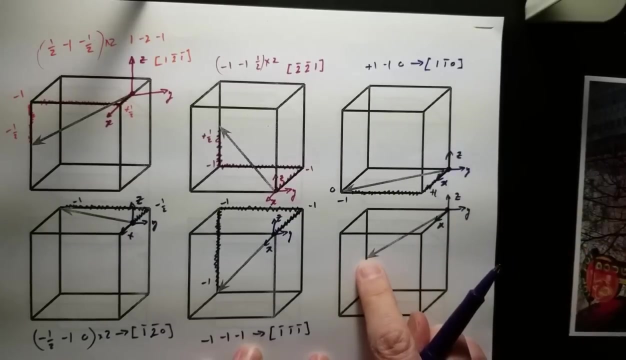 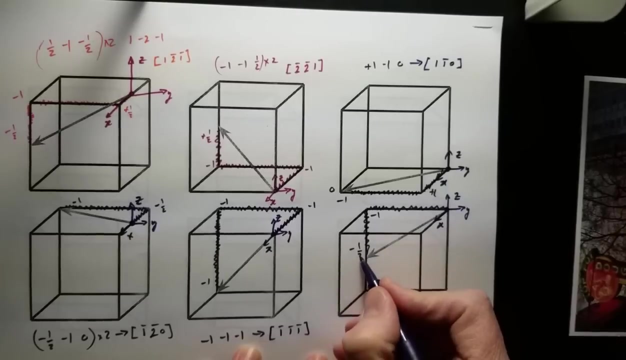 minus 1 z, So minus 1, minus 1, minus 1 is 1 bar, 1 bar, 1 o'clock bar. And the last direction: x, y, z. To get to the tip we go 0, x minus 1, y minus 1 half z. 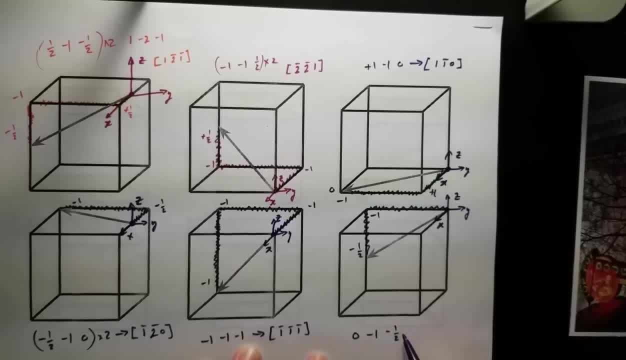 So that's 0, minus 1, minus 1, half multiplied by 2, to get 0, 2 bar minus 1, y minus 1, 1 bar, again in square brackets. So that's how we identify these directions. 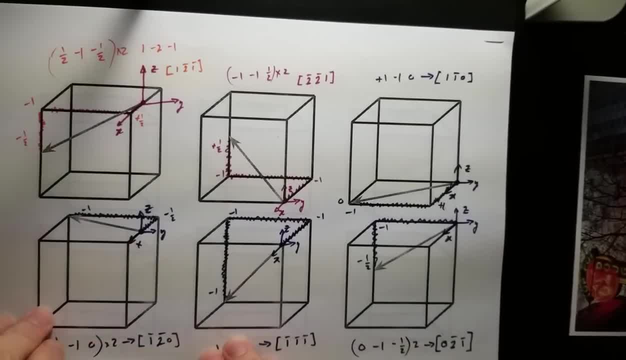 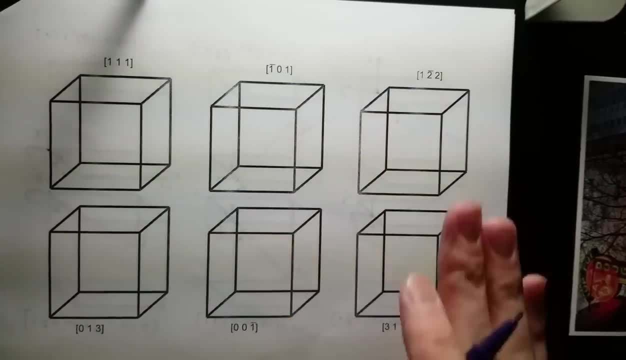 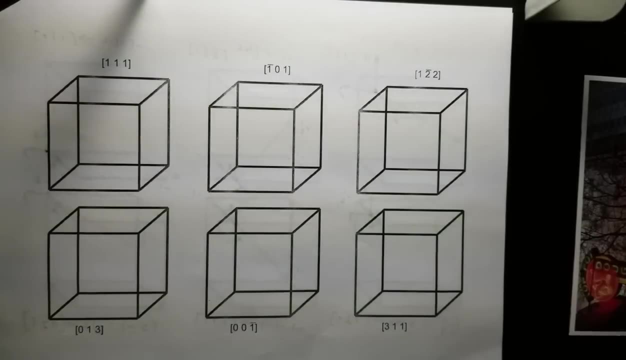 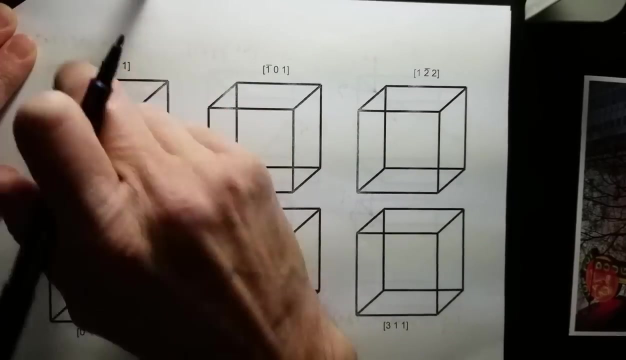 Okay, let's go to the next page. And the next page we're going to draw in the directions. So we've got square brackets. we know they're directions, Okay, So we're going to go 1,, 1, 1.. 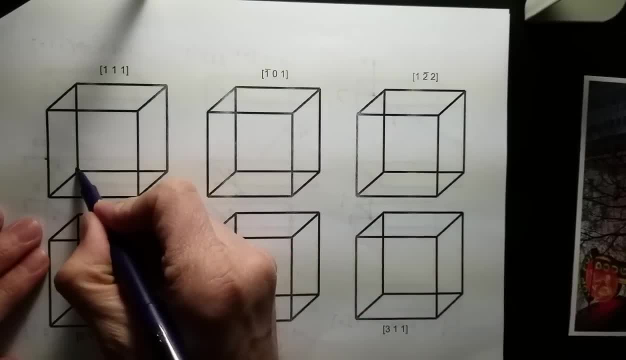 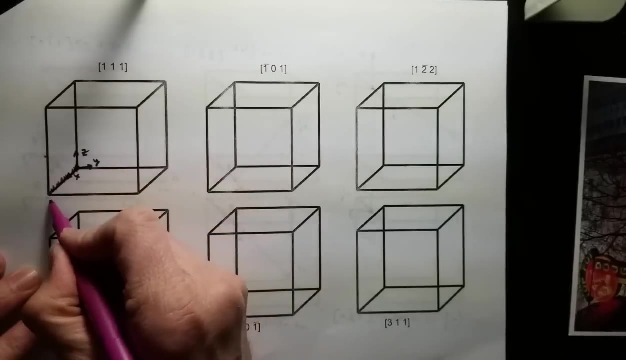 And it's fairly easy for us to start in this back corner as our origin x, y, z, So we can go plus x 1. x 1. 1. Plus y 1. Plus z 1.. 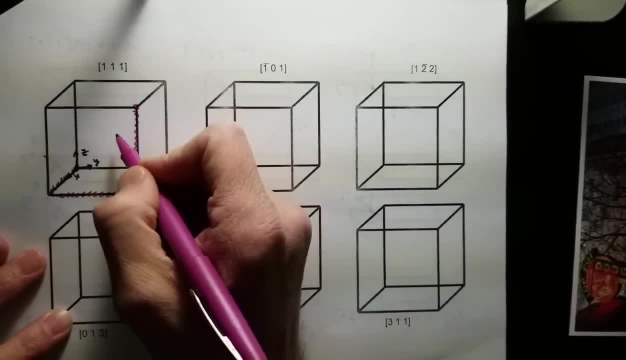 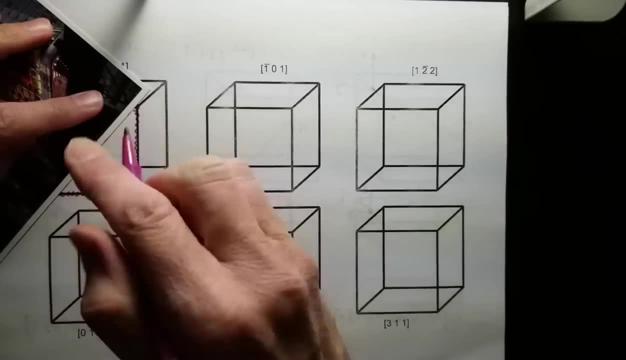 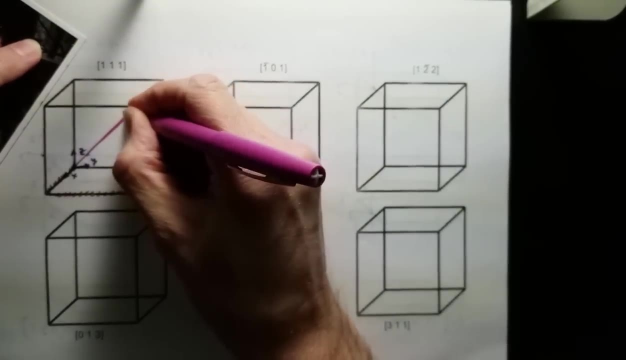 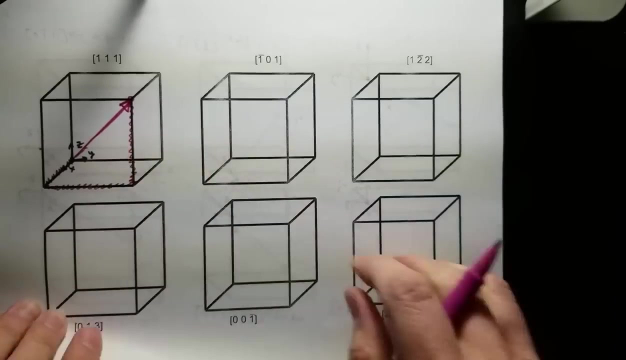 And our vector. we start with the tail, at the origin and the tip, where we ended, And that is our 1, 1, 1 direction. Notice, the 1, 1, 1 direction is that way, And the 1 bar, 1 bar, 1 bar is exactly the opposite. 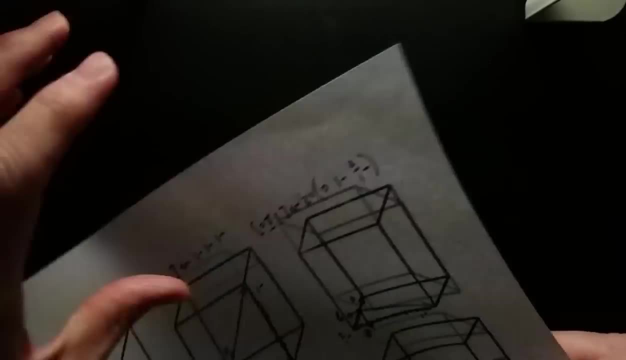 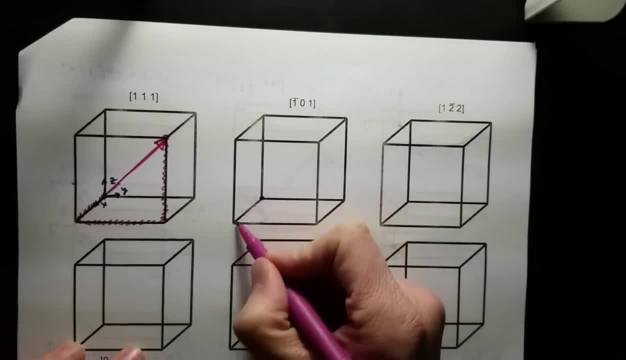 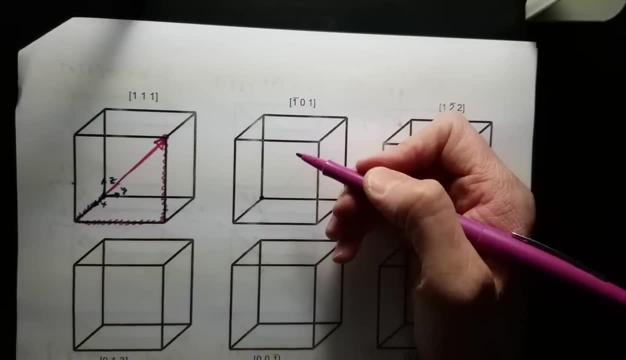 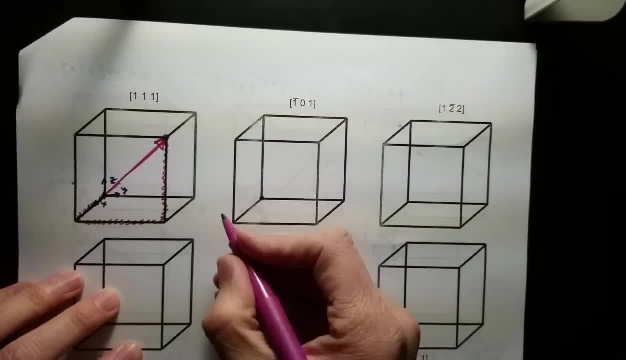 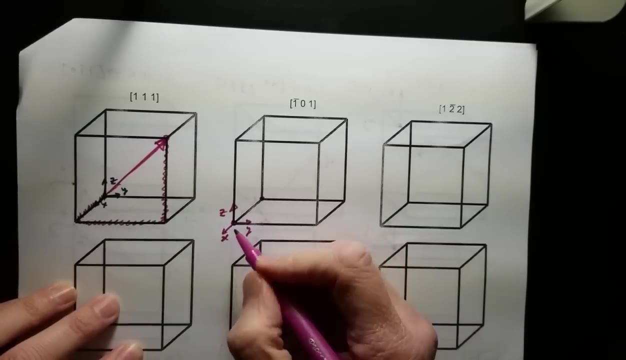 So we could start back here in the back corner again. But if we do that, it's really tough for us to draw negative x right, because we have start over here. so let's, let's pick. this is our origin: X, Y, Z. so now we say that: 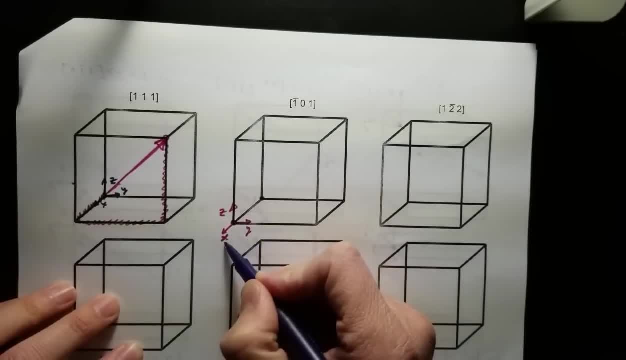 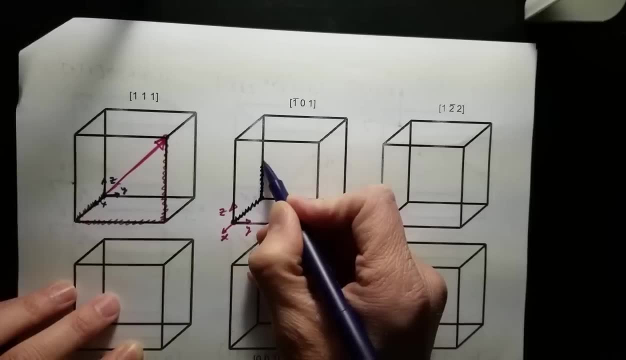 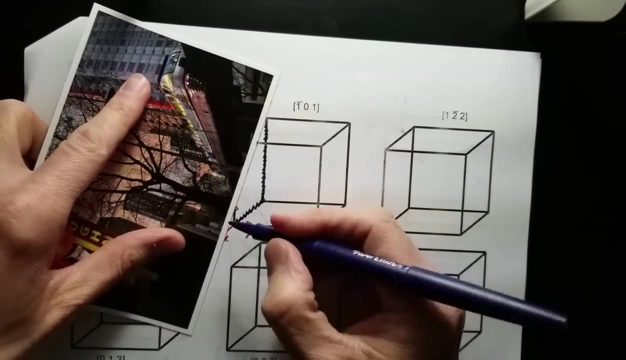 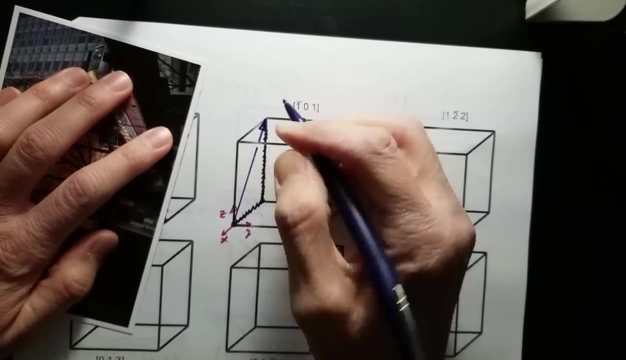 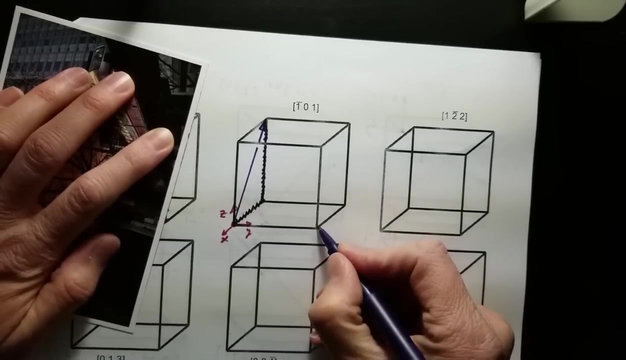 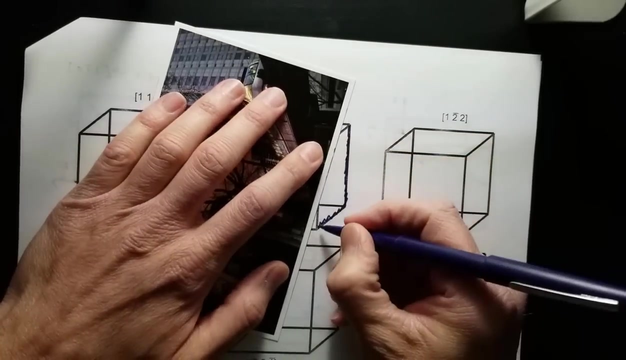 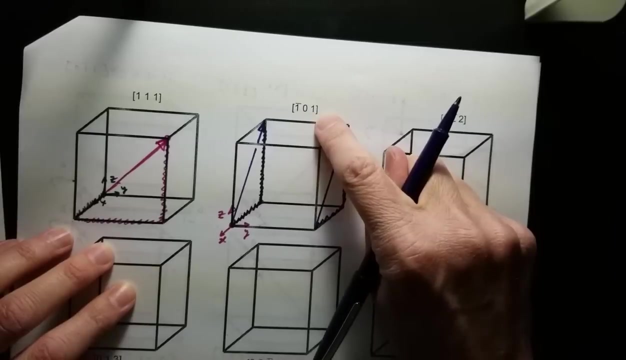 from the origin. we go minus 1 X, we go 0 Y and we go plus 1 Z. so that makes this our direction. now you should note that if we picked this is our origin instead, well then we go plus X, plus Z, and we'd have that. these two are exactly the same. 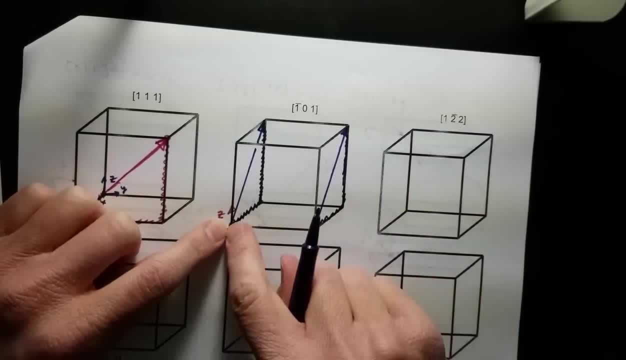 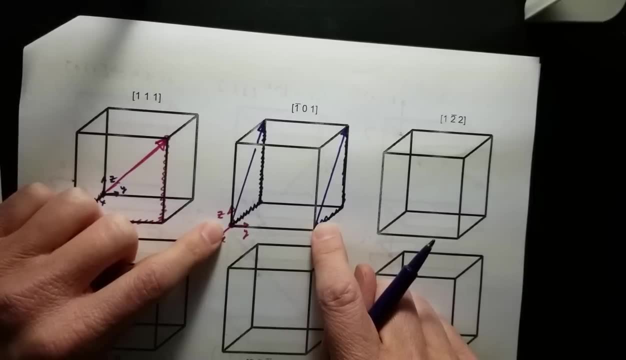 direction. I mean they run parallel to each other. so it doesn't matter where you draw the origin. you're going to wind up with the same vector and the way you draw the origin is going to be the same vector and the way you draw the origin is going to be the same vector. and the way 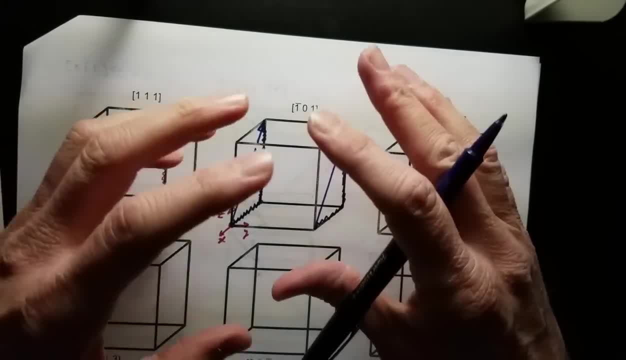 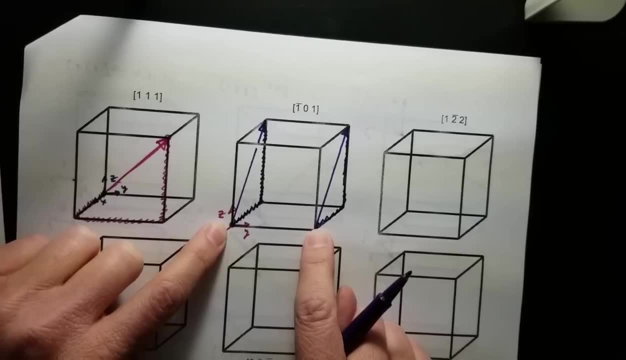 that you should think about this in terms of a crystal is if you imagine yourself taking this crystal and rotating as you're looking in that direction. well, whether you look here or here, or here or here, you're going to have the same picture. so the directions are basically telling you: so okay, you're. 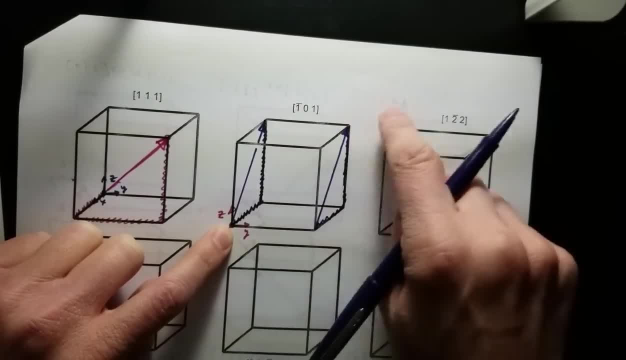 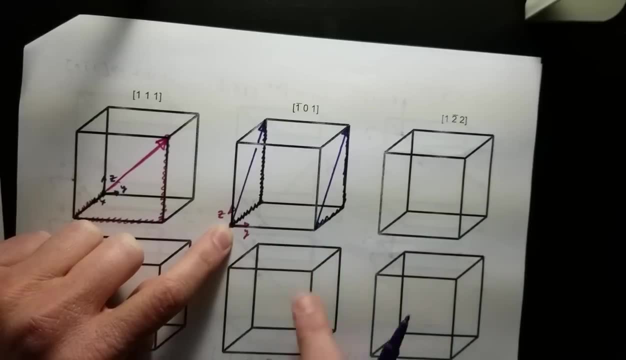 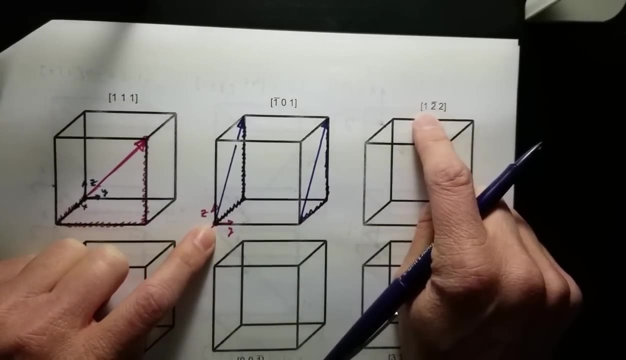 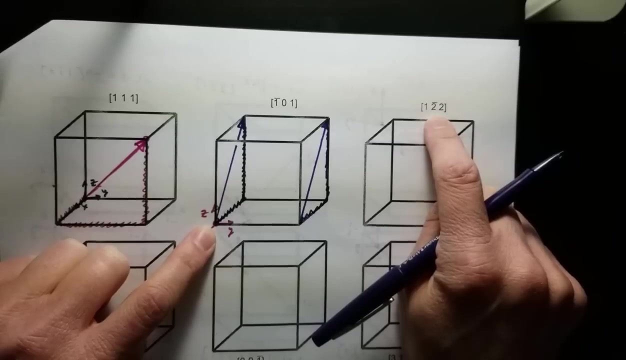 standing inside the crystal and you look in the- you know- HKL direction, whatever those vectors, whatever those numbers are. well, it doesn't matter where the origin is, you're going to have the same picture. so now let's go to third. so that gives us a 1, 2 bar 2 and we have a number. 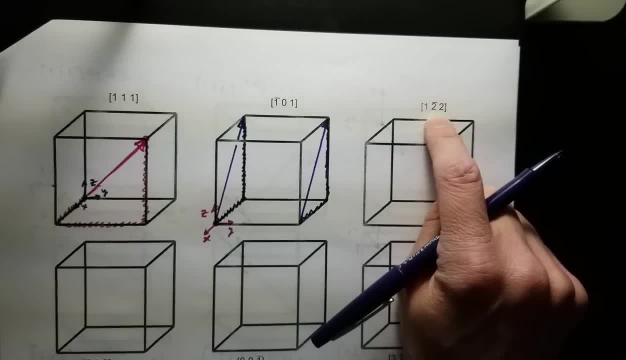 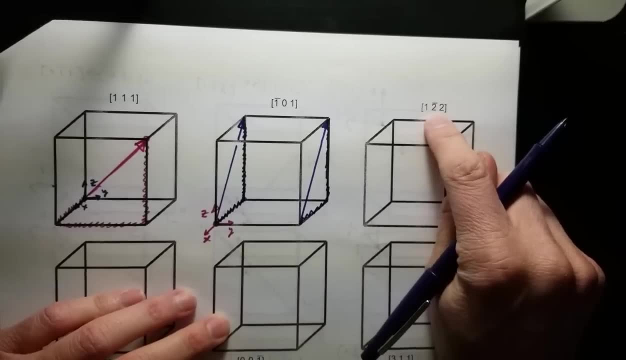 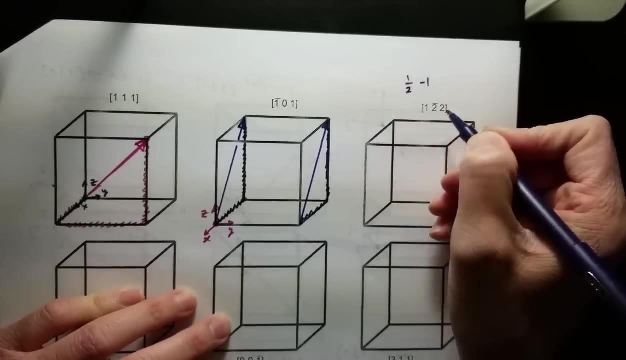 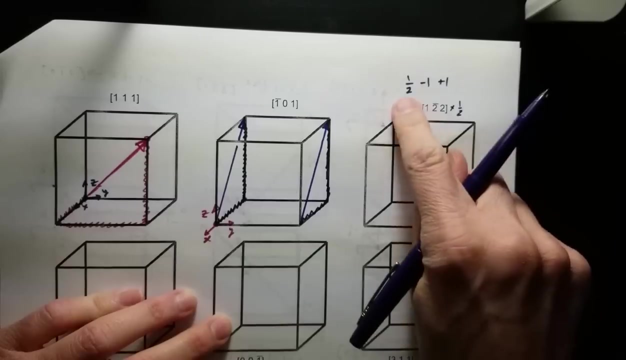 larger than 1. so in order to get rid of that, in order to make it possible for us to draw our entire vector inside the unit cell, we're going to divide by 2, so we're going to have 1 half minus 1 plus 1, if you say, take that by 1 half, so now we have all of our values less than. 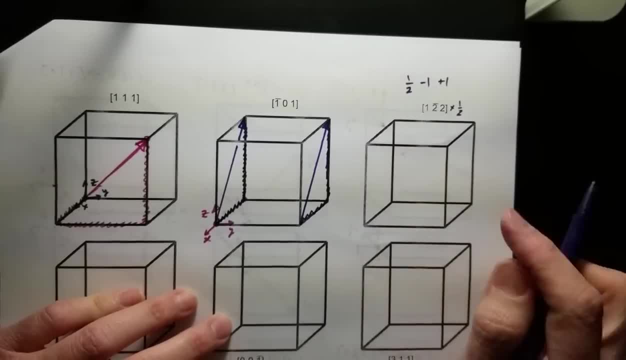 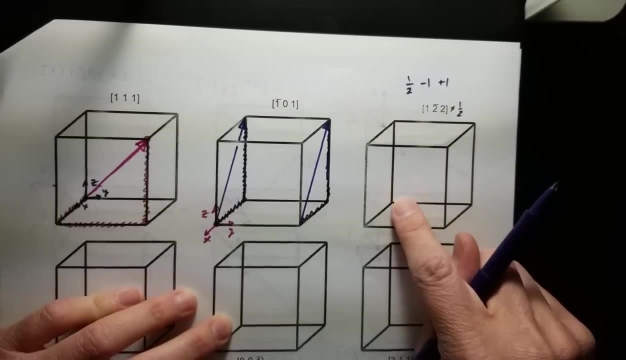 all of our values less than 1, and so X is in the in the plus direction, so we can start back in the back plane. Y is negative, so if we start over here, then we're going to be drawing vectors over on this side, so instead we're going to 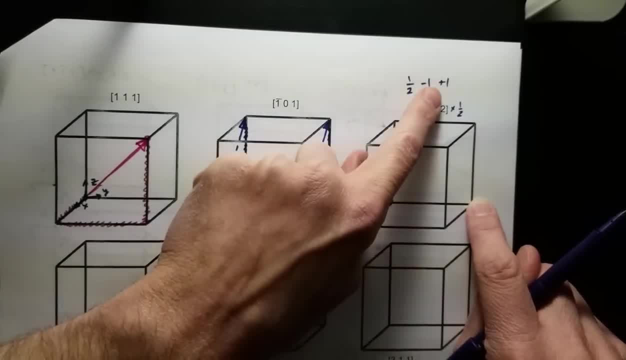 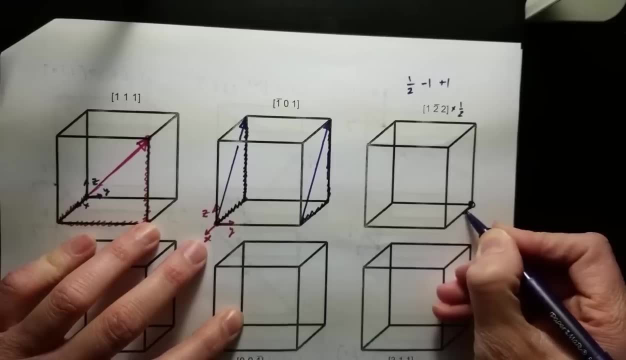 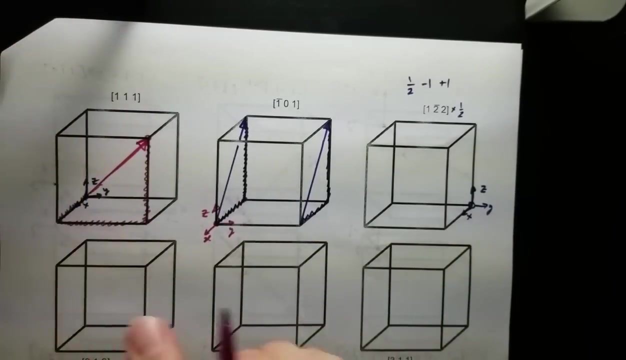 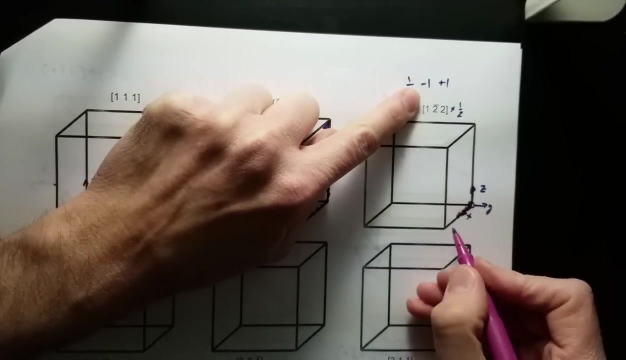 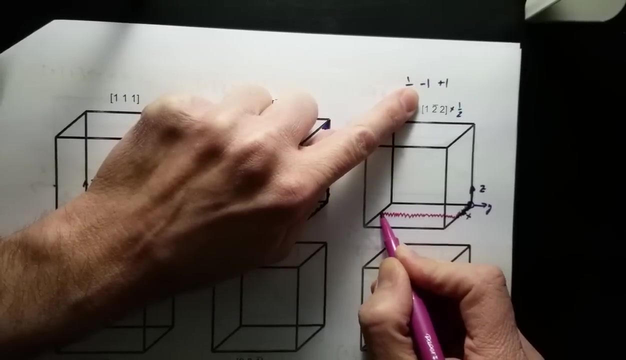 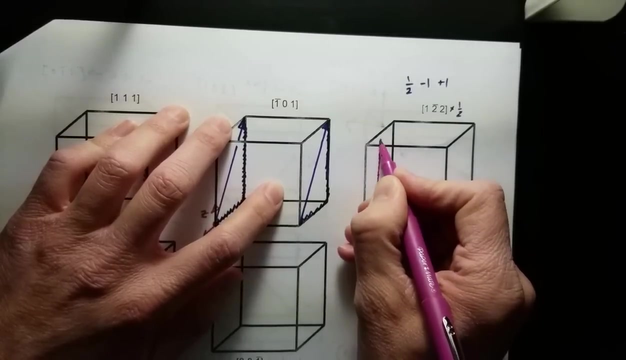 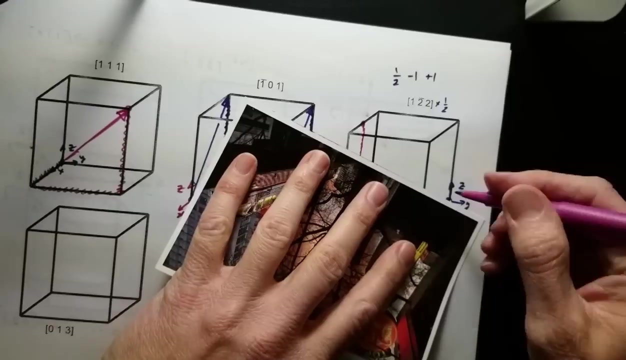 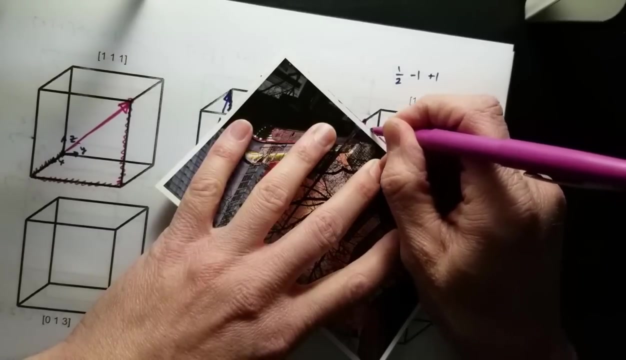 push ourselves over to this area and then our z is plus. so we'll start in the bottom. so we'll have this as our origin- X Y, Z- and says we go one half X, 1 half minus 1y and then plus 1z. So that's the tip of our vector, or the tip of our direction. 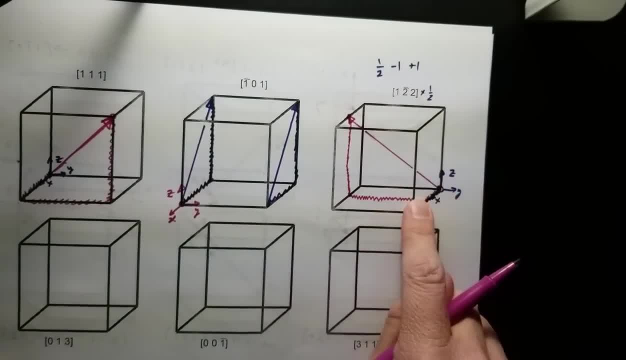 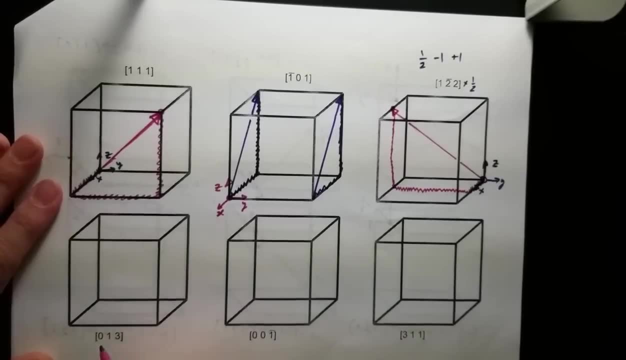 So this is the 1,, 2 bar 2 direction. Coming to the 4th, again 3 is bigger than 1, so we multiply by 1, 3rd, and that's going to give us 0, 1, 3rd, 1, they're all positive. go to the back left corner: x, y, z. 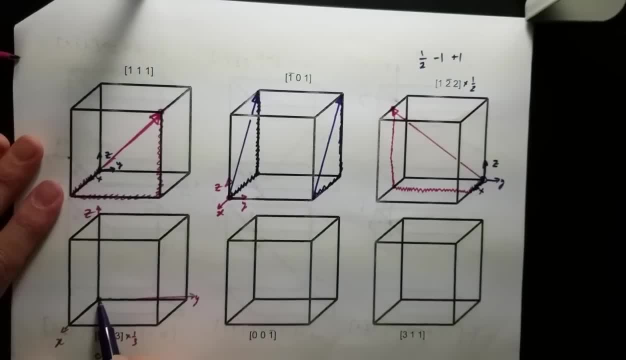 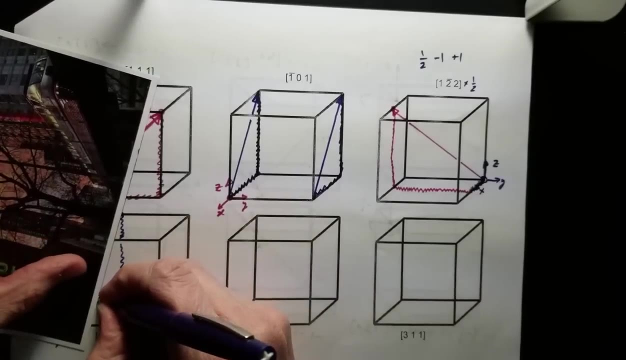 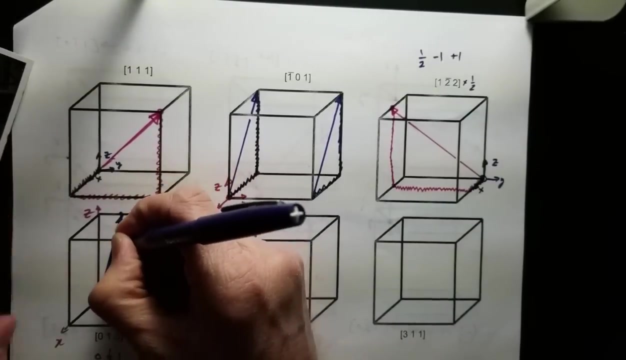 So if we go 0 in the x direction, 1, 3rd in the y direction- Am I right there? And then 1 in the z direction and we draw our vector in like that. So that is the 0,, 1, 3 direction. 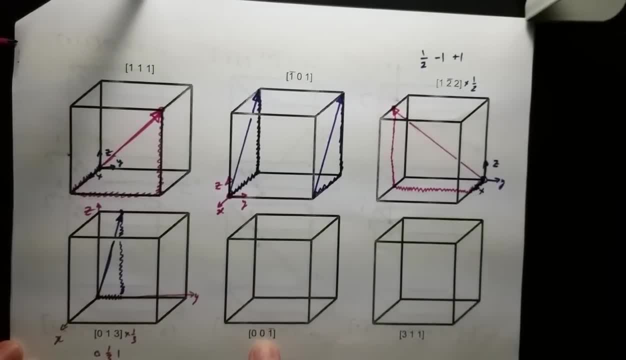 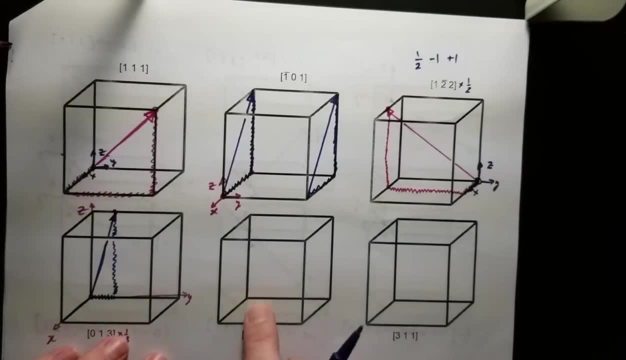 Let's look at the 0, 0, 1 bar. Okay, so in the x and the y we're not going to go anywhere, so we'll just keep ourselves in that back, But we're going in the minus z direction. 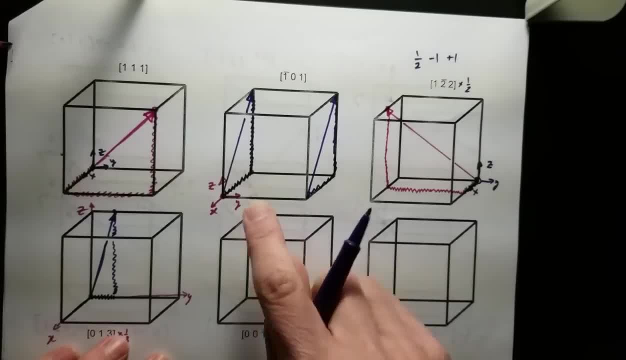 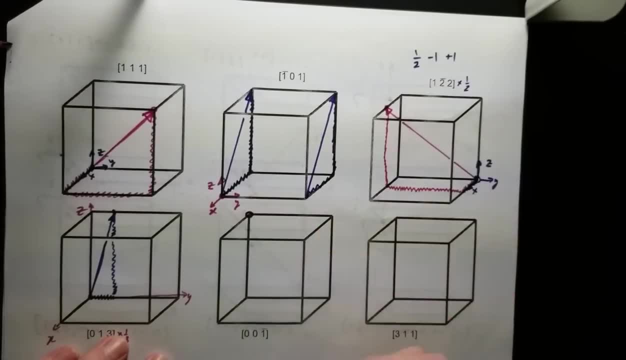 So that means that it's going to be a lot easier if we work from that top plane. So let's pick that as our tail, and then the direction we're going is 0, x, so x, y, z. Okay. 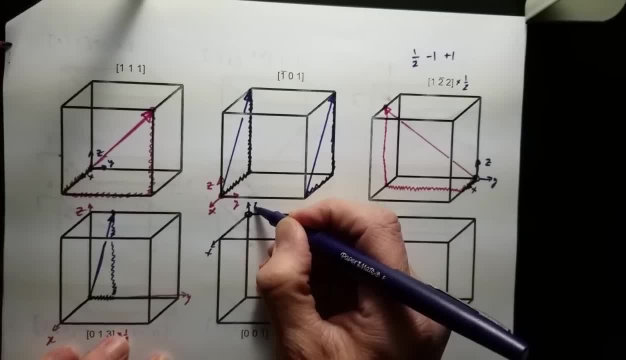 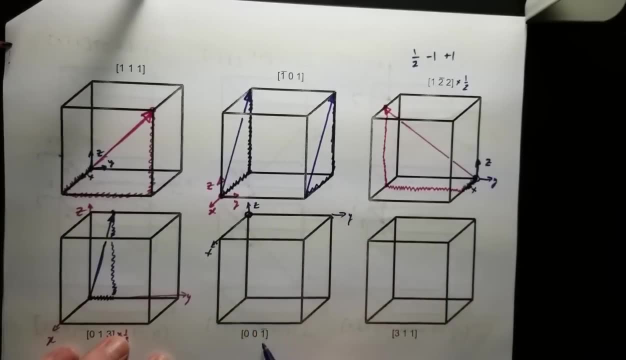 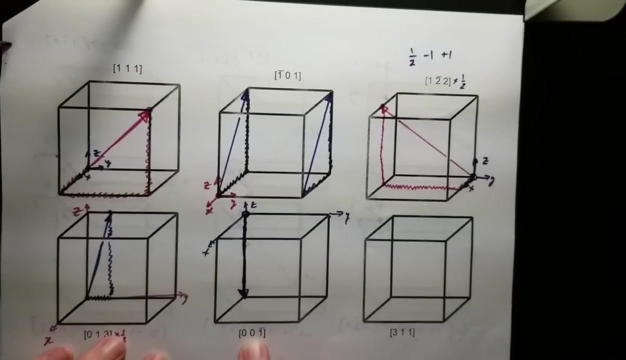 That's it Okay. So we've got z: 0 in the x direction, 0 in the y direction and 1, minus 1, in the z direction. It's going to be down here. So that is our 0, 0, 1 bar direction. 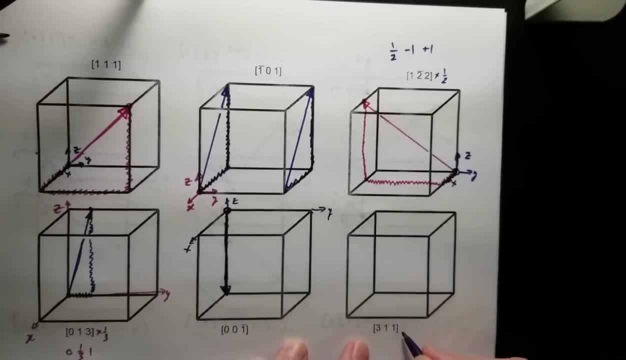 And the last direction: 3,, 1,, 1.. Get rid of the 3 by multiplying by 1.. One third To get 1, 1 third, one third. Pick the back corner as our origin. X, y, z. 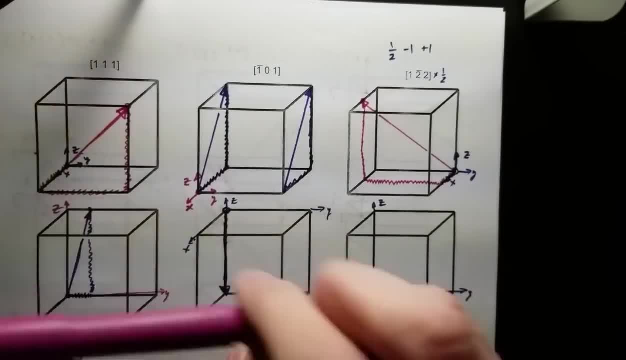 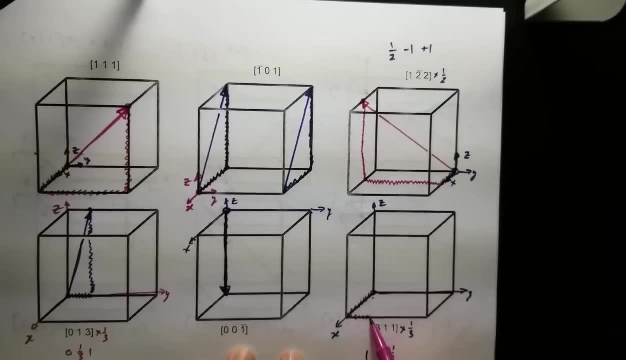 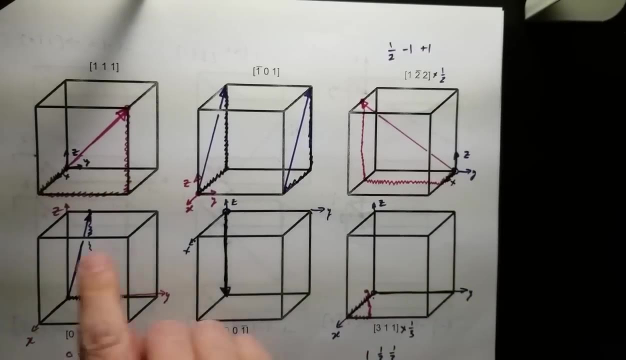 So we go 1 in the x direction, One third in the y And one third in the z Right. Push, Push, Push, Push, Push, Push, Push. It's kind of tough to see the way the angle is, but it's basically going from this back. 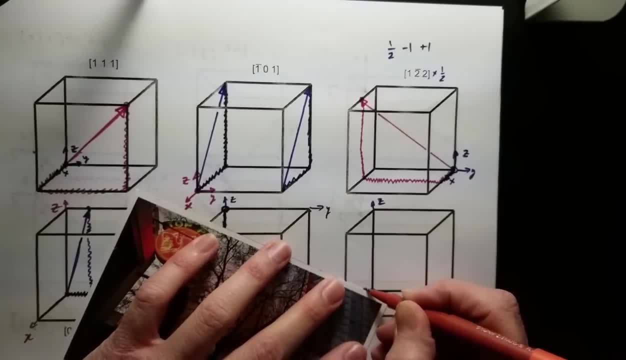 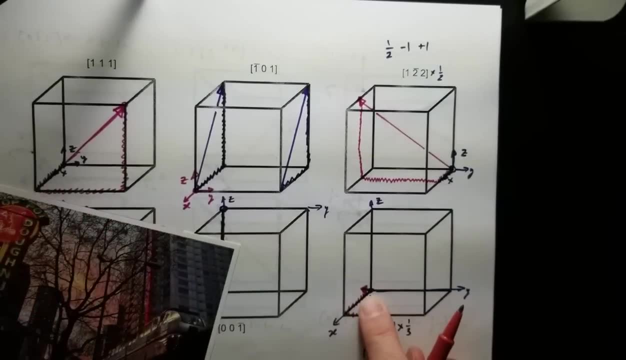 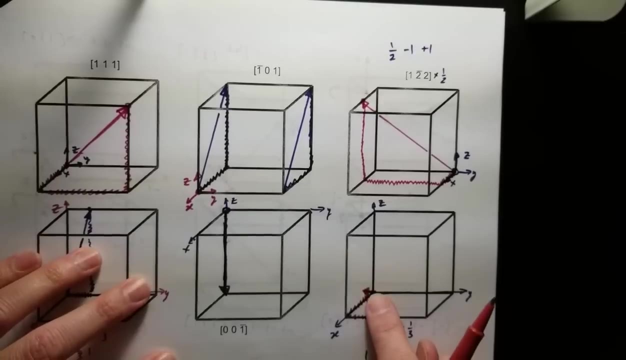 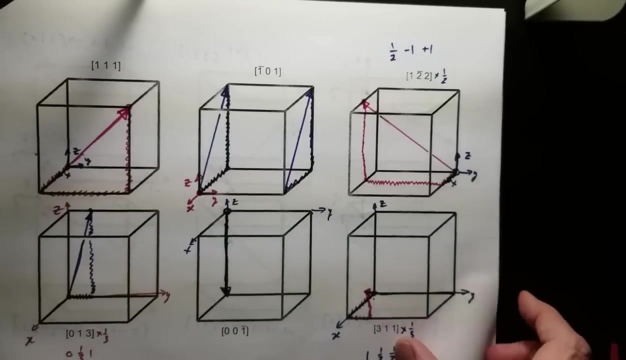 corner to the front face like that. Again, it's not a very clear picture just because of the angle, but hopefully you can see from the trace that we go one, one-third, one-third. So that is how we deal with Miller index directions. 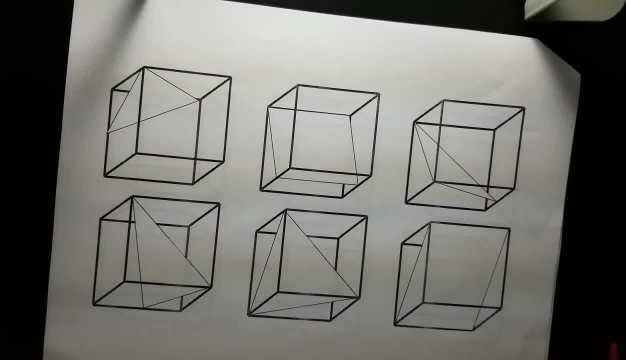 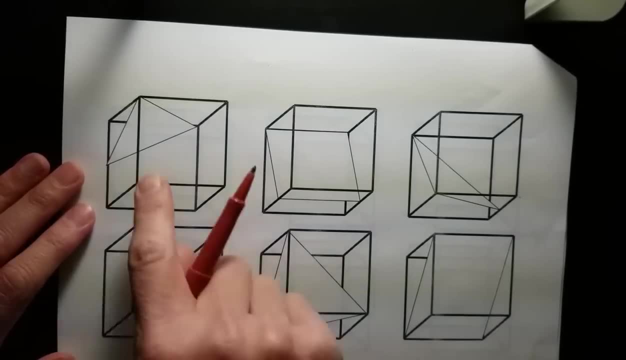 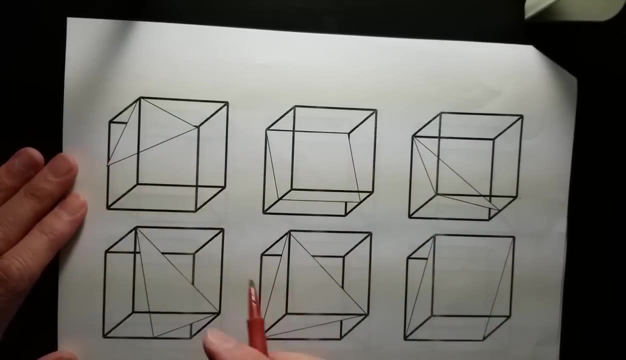 Let's now look at planes. So these planes: when I made them in PowerPoint, I had these lines drawn in, but apparently, converting them to PDF, we lost some of that resolution. So I'll try to draw them in, but you'll have to use some of that. 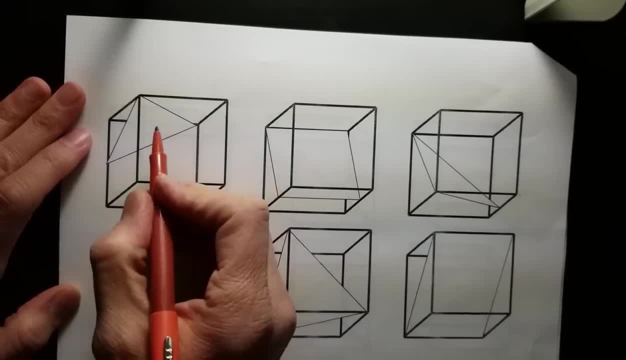 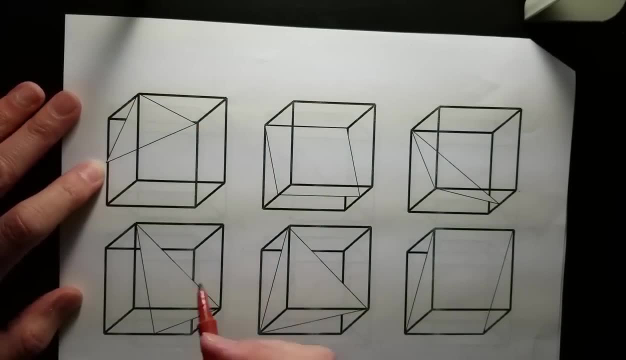 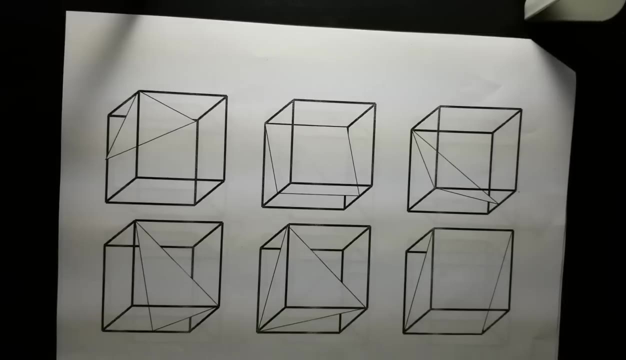 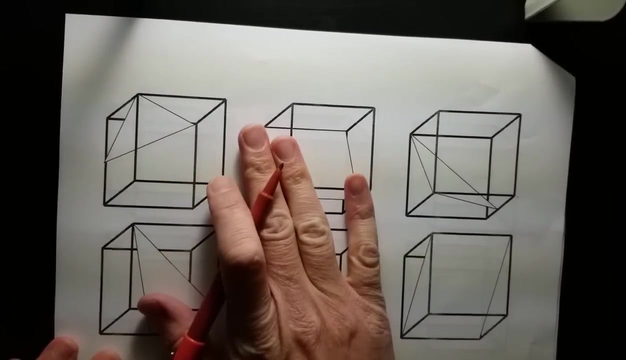 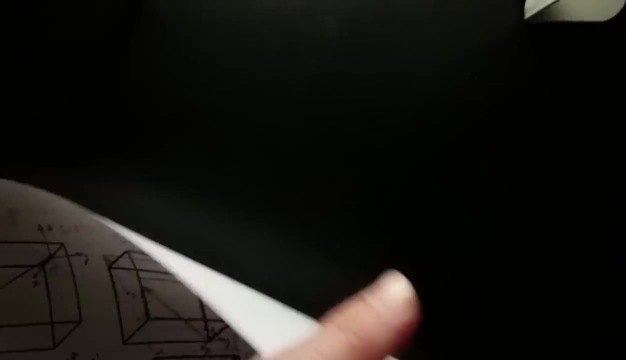 You can use some of your engineering visualization skills to realize where they are, but you can see where they cut the box fairly easily. I think before we do this, let's do the exercise where we identify, We draw the planes. I think that might be easier to follow. 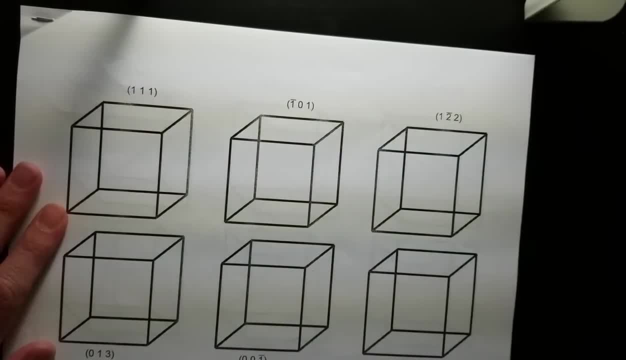 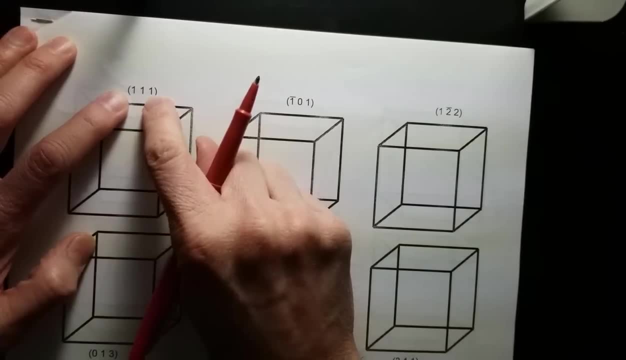 So we'll do this first. Okay, so here I've given you the planes and we'll draw them in the box. So first one is one, one one. So in order to figure out where it intercepts the axis, we have to take the inverse of that. 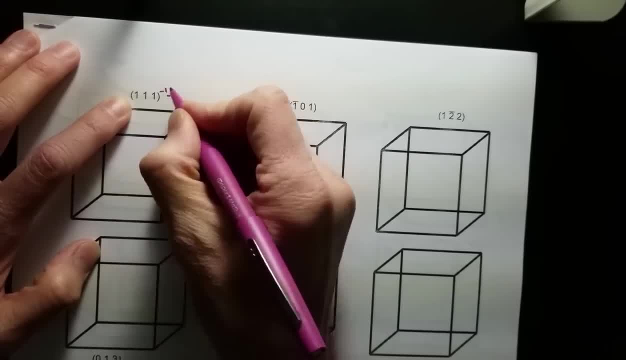 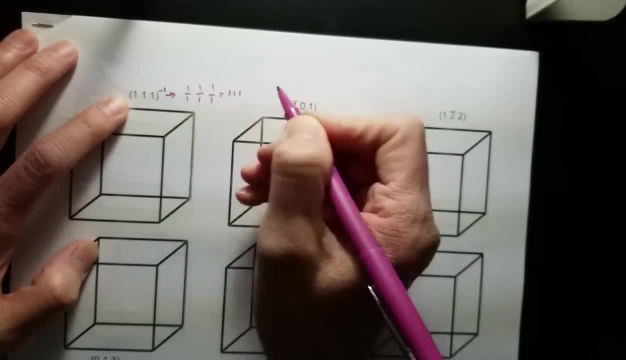 So you raise that to the minus one, which means that we have one over one, one over one, one over one, which is equal to one one one. So it intercepts the x at one, the y at one and the z at one. 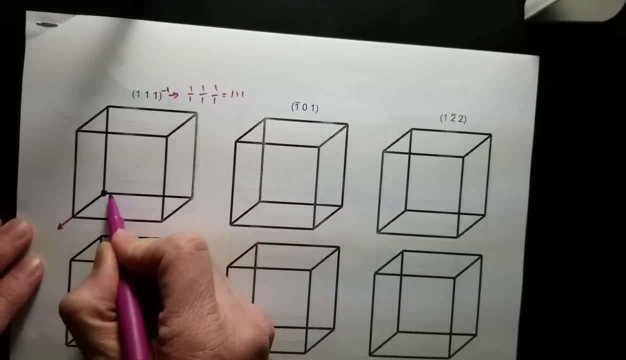 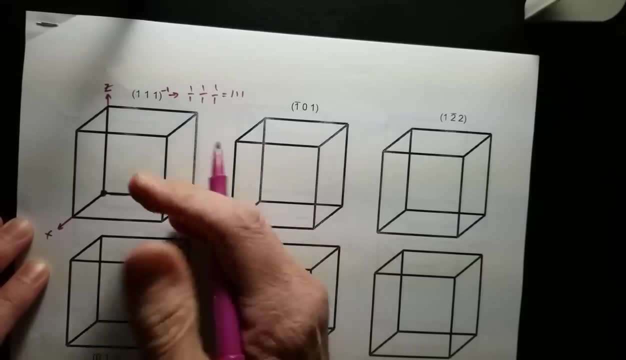 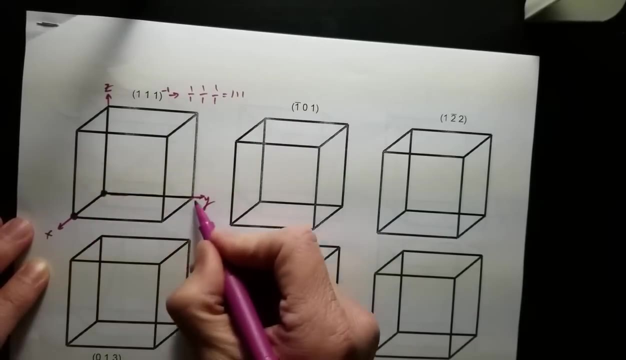 We pick that as our origin. z, so x, y. z got a right-handed axis. It intercepts the x at one. It intercepts the y at one. It intercepts the y at one. It intercepts the y at one. 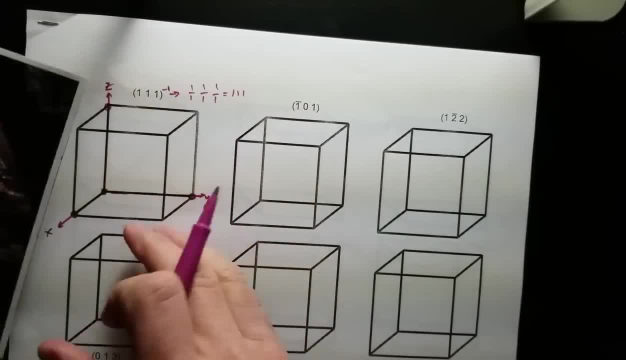 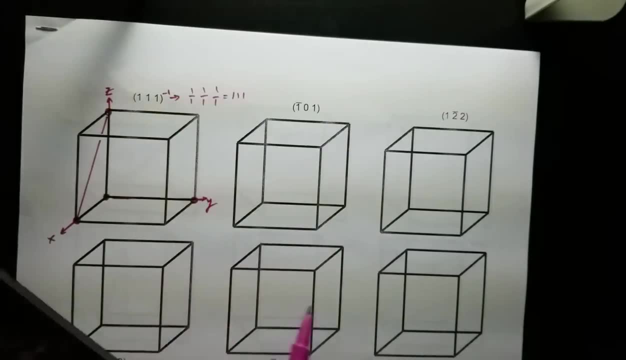 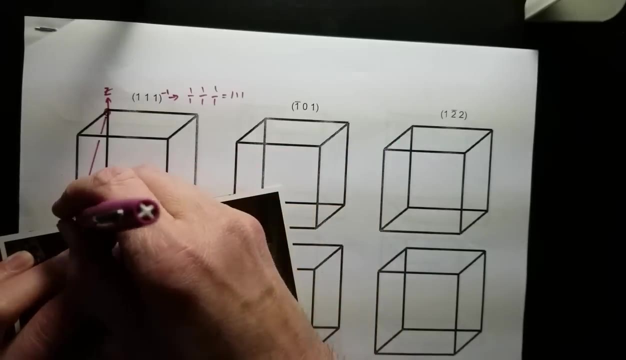 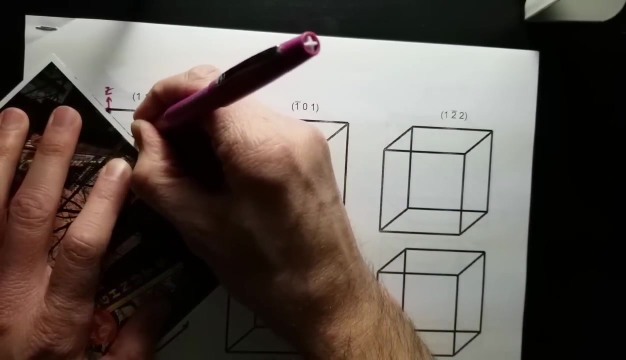 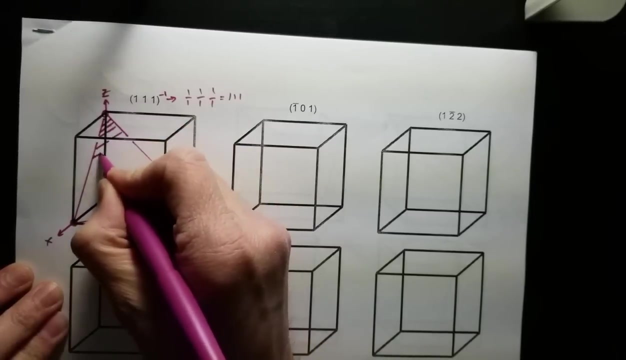 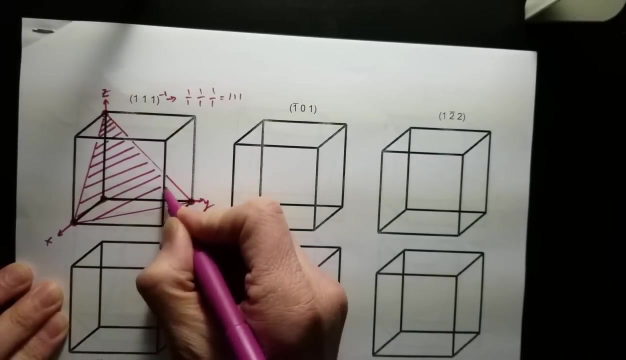 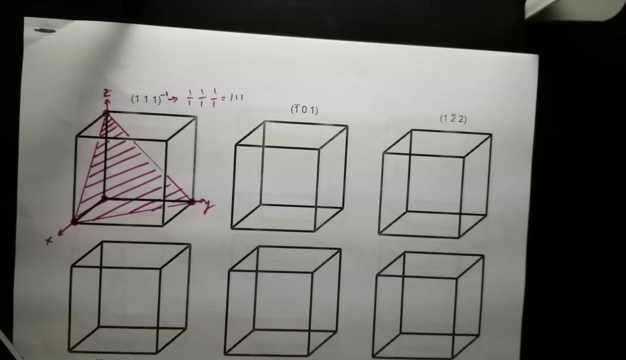 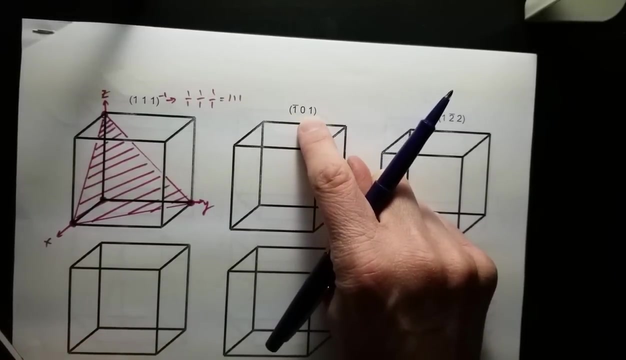 And it intercepts the z at one. So let's draw our plane now. Have some more time. There we go, We trigon, Hey. So this is the plane. Let's try the next one. So this is 1 bar 0, 1.. 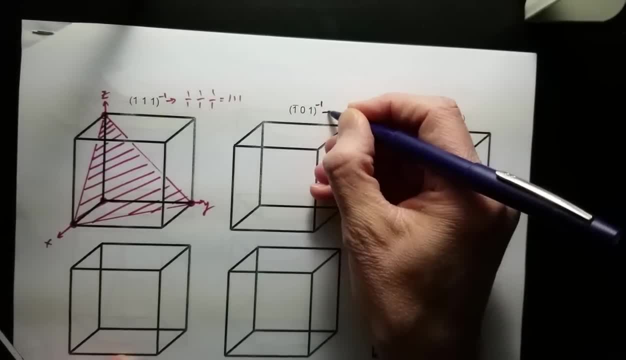 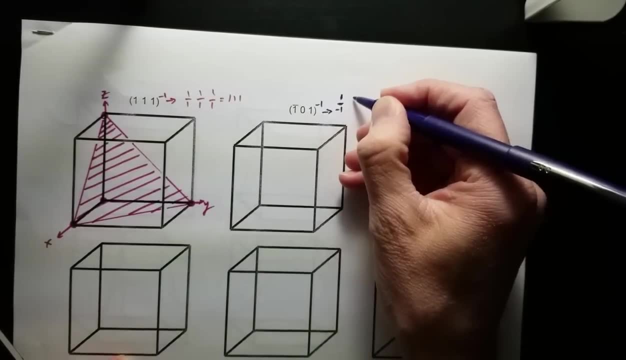 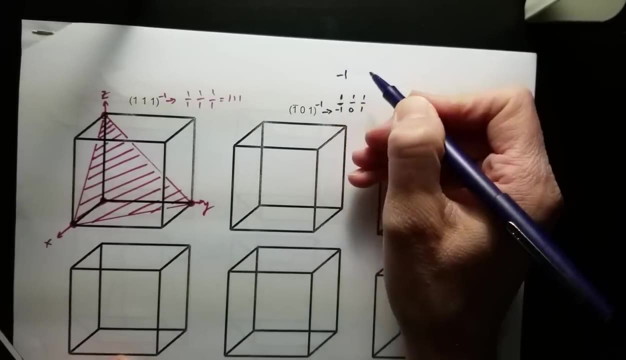 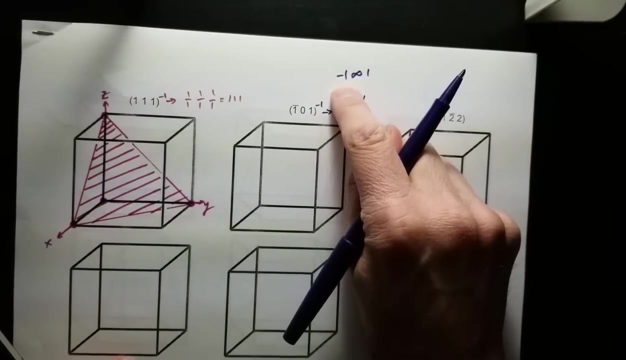 We take the inverse of that, That gives us 1 over minus 1.. 1 over 0, and 1 over 1.. So that is minus 1, infinity 1.. So it intercepts the x-axis at minus 1,. 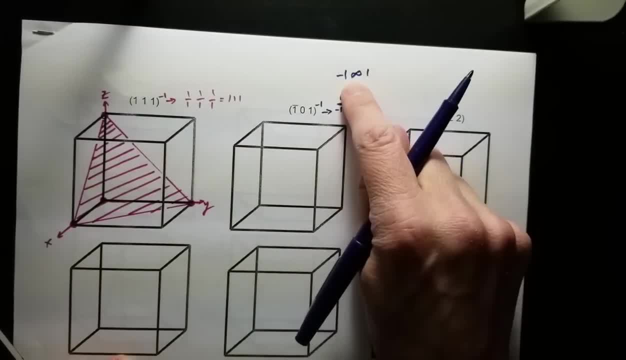 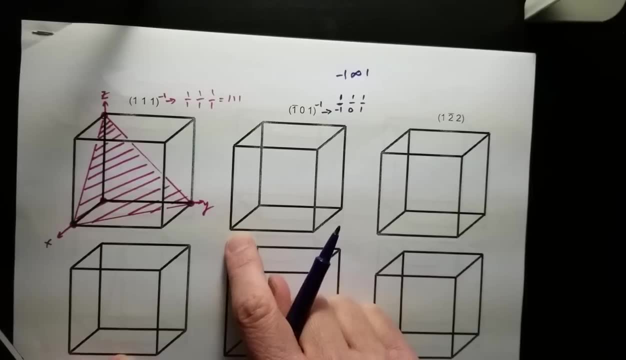 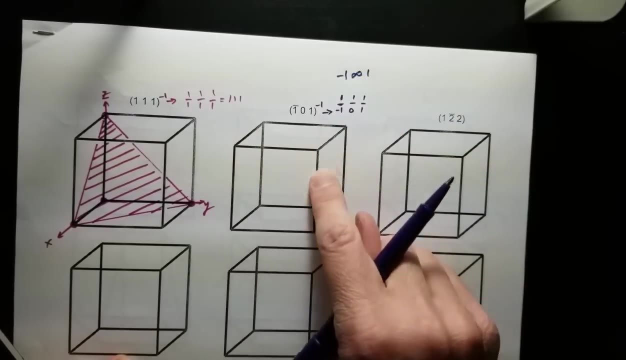 the y-axis at infinity. so it's parallel to the y-axis and it intercepts the z-axis at plus 1.. So we can pick our origin anywhere, because we need an intercept at minus 1x. That means it's going to be most convenient. 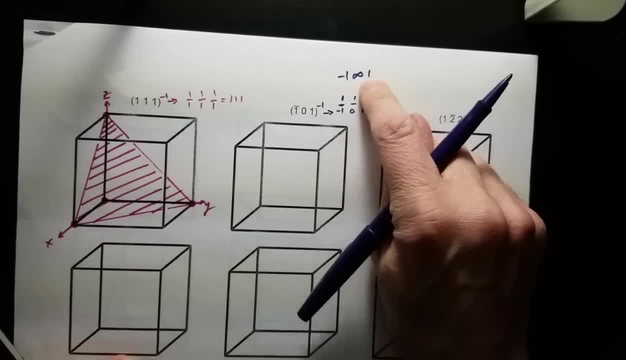 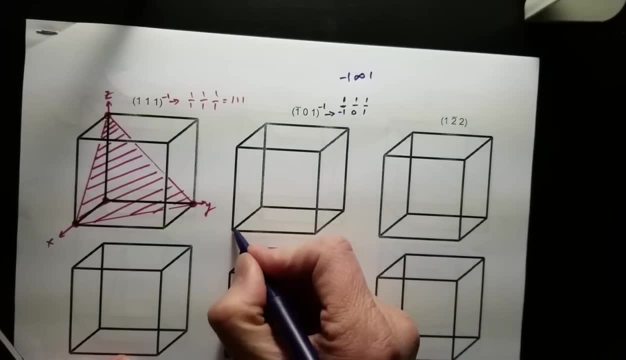 to pick something on the front here, And it intercepts z at the plus 1, so that means it's more convenient to pick something on the bottom. So let's pick this point Right. here is our origin, Z, So it intercepts x at minus 1,. so right there. 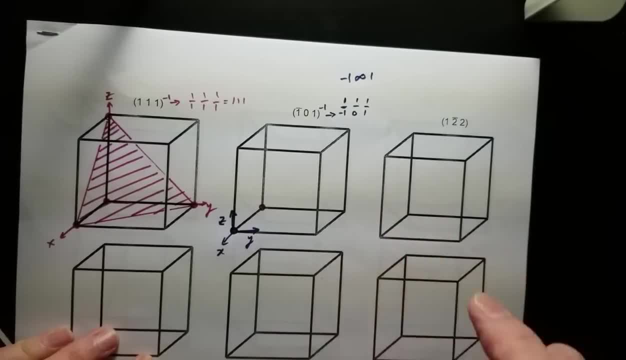 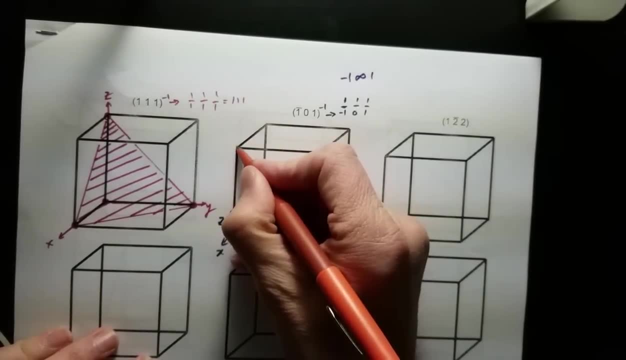 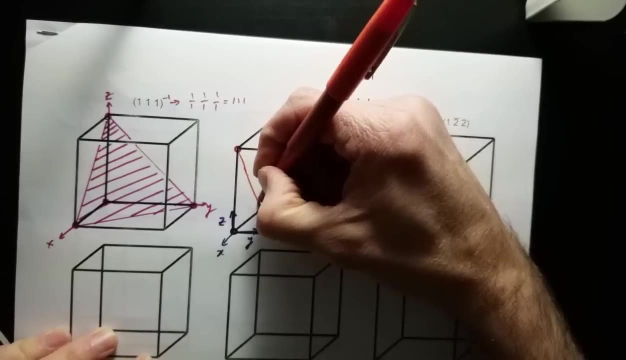 It intercepts y at infinity, so I can't draw that anywhere- And it intercepts z at plus 1.. So that's the intercept. So if I've got some plane where that's part of my plane and it goes all the way out to infinity, 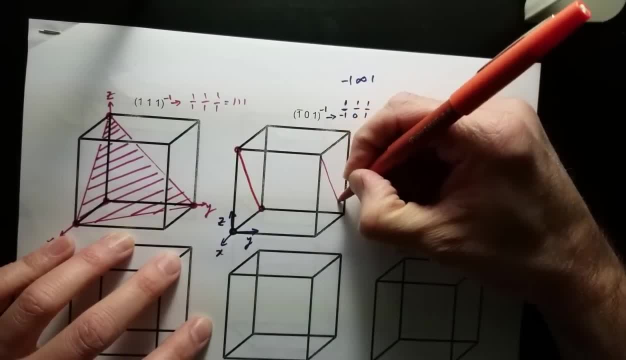 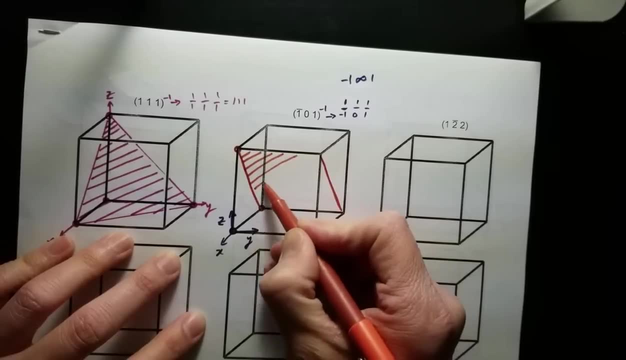 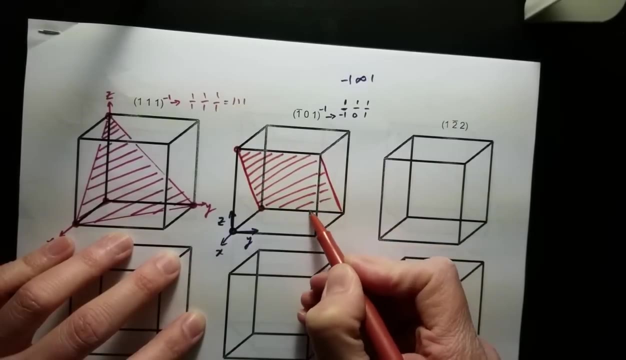 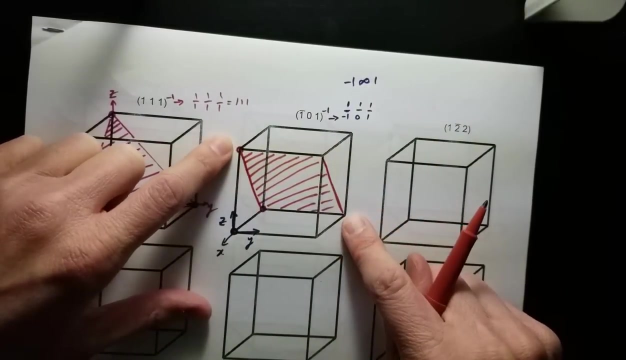 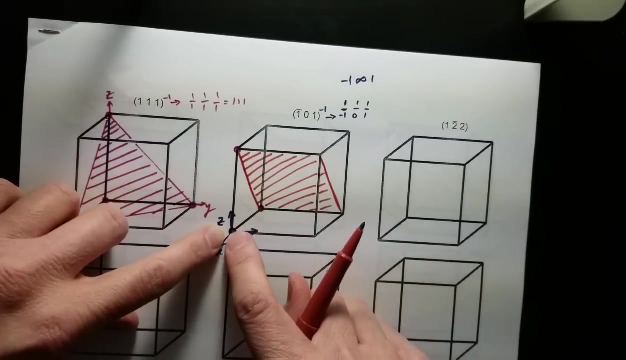 well, that means that my plane is actually defined by this. Can you see that This plane, which cuts through kind of this diagonal of the box, it runs parallel to the y-axis, so it never cuts the y-axis and it cuts the x-axis here. 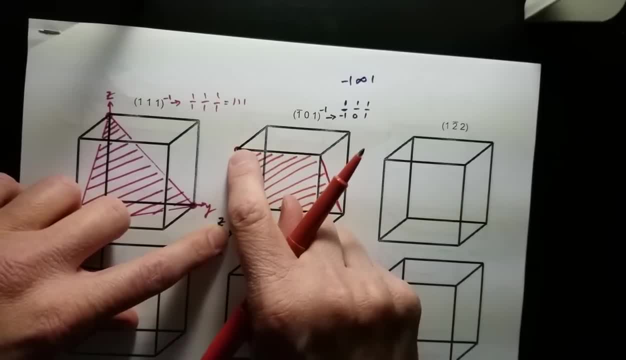 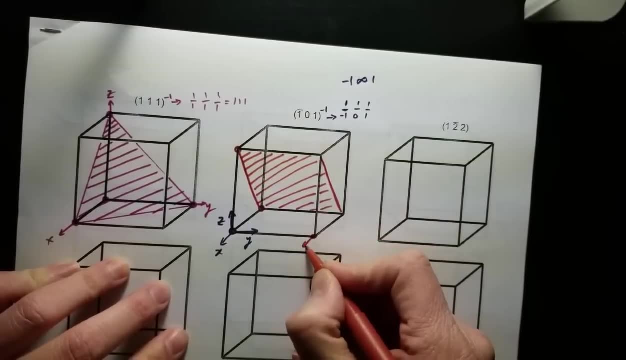 and the z-axis here, so minus 1 and plus 1.. If I'd picked my origin to be here instead, I could have done the same thing right, Because I could have had this be x, z, y. So regardless of whether I picked here or here as my origin, 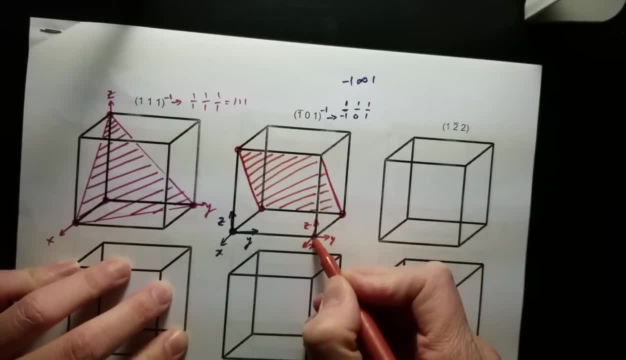 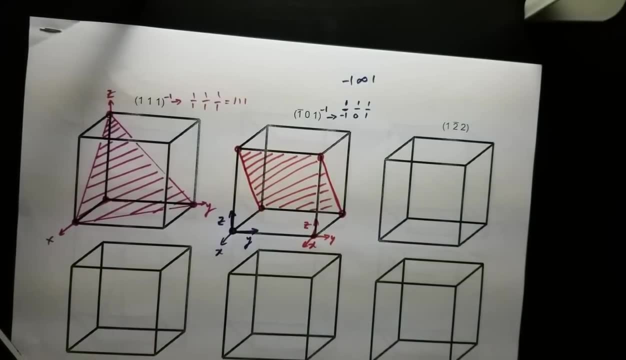 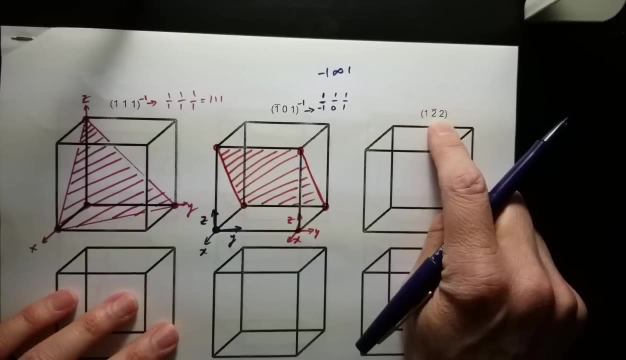 I would still have an intercept at minus 1 and plus 1.. This is the z-axis. The y-axis is minus 1 and minus 1 and minus 1, and this here and the z-axis crossed out is just 1 and then 2.. 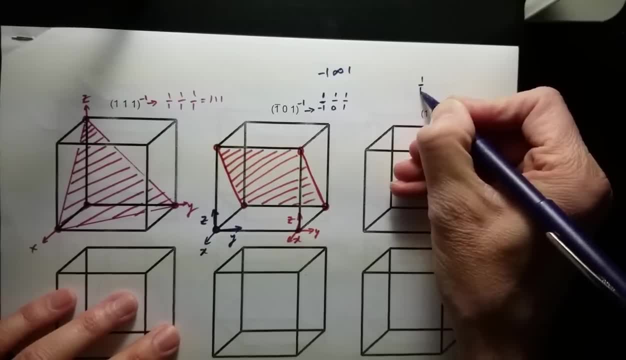 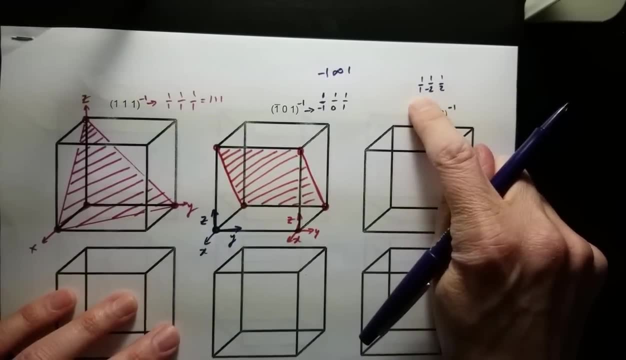 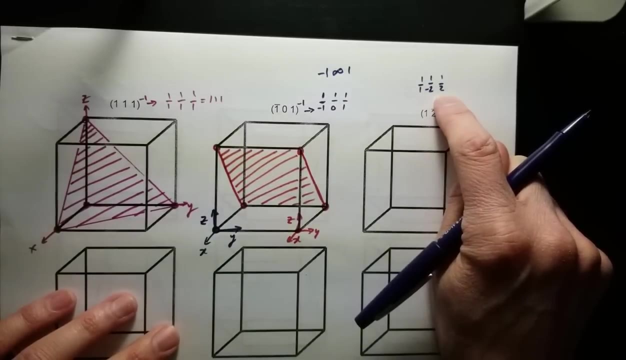 Now what I have is the x-axis will be a 2, and the z-axis will be a y-axis, and therefore the z-axis will be an y-axis, But the y-axis is just a y-axis and the z-axis is just a y-axis, and the z-axis is 1 and minus 1.. 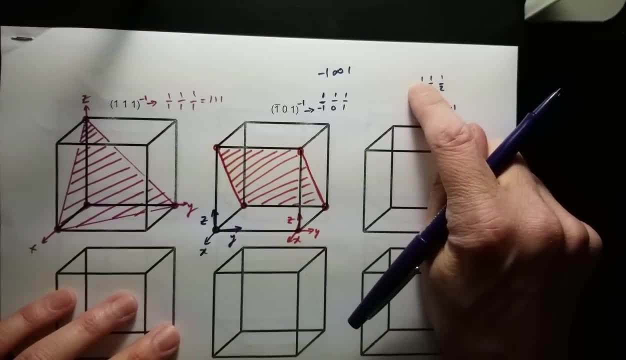 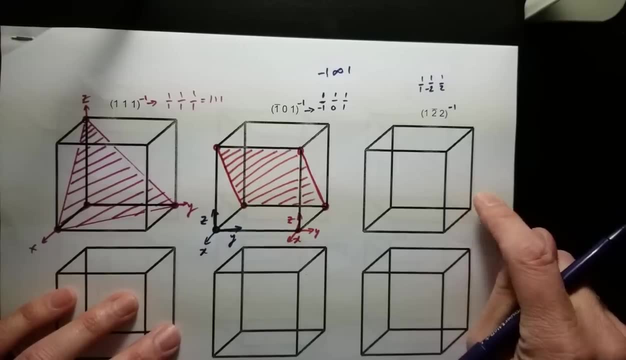 at plus one half. so the fact that we've got a plus positive x intercept means back plane makes the most sense, the fact that we've got a plus z intercept means the bottom plane makes the most sense, and the fact that we have a negative y intercept means the right makes the most sense. 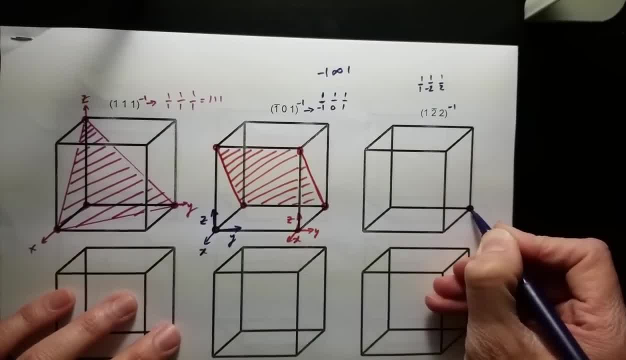 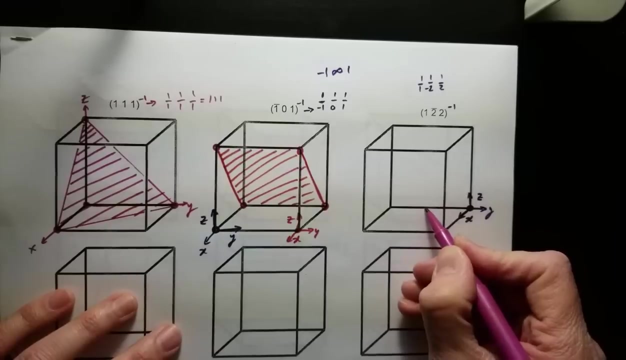 therefore i'm going to pick my origin here: x, y, z. so i have an x intercept at plus one here, i have a y intercept at minus one half, which looks like about right here, and i have a z intercept of plus one half. it's about right there. 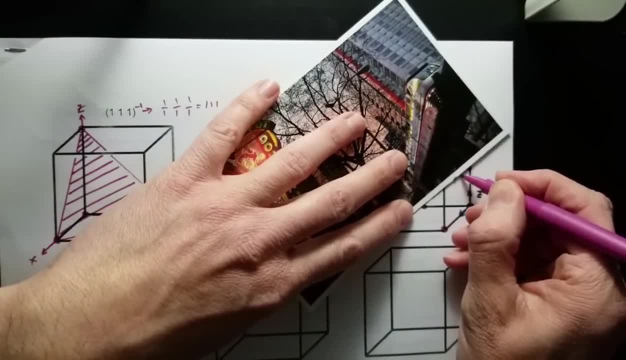 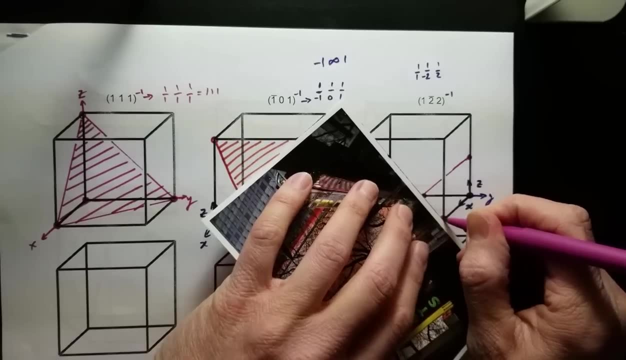 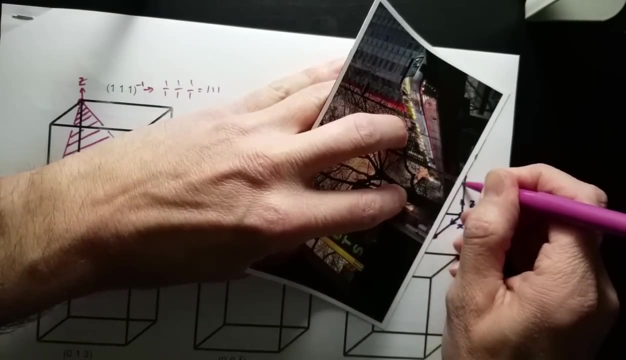 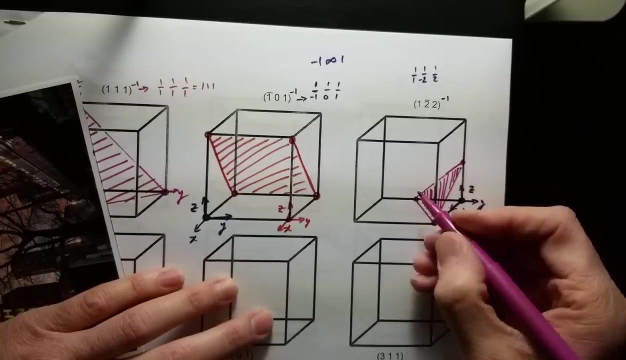 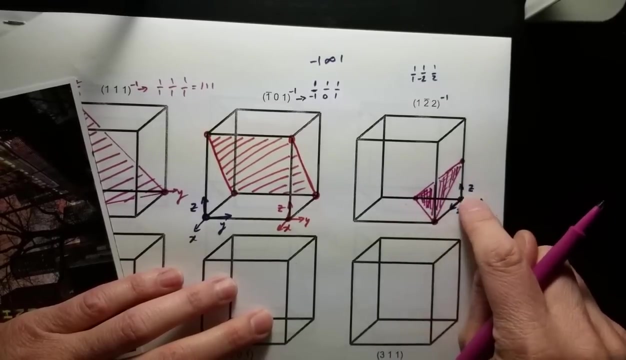 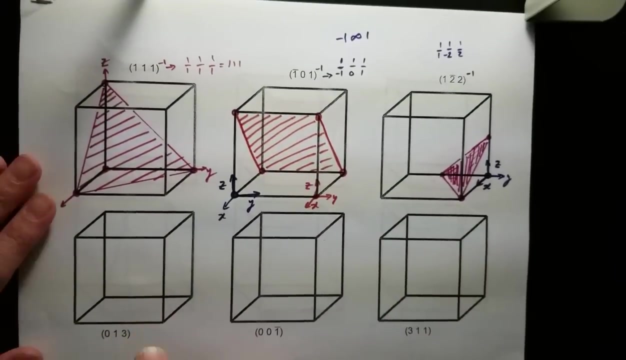 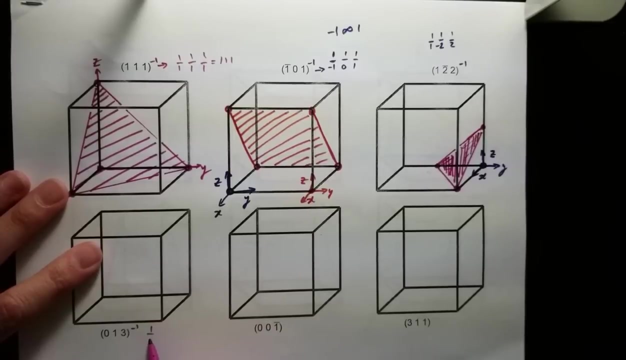 so my plane is there. so that's my plane: one minus one half plus one half. okay, the third one, take the inverse. or sorry, the fourth one, take the inverse. that gives us one over zero, one over one, one over one third, which is infinity one one third. so now we know. 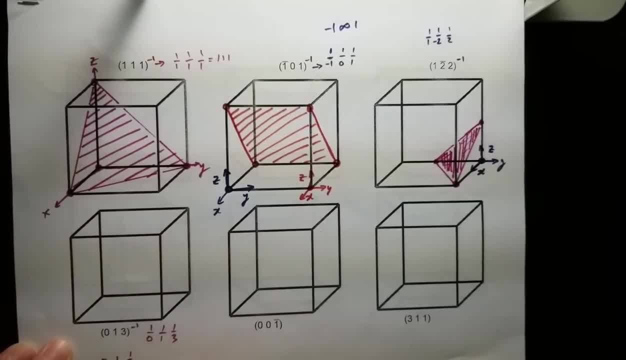 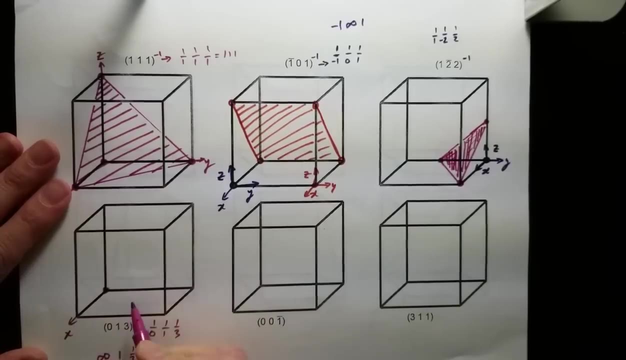 that the x-axis is going to cross at infinity, the y-axis is going to cross at plus one and the z-axis at plus one-third. so that means going to the back left a corner. that's a good place for us to make our origin: x- y. 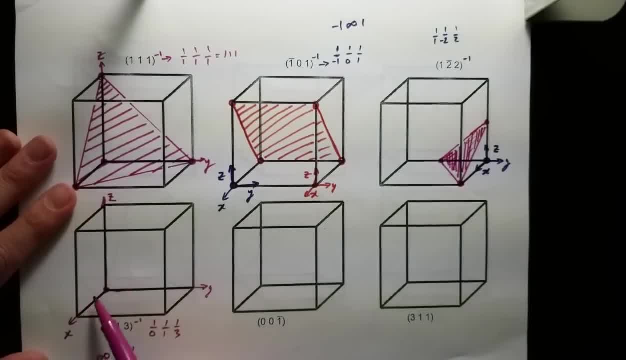 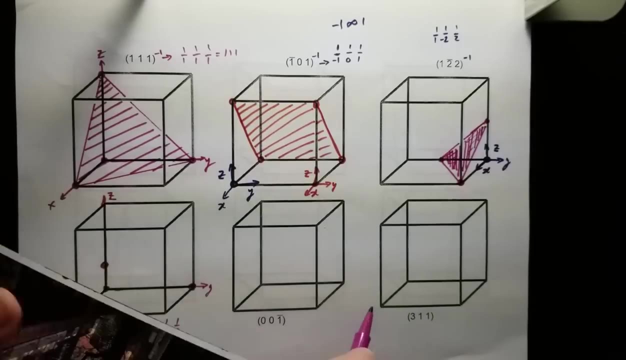 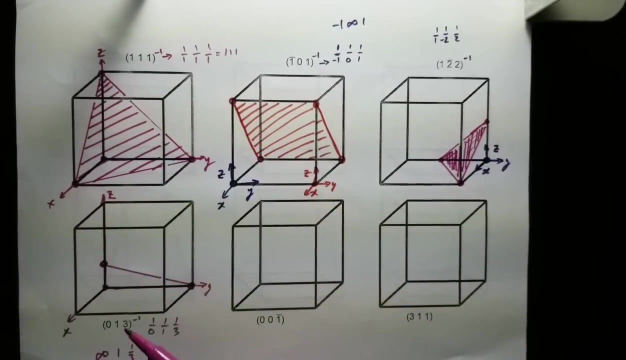 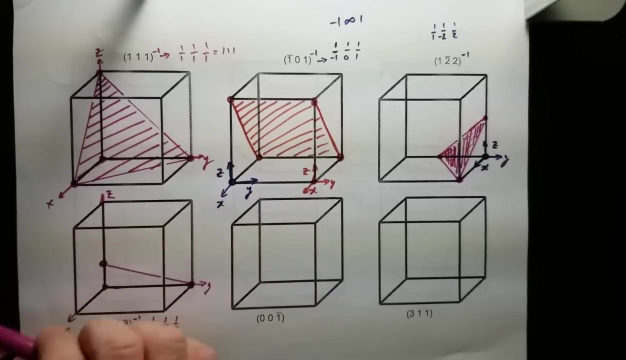 z, x crossed at infinity, so we can't draw it. y crosses at 1, that's right there, and Z crosses at 1, 3rd, which is about right here. So we have this line as part of our plane And because This plane is going to extend in the Z direction and never- sorry- in the X direction and never cross X, 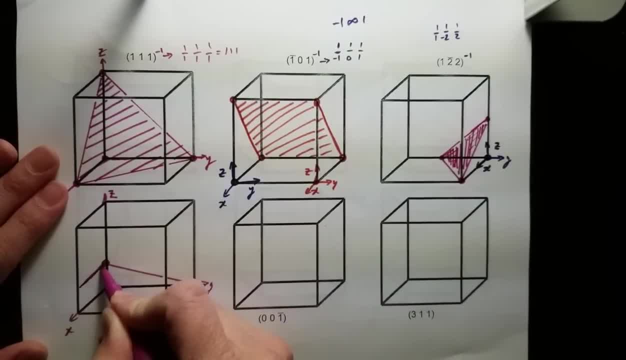 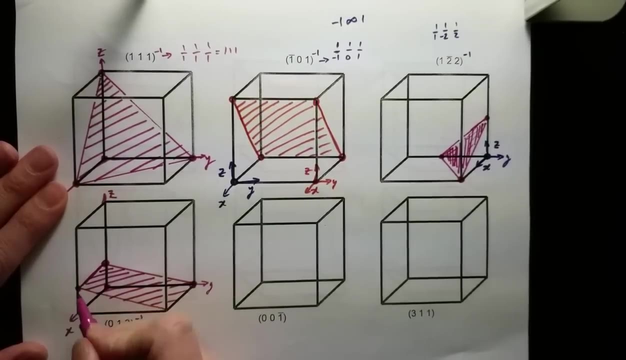 that means that it can go like this, and This is going to be our two plane Like that. And again, if I had picked this front as my origin here, Then I would still have a y-intercept of plus 1 and a Z intercept of plus 1. 3rd, 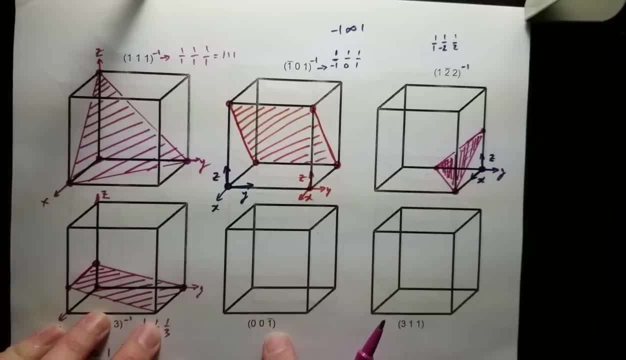 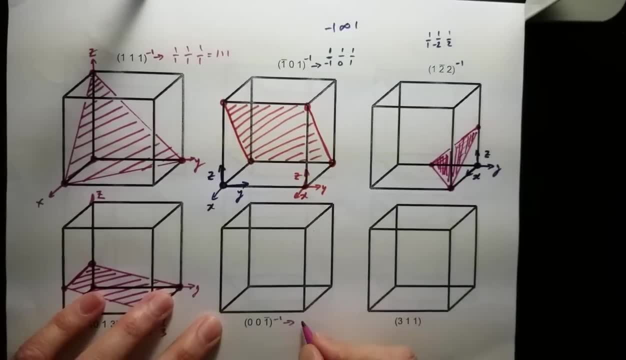 Hey, the fifth problem: zero, zero, one bar. Take the inverse And that gives me an intercept at infinity, infinity Minus one. Okay, Well, I know that I can't say anything about X or Y, except that they never cross, and The Z, we know, crosses down here at minus 1. 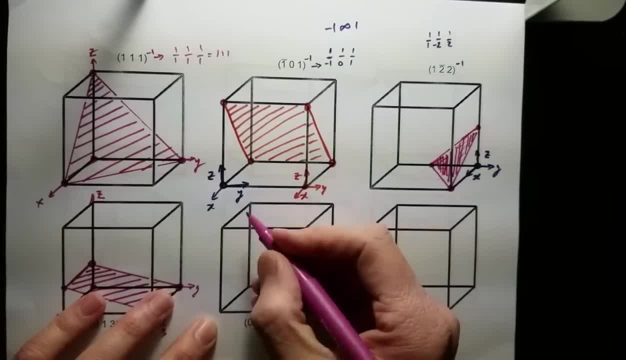 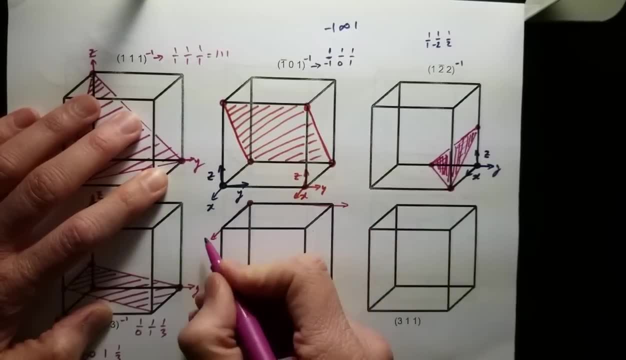 so I'm gonna pick my Origin somewhere on the top, so I'm gonna pick up here in the back left top. So that is X, Y, Z. It never crosses X, never crosses Y and it crosses Z here at minus 1. So the plane that cuts through that point never crosses X and never crosses Y. 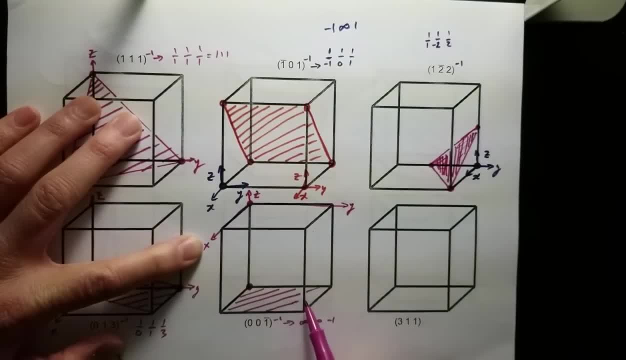 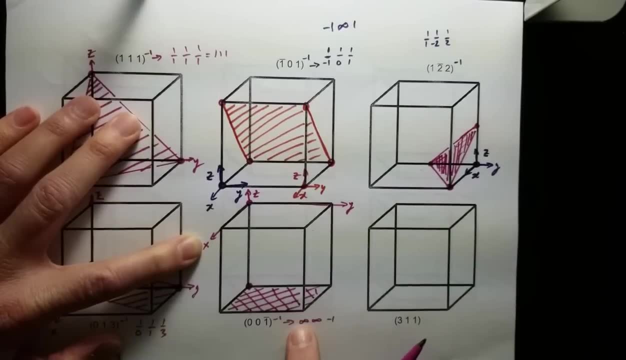 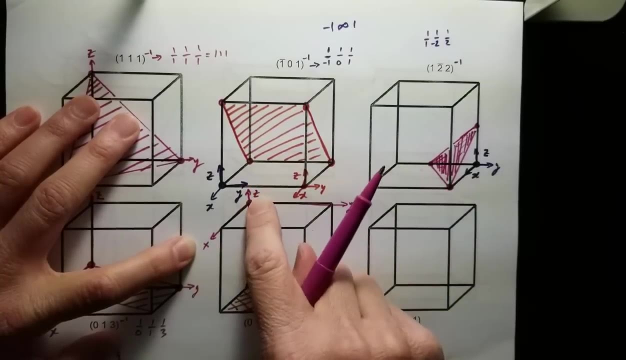 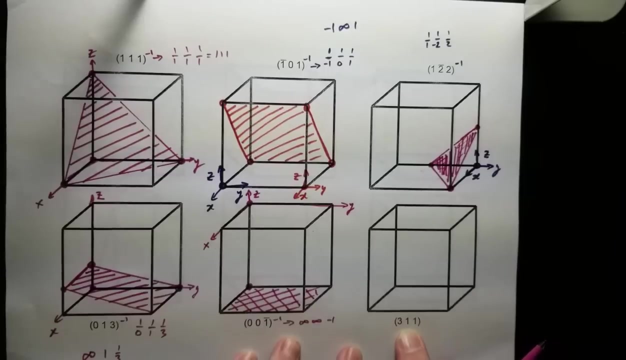 This plane. It's the face of the cube. So this is a, the plane that runs parallel to the XY plane and Crosses Z down here. And lastly, we'll go to 3: 1- 1. Taking the inverse, we get 1. 3rd, 1, 1. 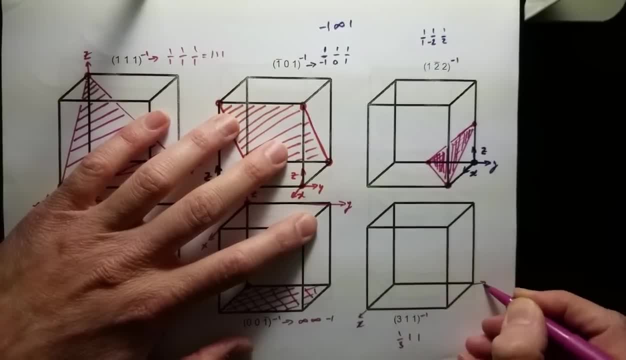 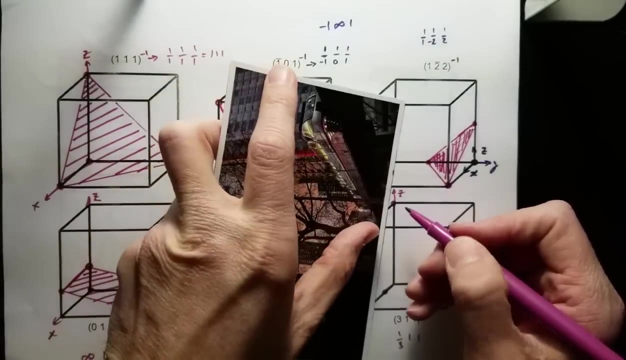 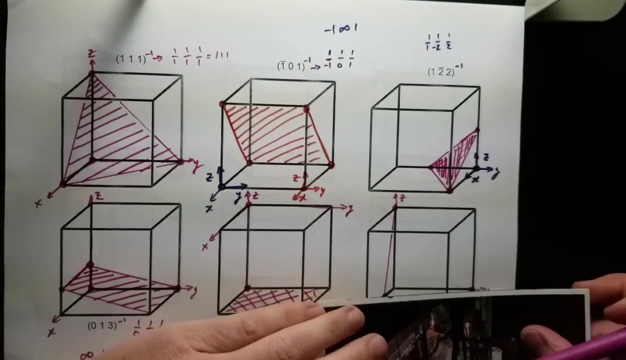 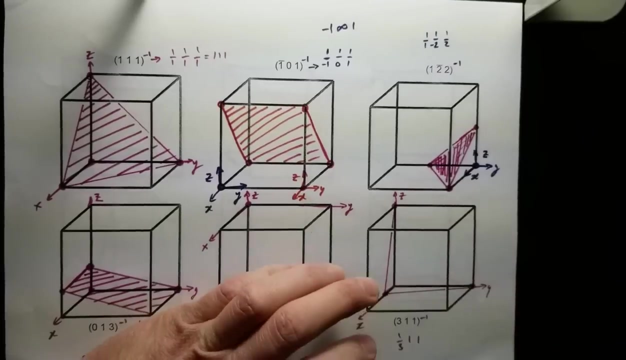 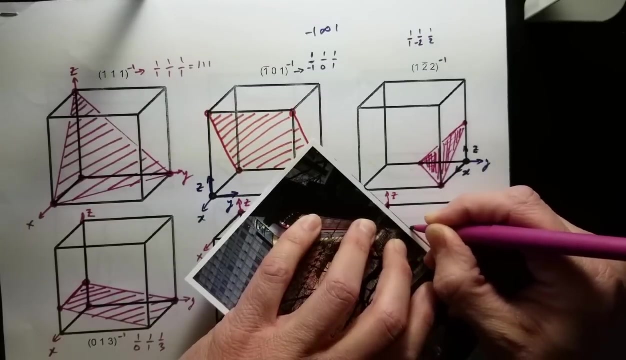 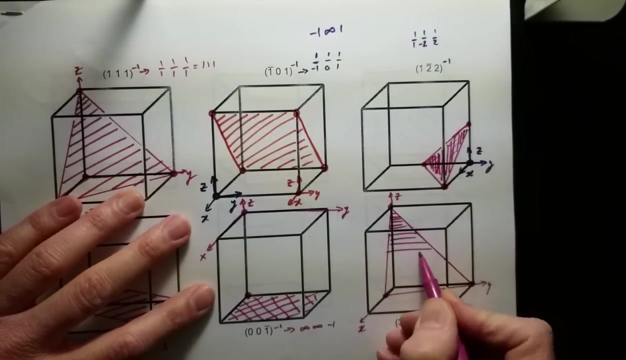 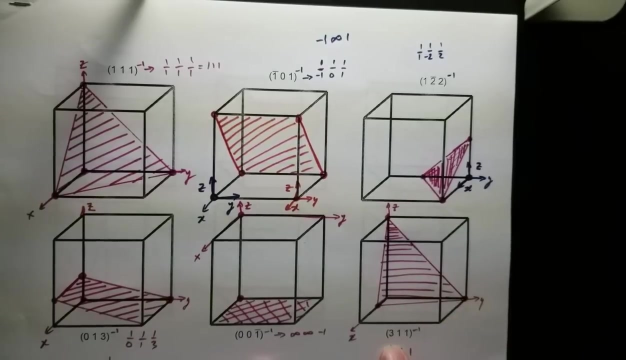 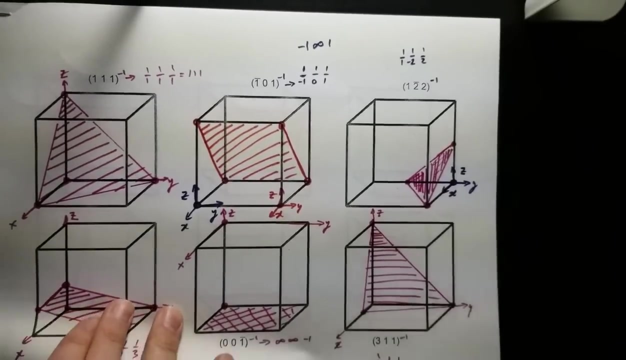 Okay, we'll pick X, Y, Z, Crosses X at 1, 3rd about right there. crosses Y at 1, crosses Z at 1, Drawing our Plane, our makeshift ruler, And this is our 3-1-1 plane. Okay, so now let's go to the last. 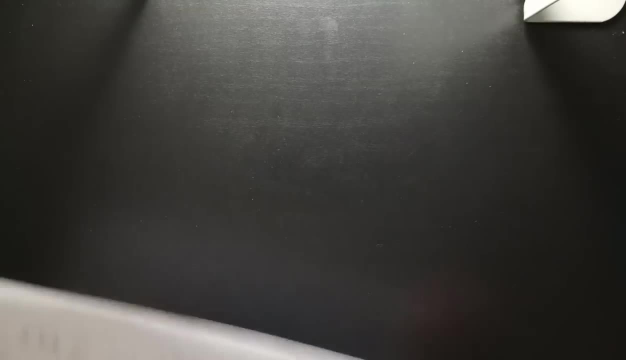 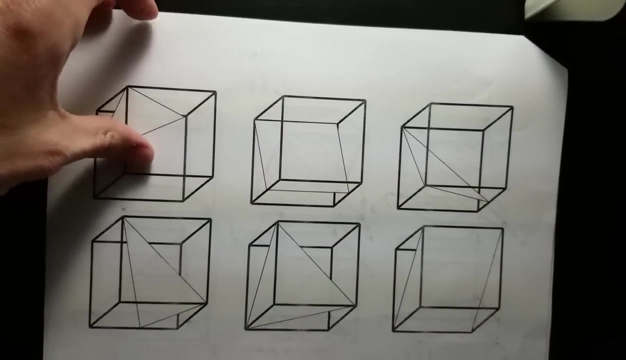 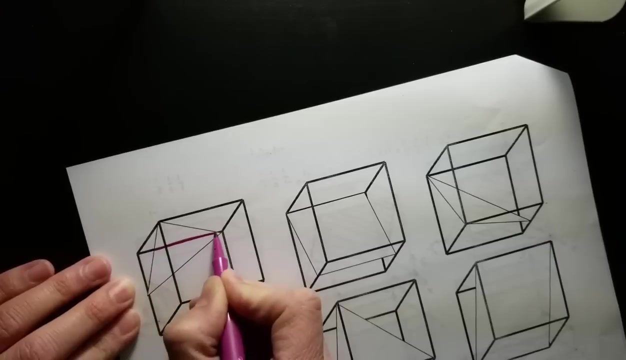 page in which we're going to identify these planes, And that, I think, is a little bit more tricky. I'll show you some of the tricks, though, And, as I said, I'm sorry that the I just cut off some of the images. 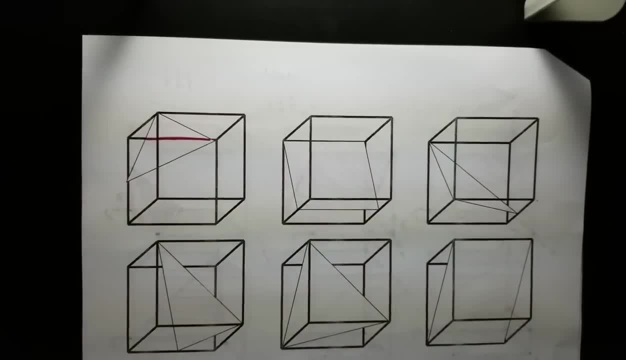 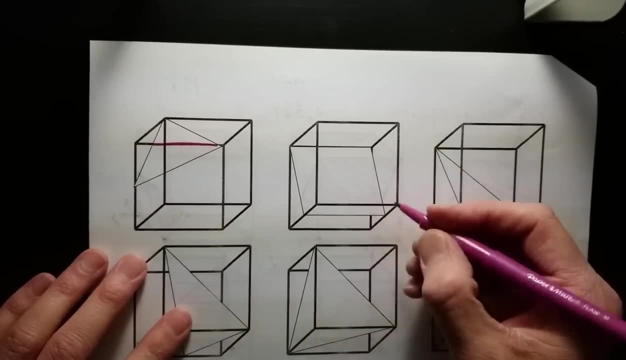 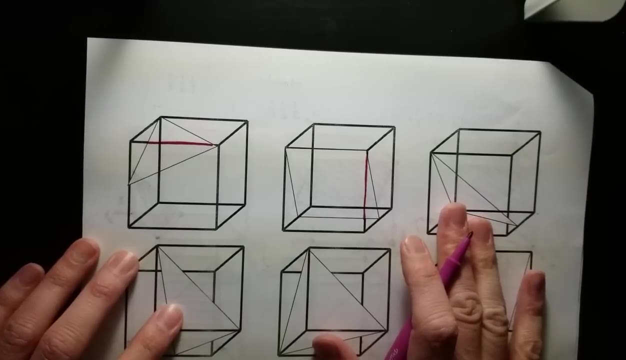 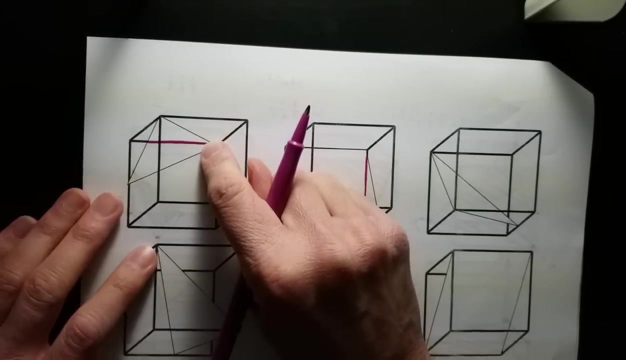 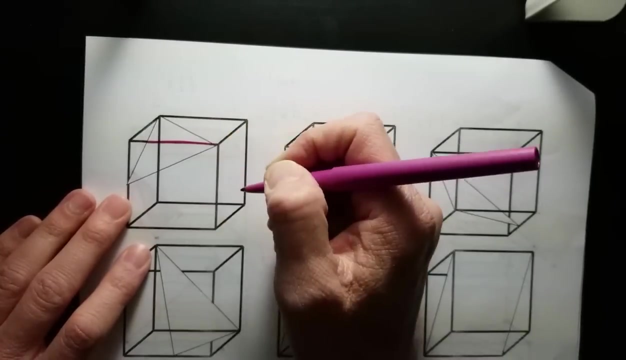 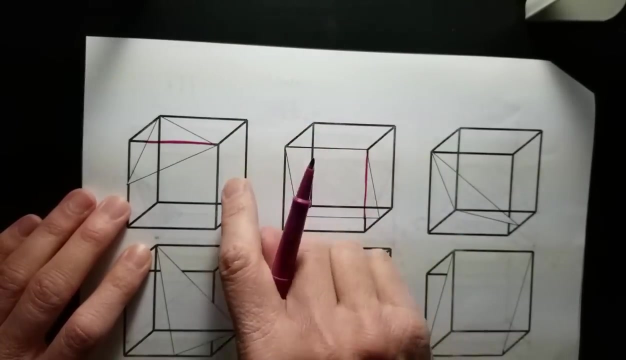 So let's start. So let's start here. Okay, so you've got this plane and we want to look for an origin that allows us to talk about intercepting the axis. And again, you can pick any, but if you pick, you know. 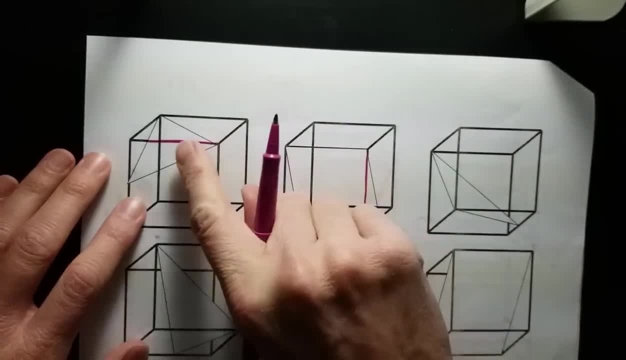 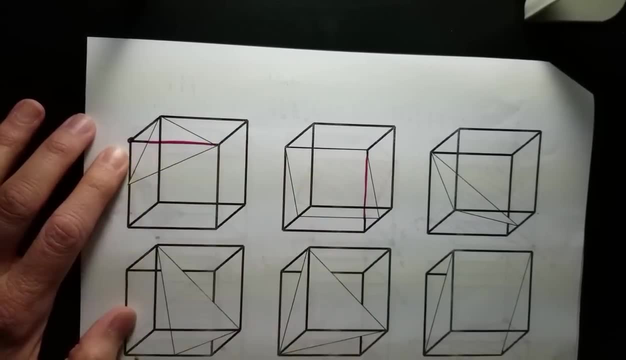 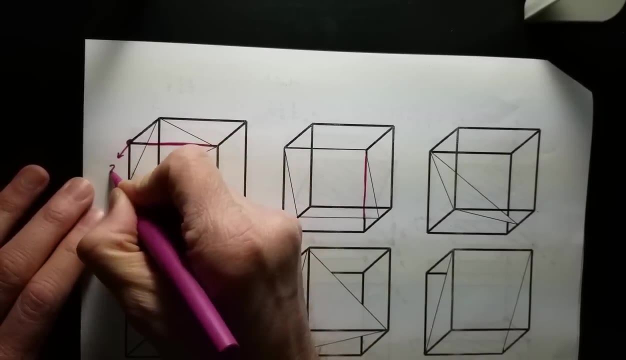 for example, this back right corner, then you're going to have to extend this plane up and imagine where it cuts. Starting here, though, we have natural places where the axes are cut, So we have our x, y, y. 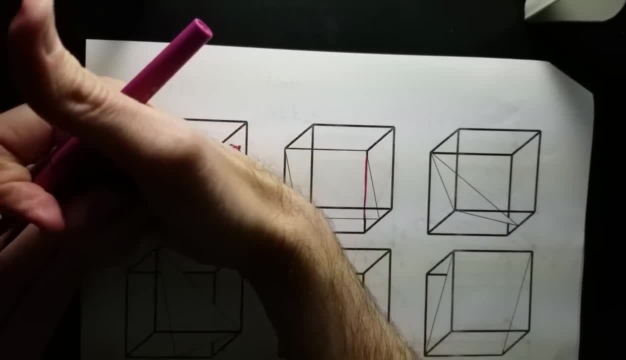 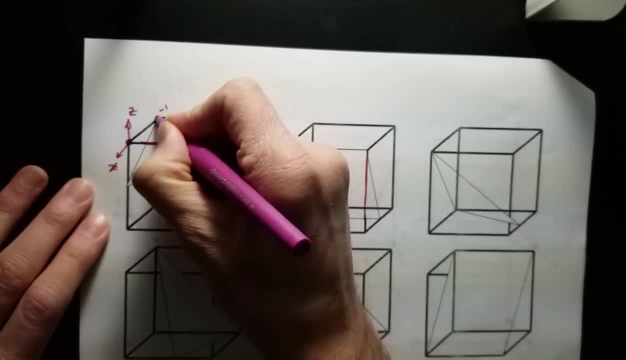 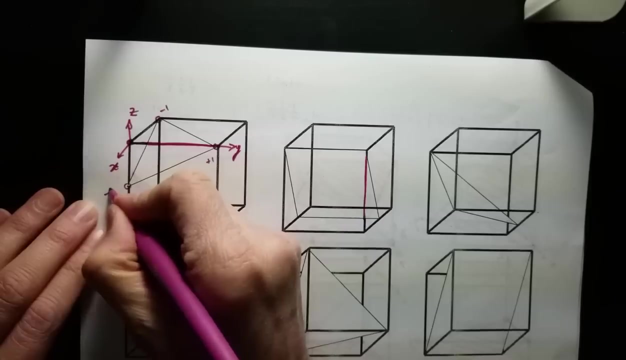 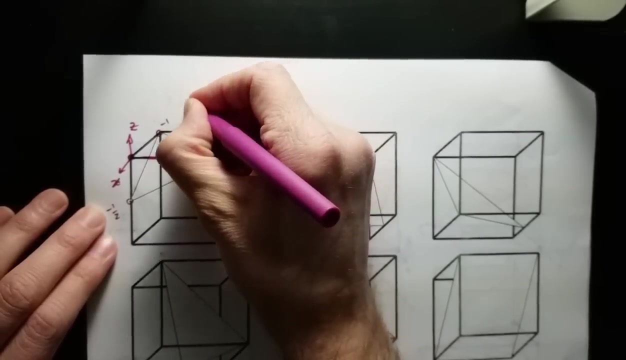 y, z. again, it's a right-handed squared system. it cuts the x-axis at minus one, It cuts the y-axis at plus one and it cuts the z-axis at minus one half. Okay, So that means we have minus one. 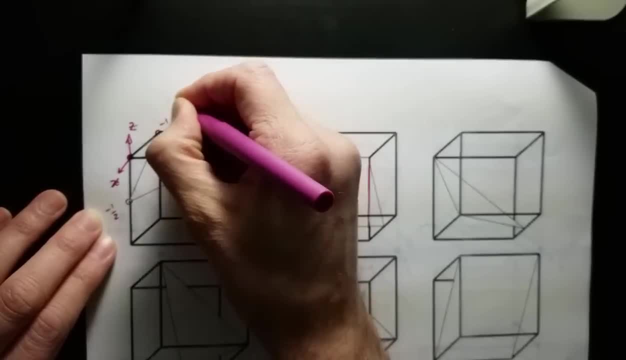 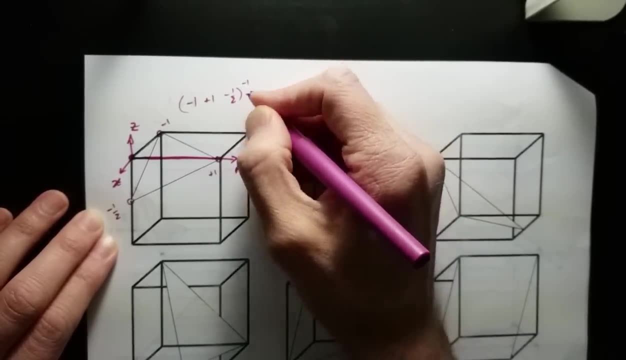 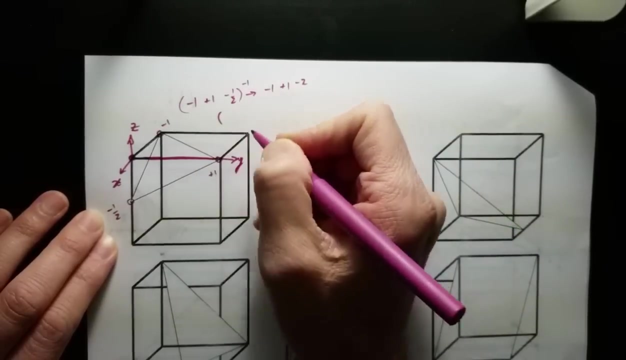 plus one minus one half. We take the inverse of that and that's going to give us minus 1 plus 1 minus 2.. And putting that in the proper notation, that is 1 bar 1, 2 bar. 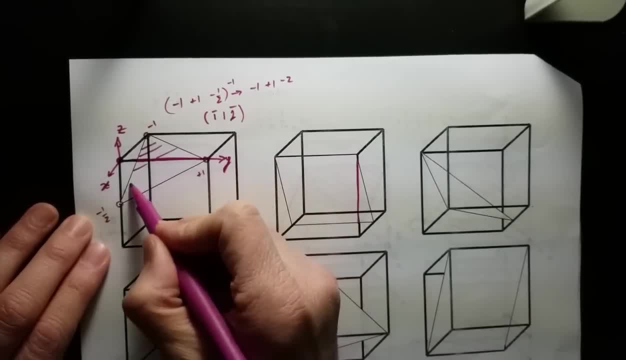 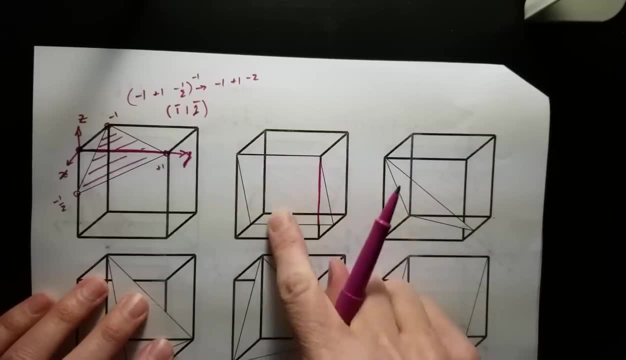 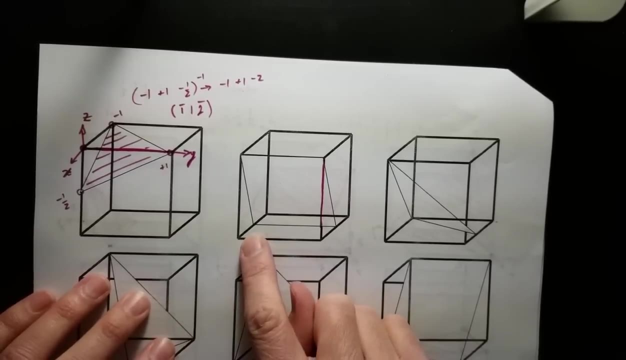 So this plane is the 1 bar, 1, 2 bar plane. Okay, let's do this one next. And again, we want something where we get natural axis being cut, And this one notice that, well, it runs parallel to this axis which is going to be our y-axis. 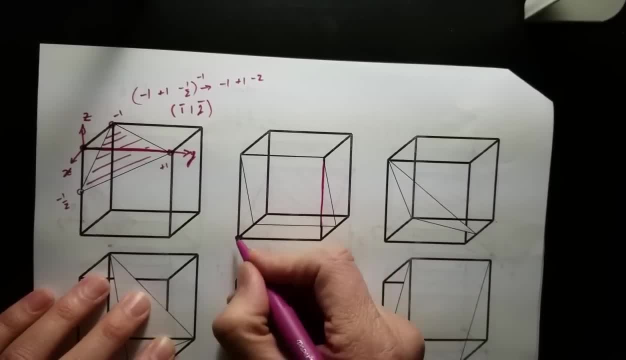 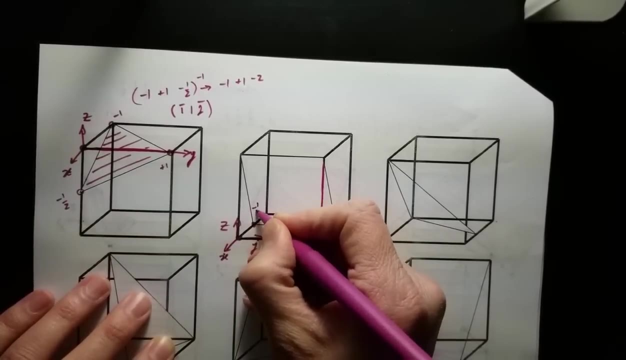 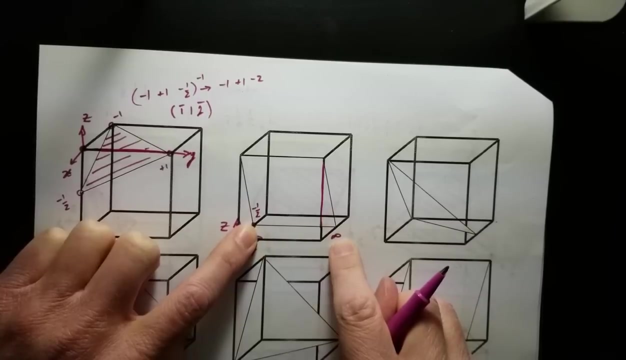 So let's make this front our origin: x, y, z. Okay, It's going to cut the x-axis at minus 1 half, It cuts the y-axis well out at infinity And it cuts the z-axis at plus 1.. 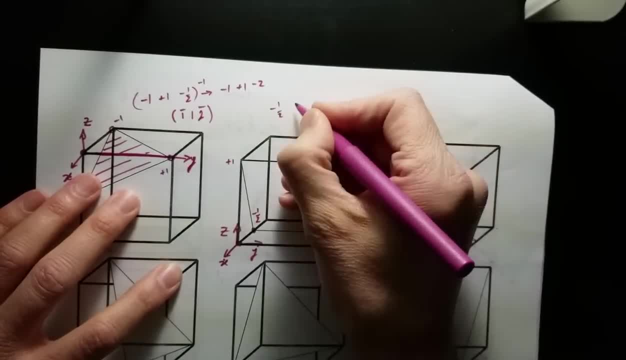 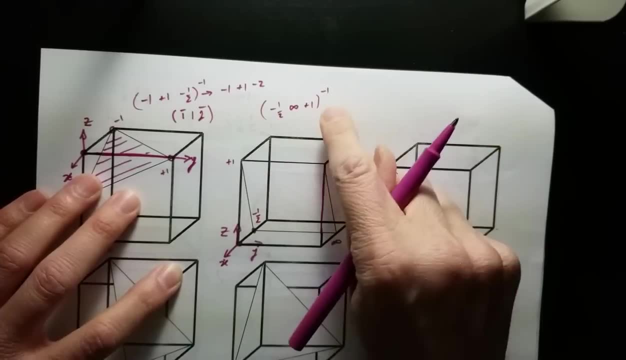 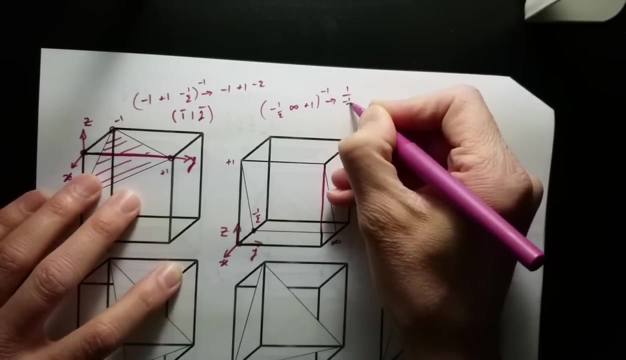 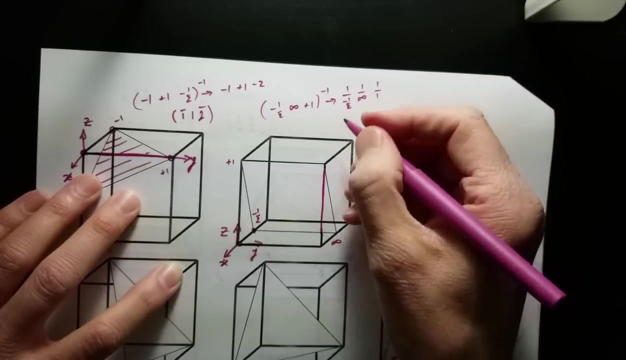 So we have minus 1 half infinity plus 1.. We take the inverse of that So we get you know 1 over minus 1 half, 1 over infinity and 1 over 1, which gives us minus 2, 0, 1.. 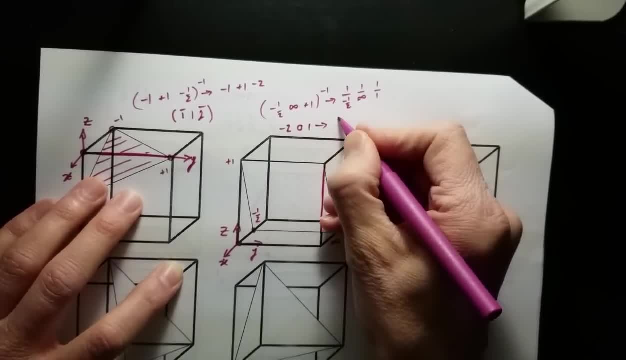 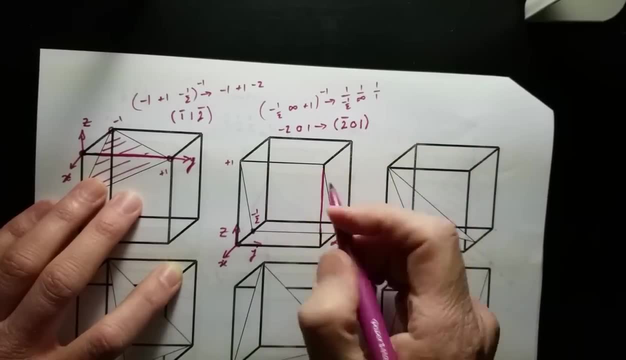 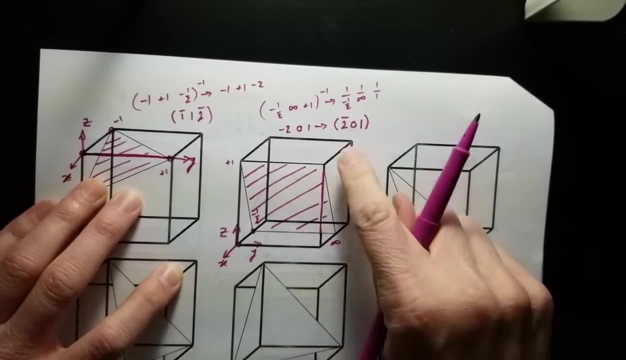 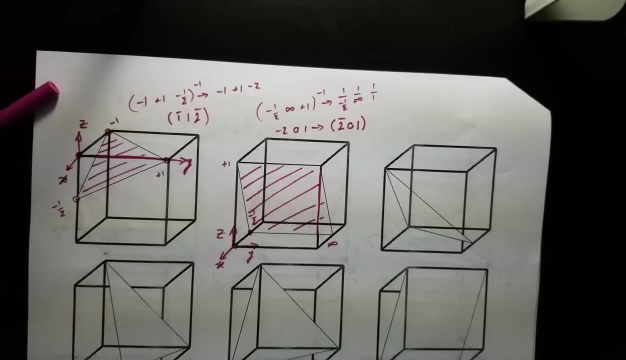 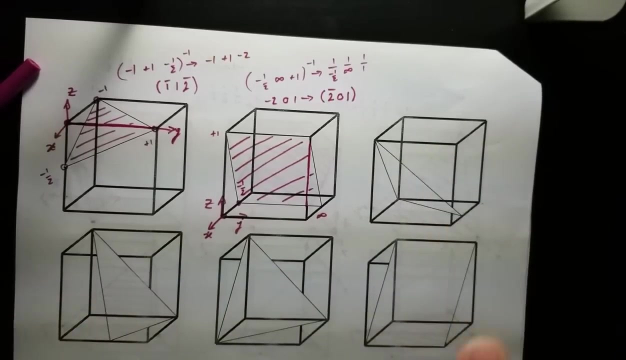 And putting that in the proper notation: 2 bar 0, 1.. So this plane is the 2 bar 0, 1 plane. Okay, let's do one that's a little more tricky. I would say that this and this are both a little bit more tricky than the others. 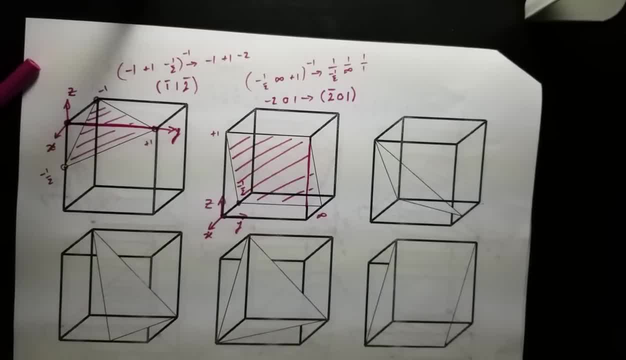 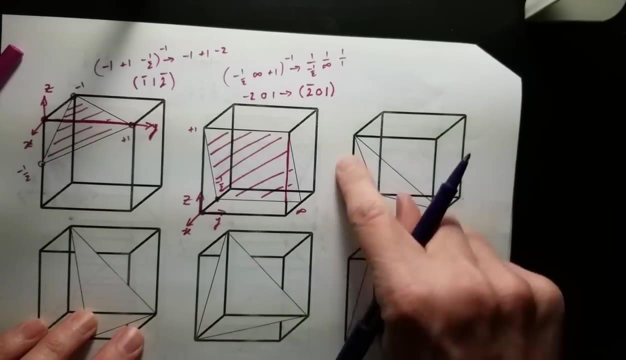 And the reason they're tricky is because you have to translate them. You have to translate the plane slightly in order to get the right answer. So let's look at that. Now. I'm trying to pick an origin And it's like: well, I can't really pick one there. 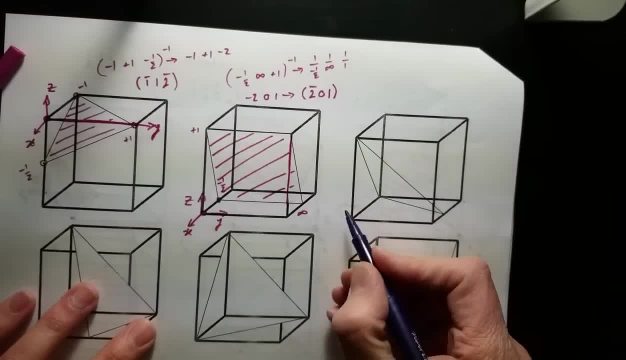 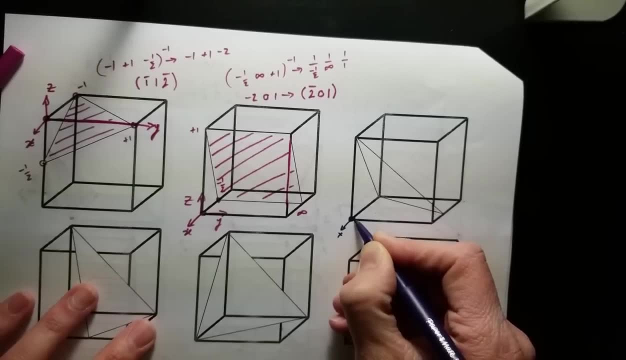 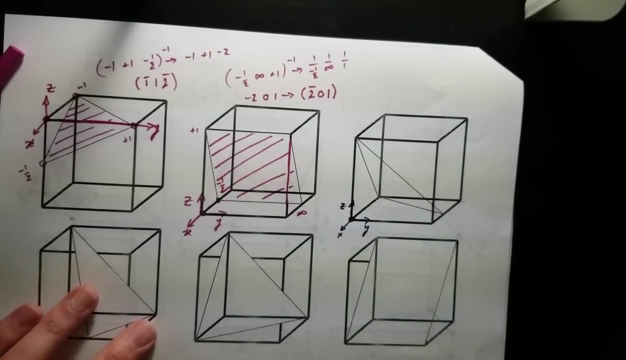 It doesn't cut. And it doesn't cut there, Where does it cut? Well, this seems to be about the closest I can get, If I were to put my axis here: x, y, Z, And that's the closest I can get. 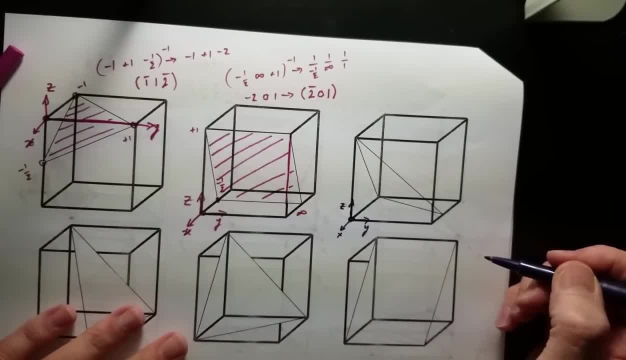 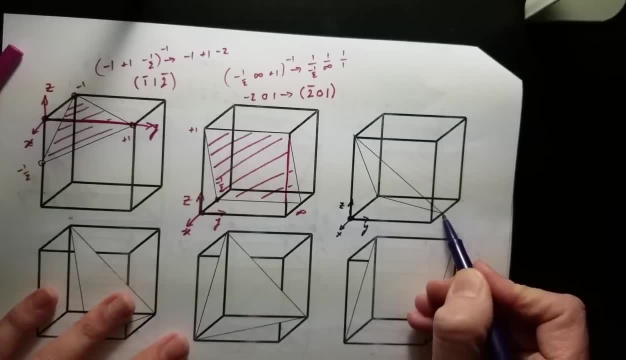 Now one way that I could determine where it cuts, because it cuts the x there and it cuts the z there, But the y. well, one thing I could do is I could extend that, And that's what I showed in class. 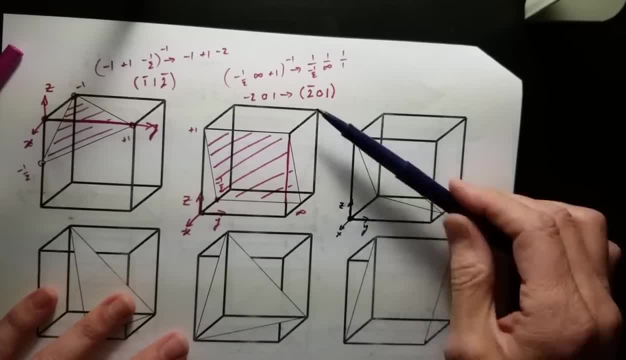 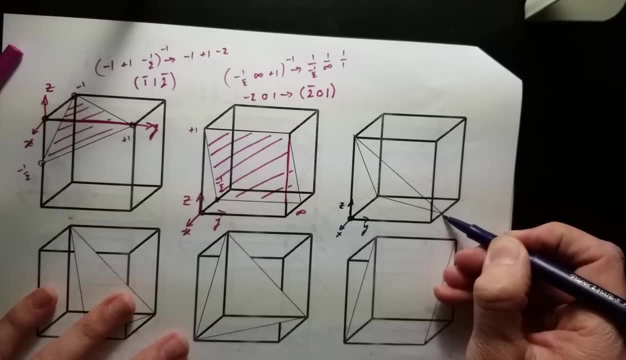 Another thing that I can do is I can take this entire plane and I can rigidly shift it. So, for example, If I could shift this entire plane by, say, I don't know, one-third in that direction, That looks kind of like one-third. 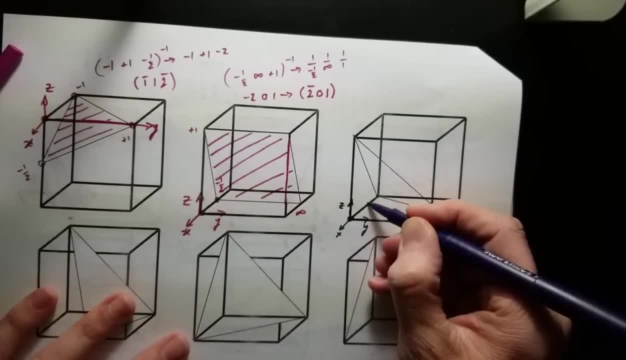 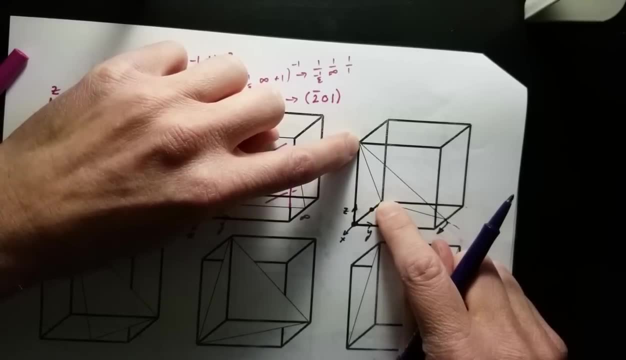 Well, what that's going to do is it's going to shift that one-third, It's going to shift this one-third And that line. if you look at that line, it cuts right through the center of the diagonal. Well, that means that if that distance is two-thirds, so is this? 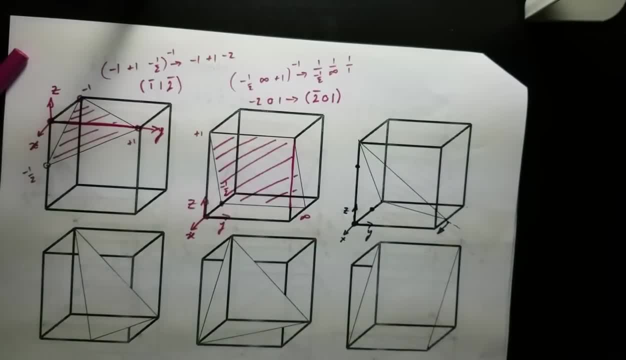 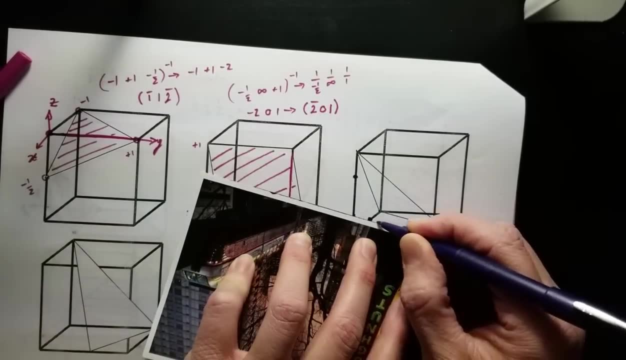 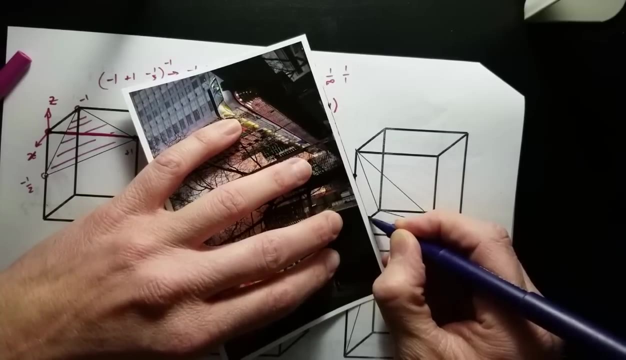 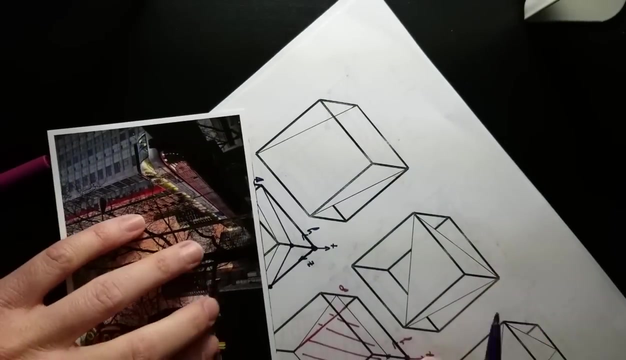 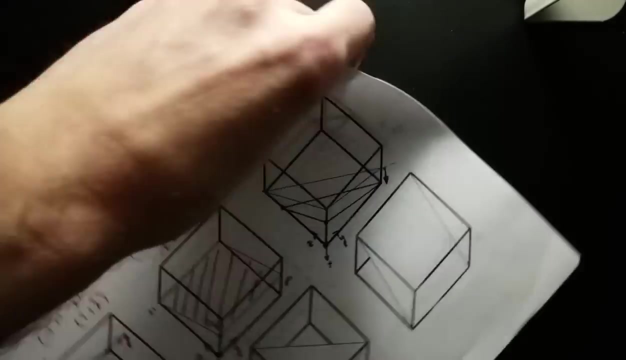 So what I'm essentially doing is I'm shifting my plane. See, Those lines are parallel And these lines are parallel, They're parallel, And then also, Like that, There we go. So now I've got a plane which has just been rigidly shifted. 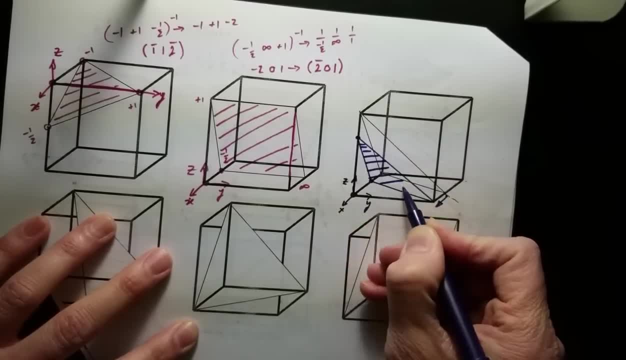 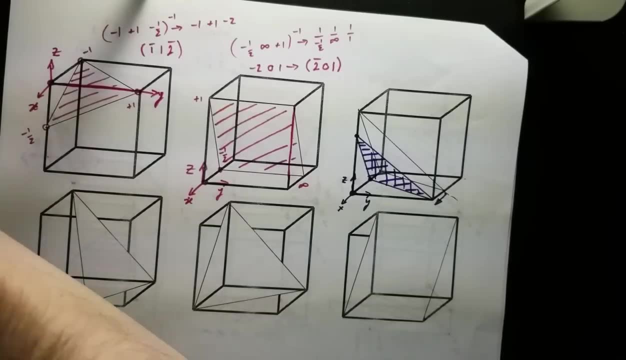 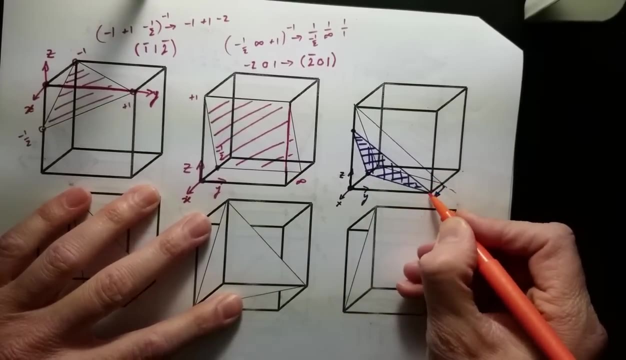 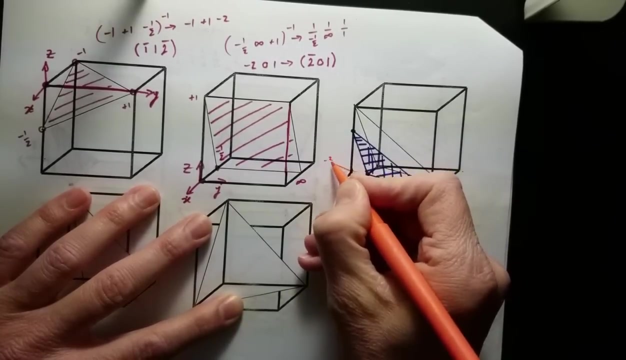 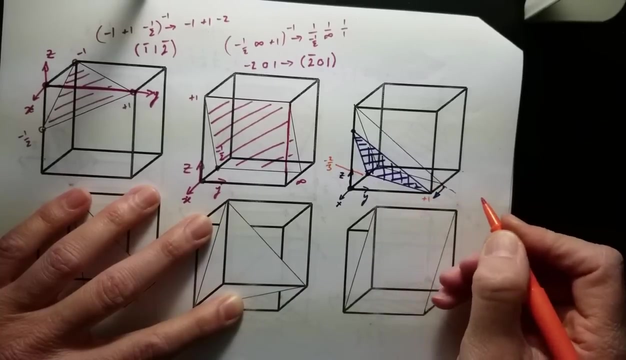 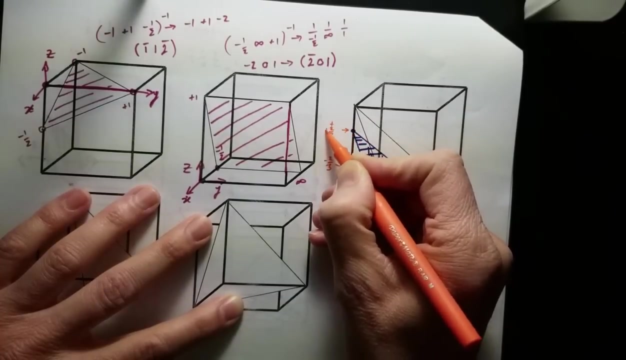 Here And when I had that shift. now I have an x-intercept that is two-thirds, So that's minus two-thirds. I have a y-intercept which is plus one And I have a z-intercept which is plus two-thirds. 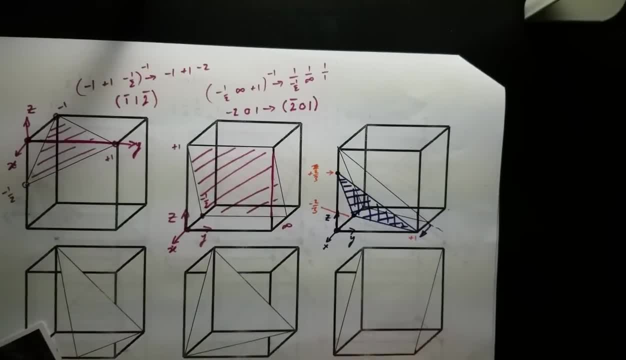 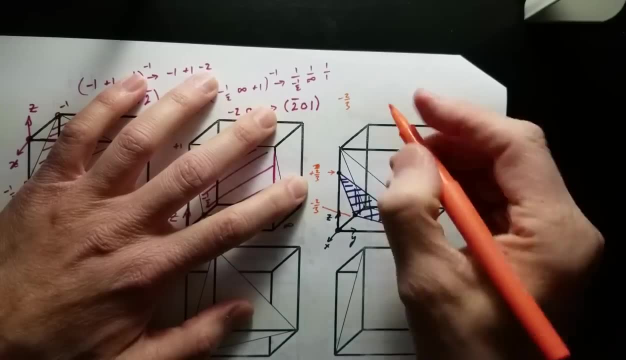 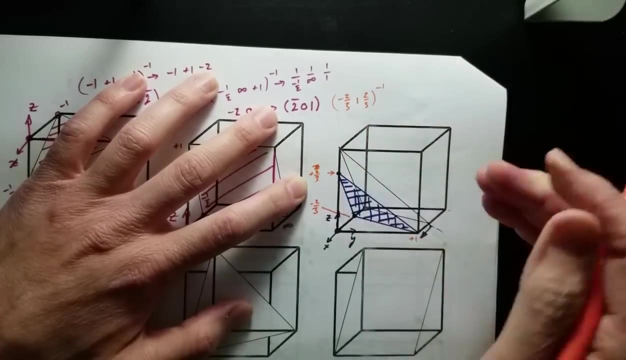 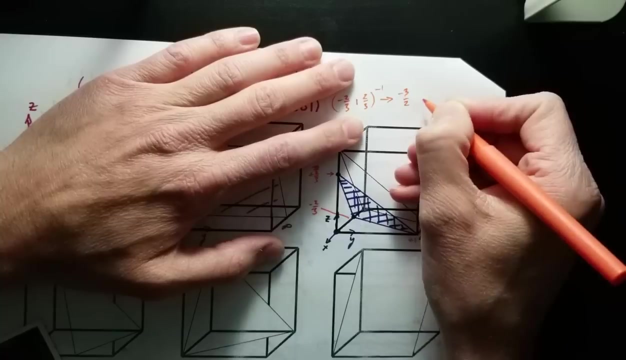 I hope you can see that It's plus two-thirds. So okay, Let's put this out. Let's say minus two-thirds, Um, Plus Plus one, Plus two-thirds. Take the inverse of that, So I'm going to get minus three-halves. 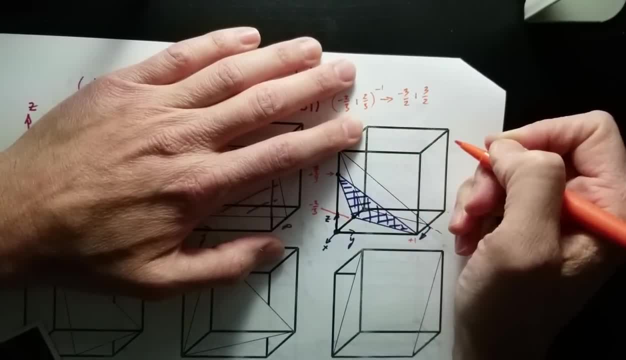 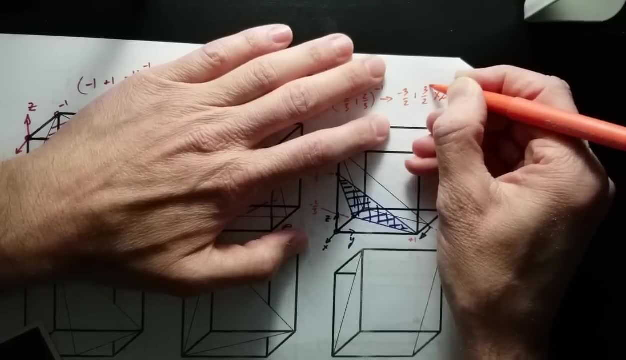 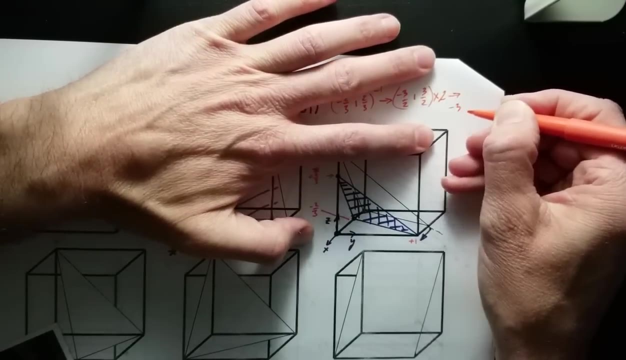 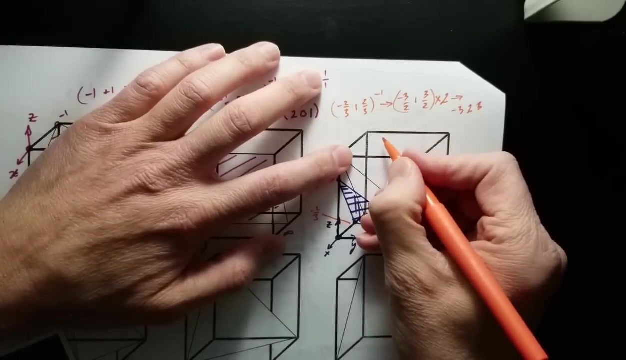 One, Three-halves. We don't want fractions, Right? So we're going to take this entire thing, Multiply it by two To get One Minus three, Two, Three. So the notation in the proper notation is going to be three-bar two, three. 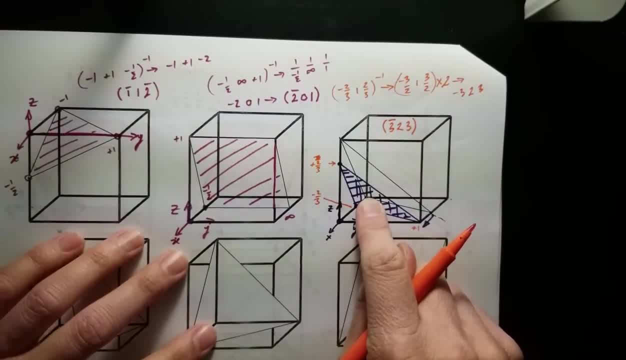 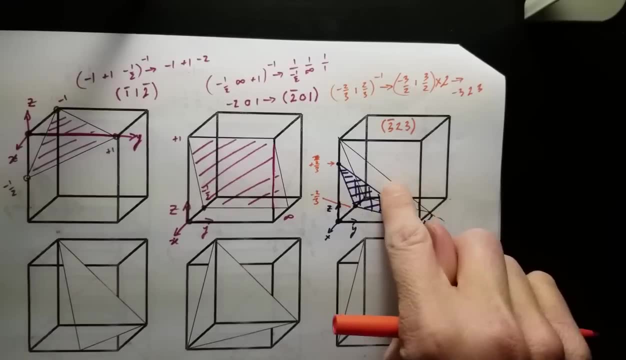 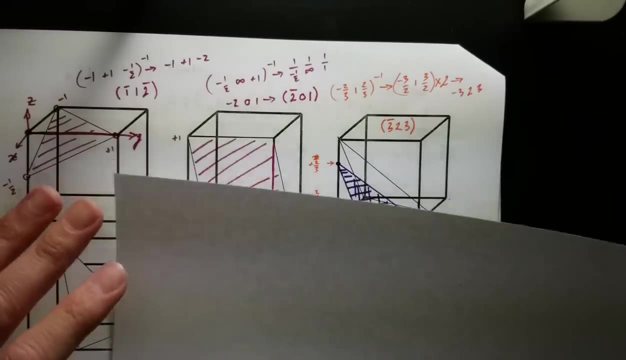 And that's this plane. I want to point something out to you, though. So this is our, Our plane. I want to point out that we can go backwards now, So I'm going to trace, Uh One, these planes on a blank sheet of paper. 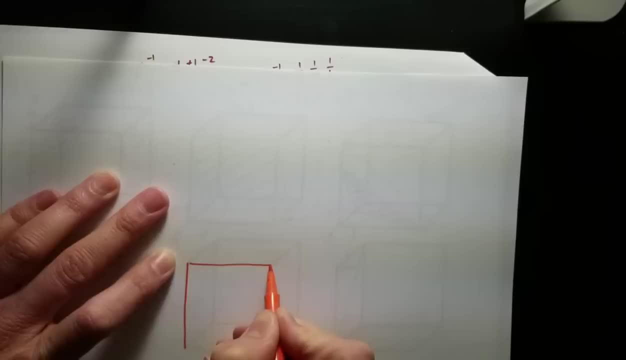 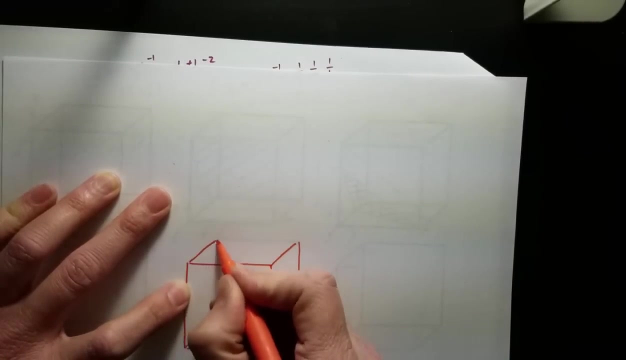 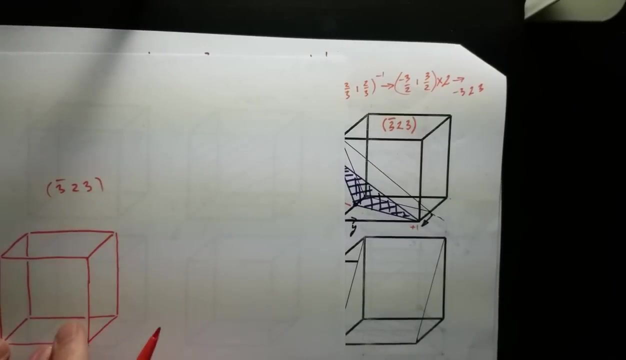 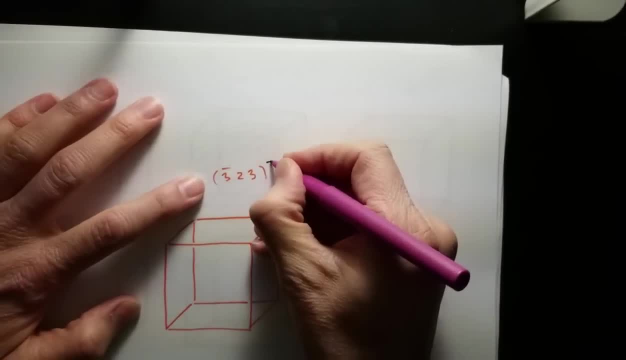 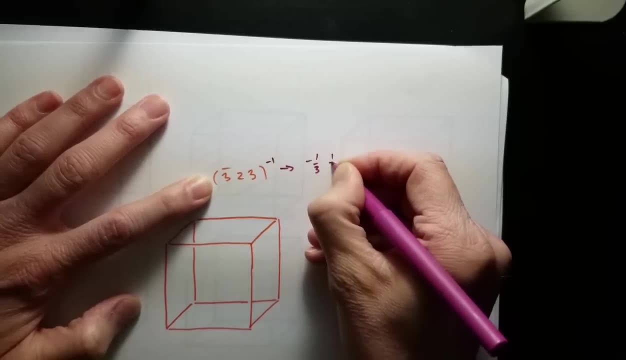 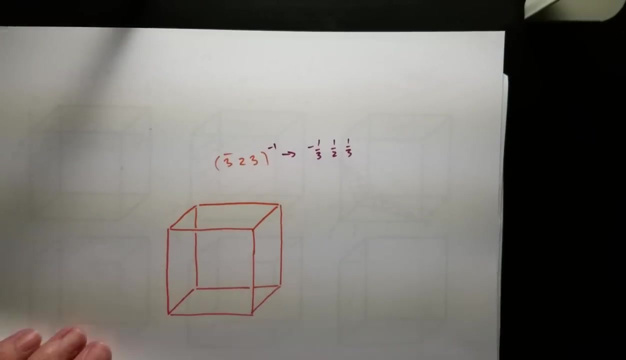 Okay, if we do that, first thing we do is take the inverse, so that gives us minus one third, one half one third. Okay, how do we get at that? Well, we know we've got to cut the x at minus one third. so that means we want to be in. 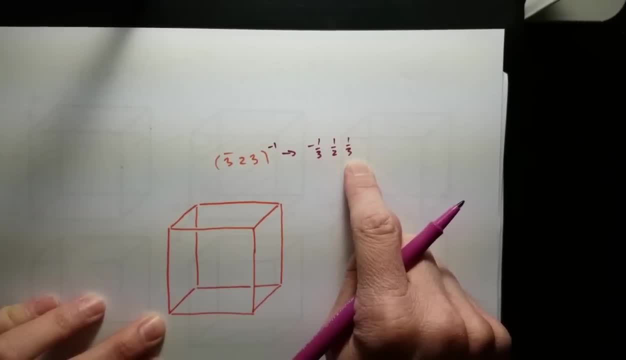 this front plane and plus y and plus z, so we'll pick this as our origin and that means that I've got x, y, z, Okay, And I cut x at minus one third, which is right here. I cut y at one half, which is right here. 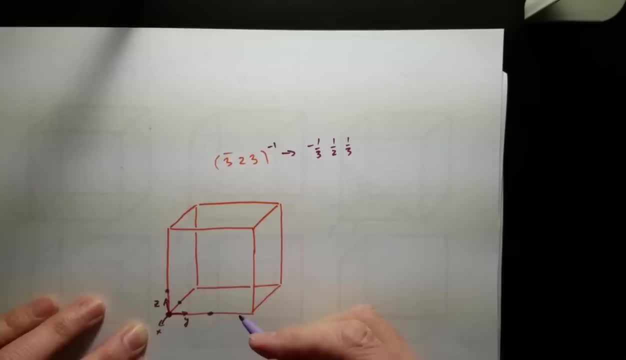 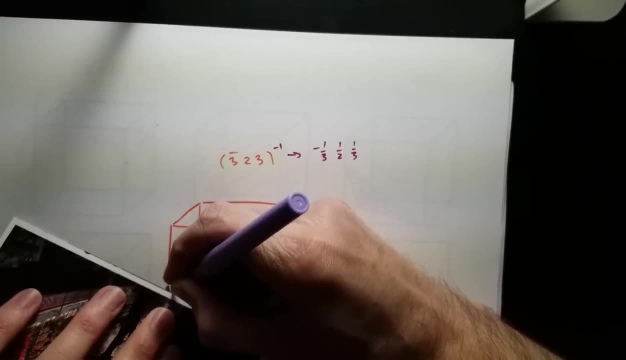 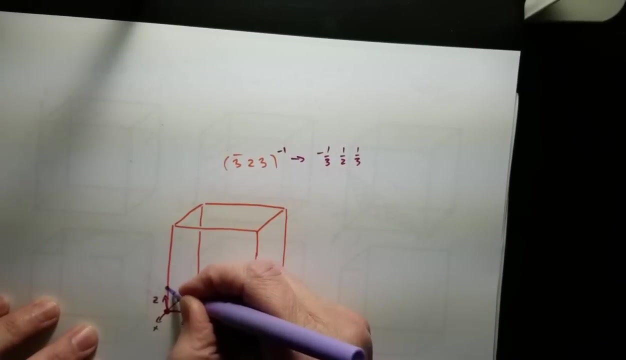 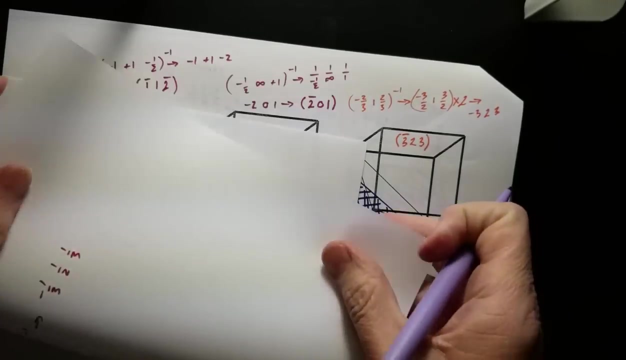 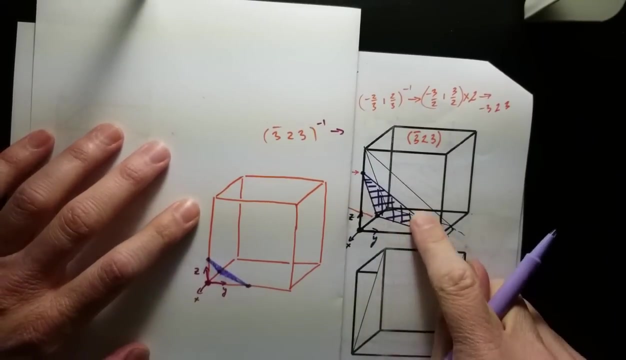 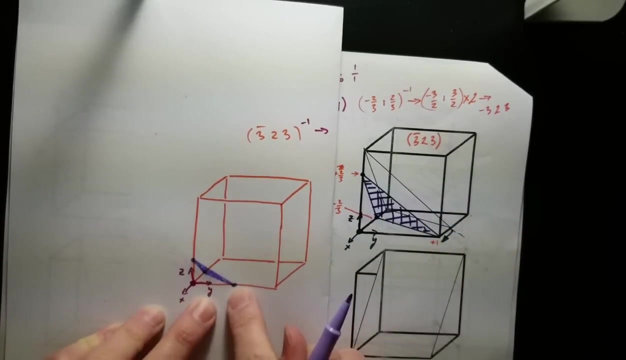 And I cut z at one third, which is right here, So trying to draw this in, That is our plane, Okay, So what I'm hoping you can see, though, is that this plane, which I had drawn originally, and the second, which is the shifted plane, and the third, which is the one I just drew, 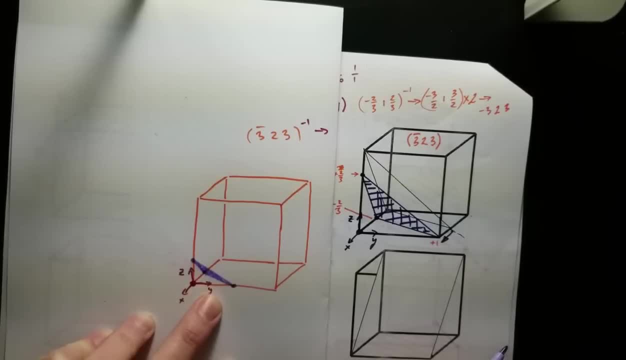 those three planes are all parallel to each other, Right? So if I take this plane and I shift it Right, It's going to be rigidly outward. so this goes by, you know, cuts that corner. Well, that cuts that corner multiplied by two. 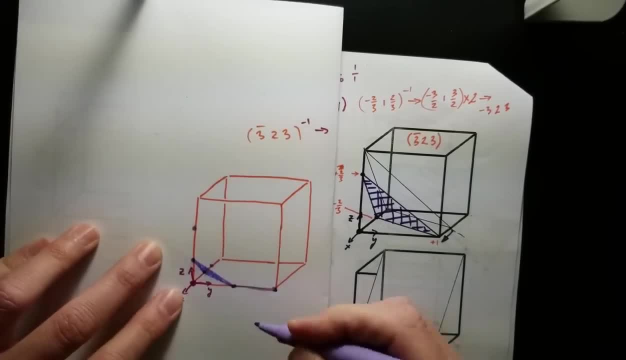 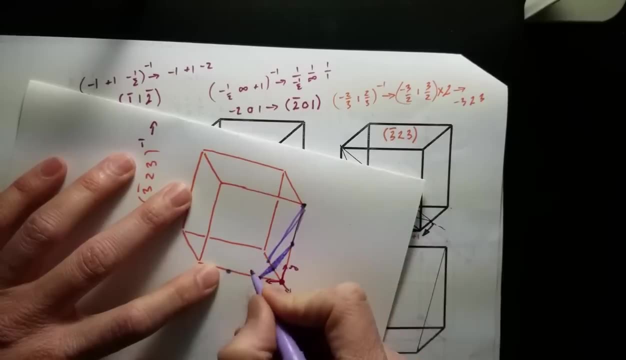 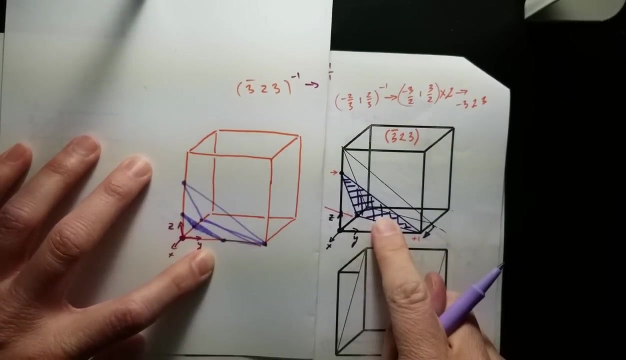 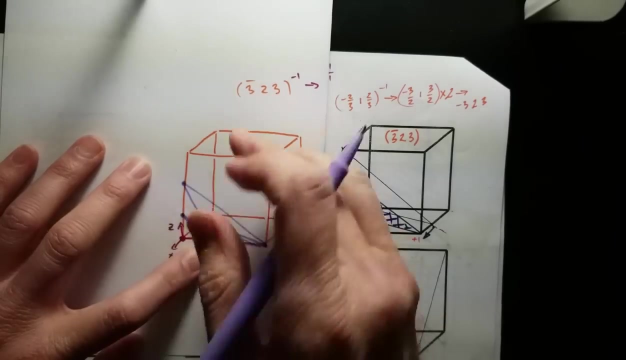 Then this gets multiplied by two. This gets multiplied by two, And now, pardon my terrible drawing, but I have that plane which is the same as this. Okay, So when we're identifying the planes, we're actually identifying all of these planes that. 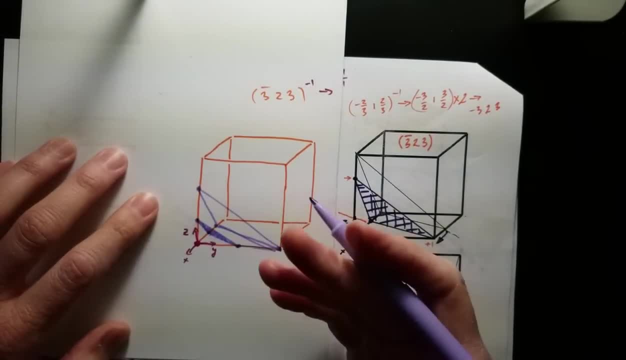 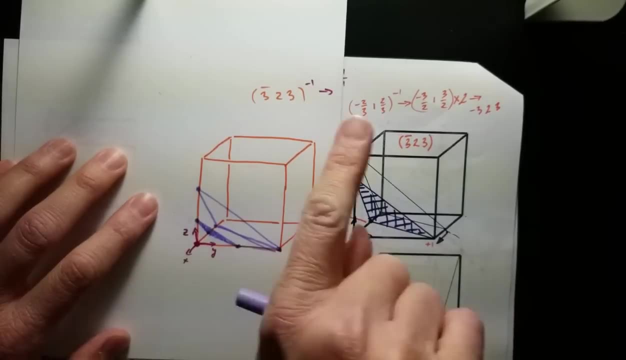 are parallel to each other. So, just as in the directions I said, you imagine yourself looking in the direction and, regardless of where you're looking, you're looking in the same direction. when you think about looking at planes, you actually can imagine yourself looking in the same direction. 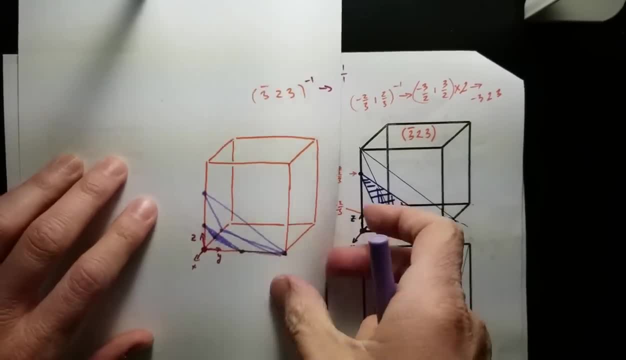 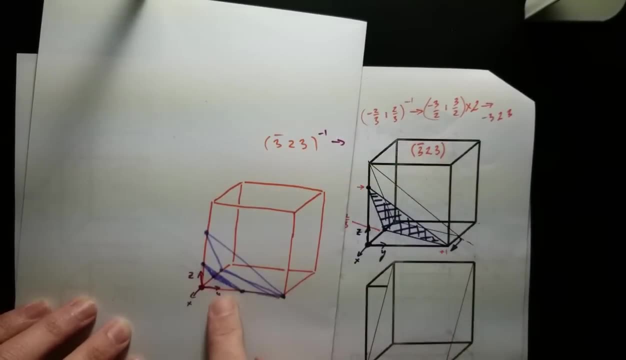 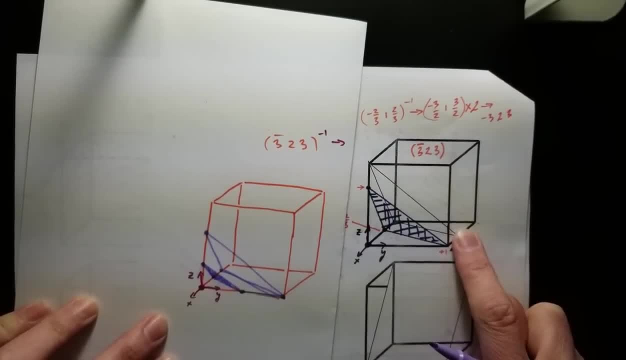 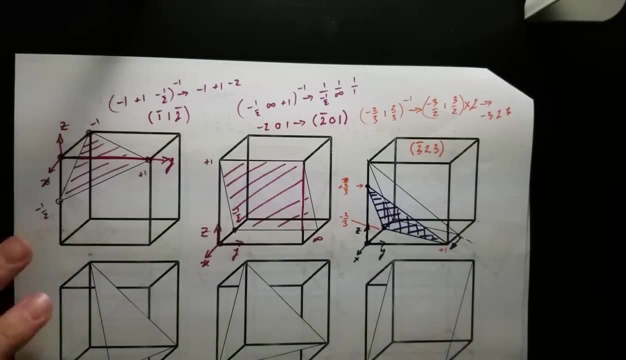 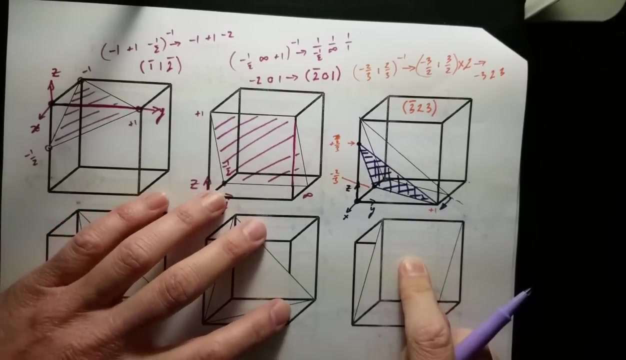 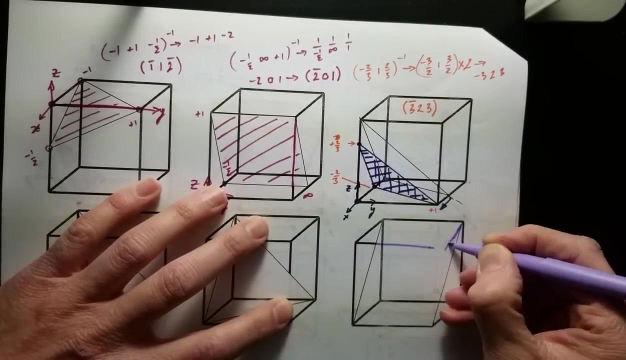 here, And that means that we can identify it by any of those Right. It'll still be okay. Okay, So let's draw in this plane next. Again, I'm very sorry if he's being disrupted the way they are, but fortunately you're. 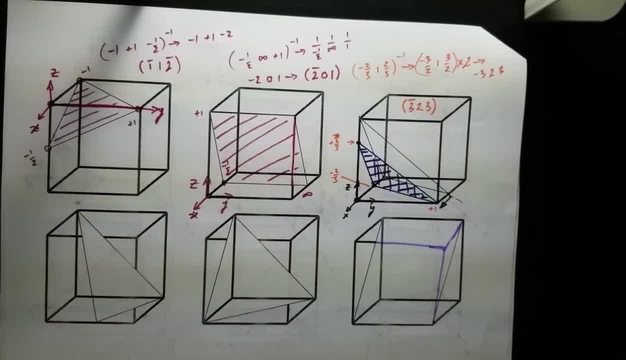 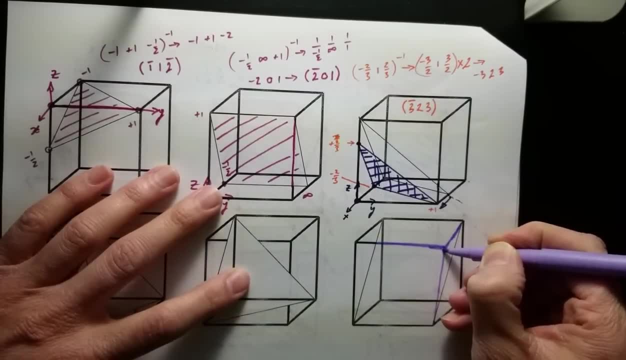 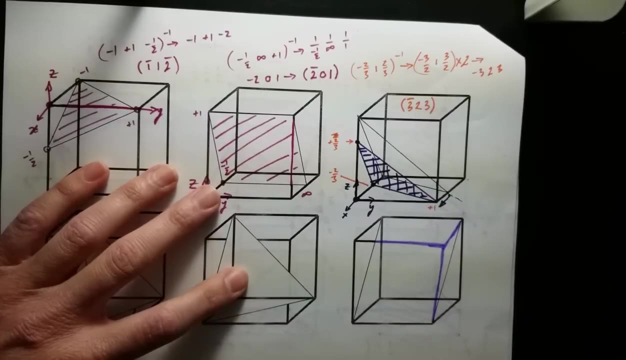 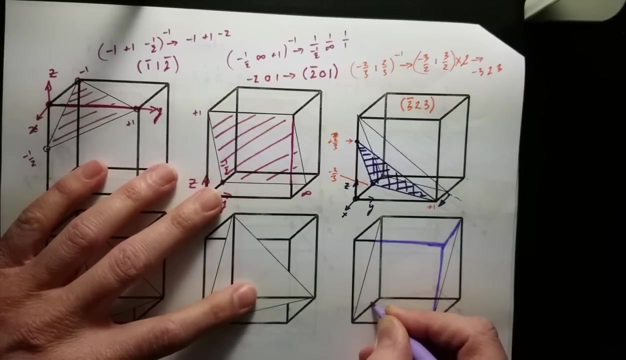 engineering students, which means that you're supposed to have Okay to have the ability to infer content from what you're given. Okay, So that's our picture, You know, picking an origin, the back corner. that seems to make a lot of sense. 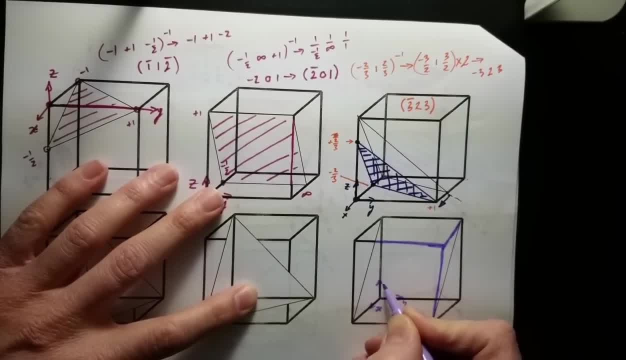 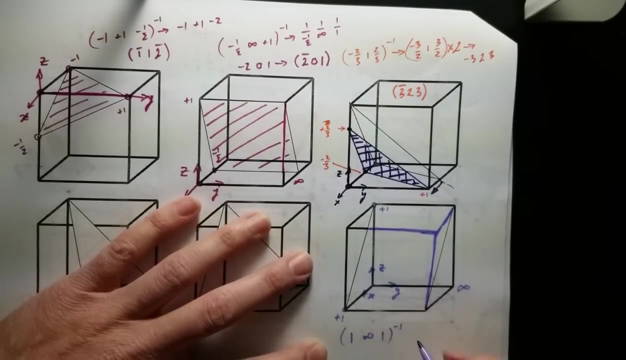 X, Y, Z. Cuts X at at plus one. cuts y- well, it doesn't, so it goes to infinity. and it cuts z at plus one, which means that we have one infinity one. take the inverse, and we have one zero one. 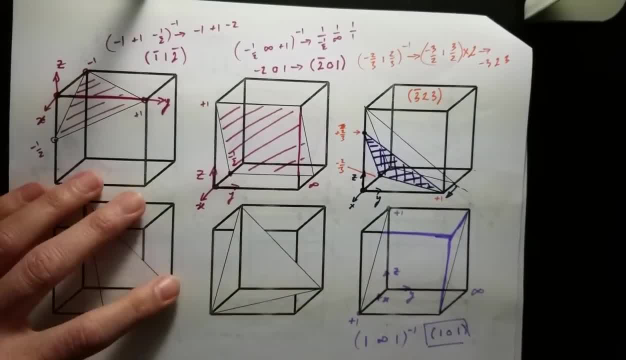 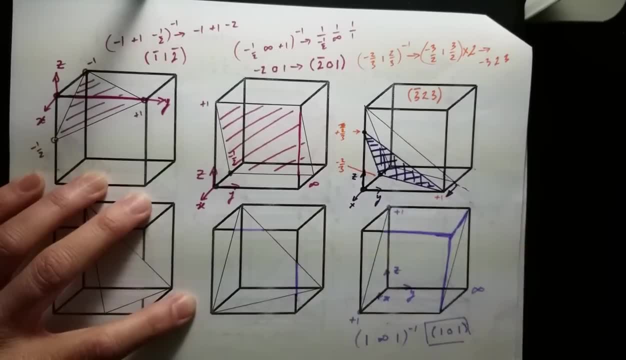 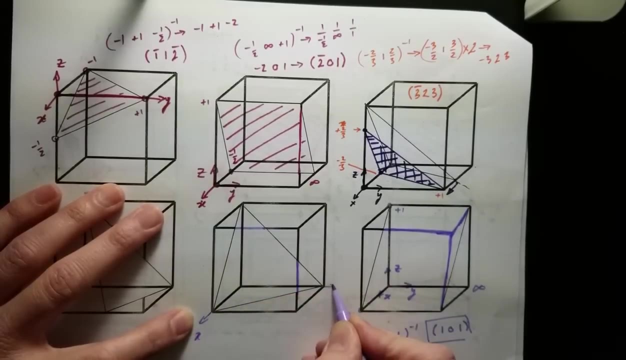 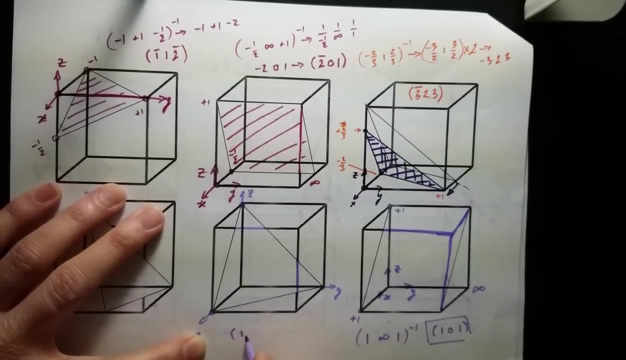 That's our solution for that plane. Next plane: X, y, z. it cuts x at one, it cuts y at one and it cuts z at one. so that's going to be one, one, one. That's our plane. 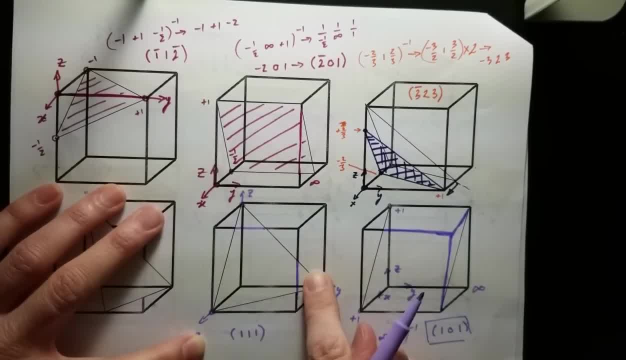 And I think we should know and note here that that one, one one. well, what if you draw the normal to that one one one. What line So remember from your multivariable calculus class, or what will be your multivariable calculus class? 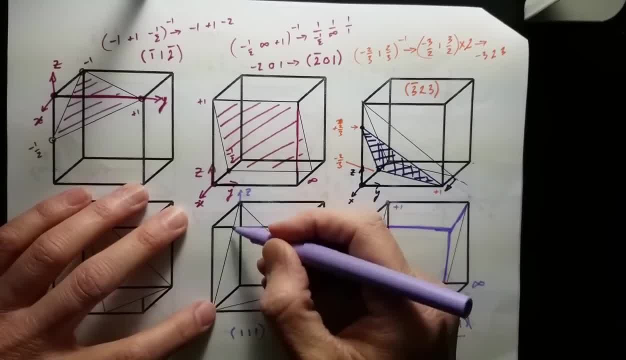 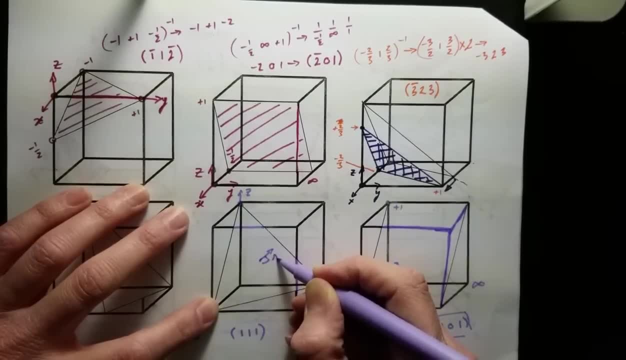 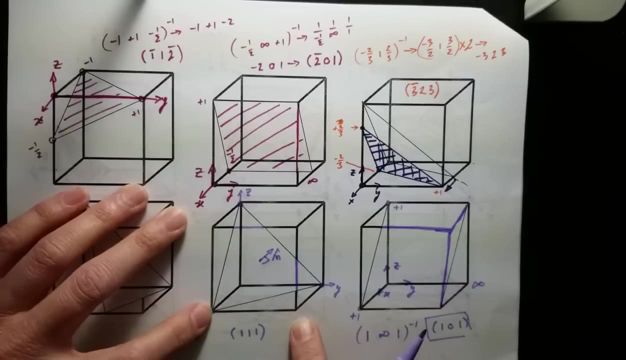 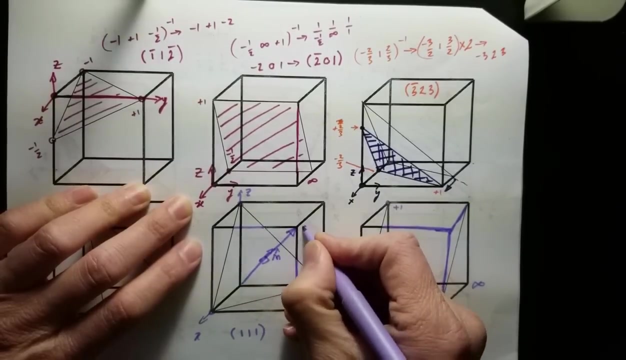 Actually you probably saw this in a trig- that if you have a plane and you've got a normal for that plane, that the normal defines the plane. well, if we have a cubic structure like this and we draw that line, it goes from one corner of the box to the other. that direction is 1, 1, 1. so that means 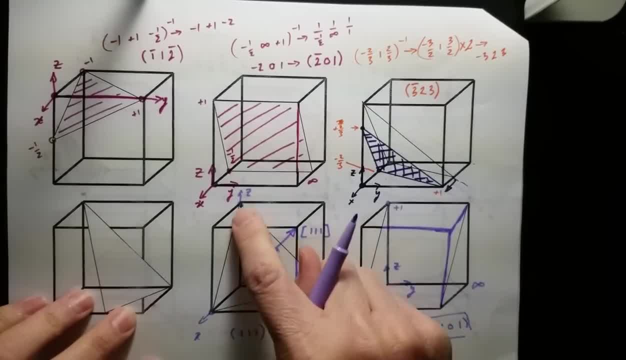 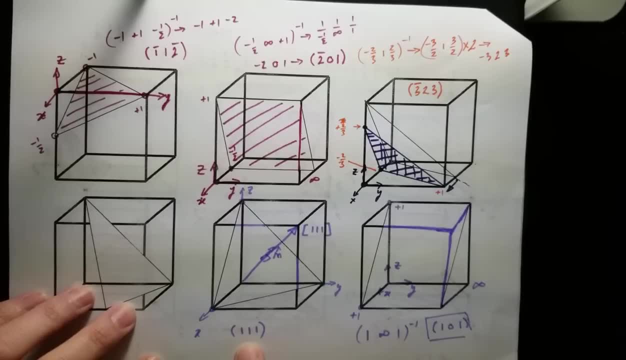 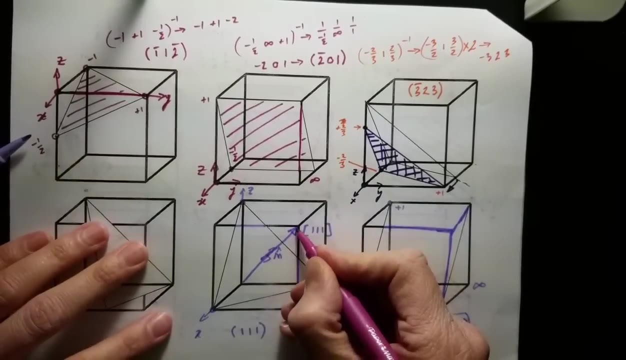 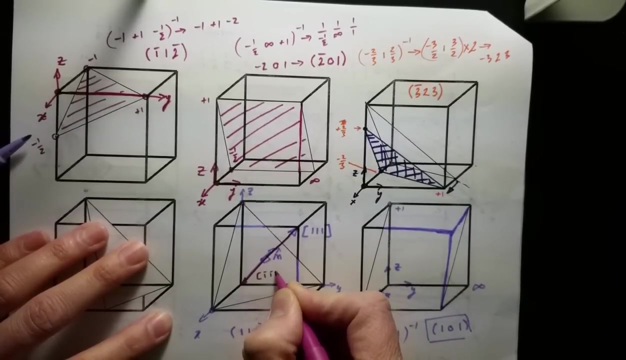 that the direction 1 1, 1 is normal to the plane 1 1, 1, and that's something that's actually pretty useful when we're thinking about crystals. interestingly, we can have another vector that goes from this corner through to that. right in that direction was one bar, one bar, 1 bar. 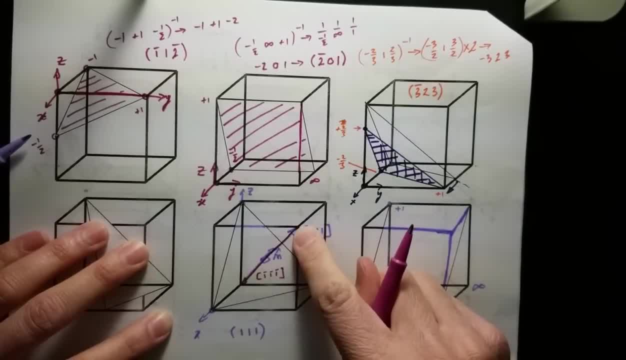 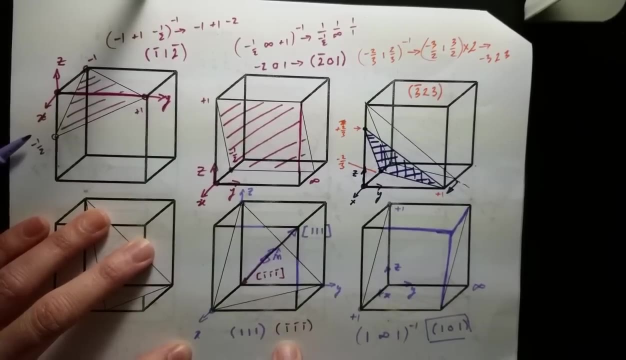 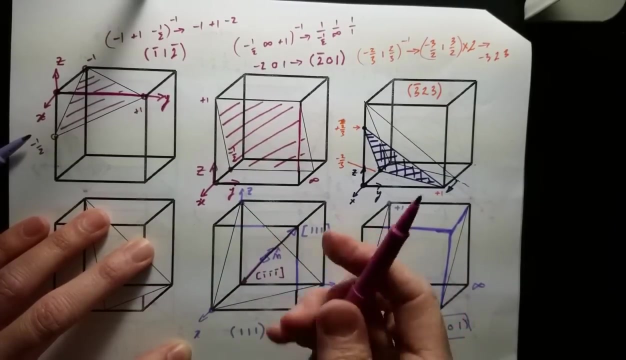 so we have two directions identifying the same plane. what does that mean? what means that the one one one plane and the one bar one bar, one bar plane are actually the same. so if I ask you to draw both those planes, you could draw them just once. and the difference is whether the 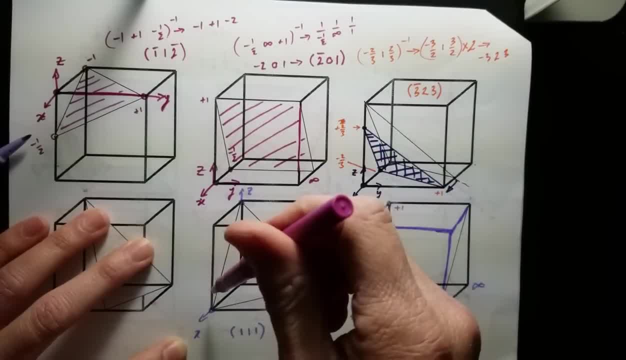 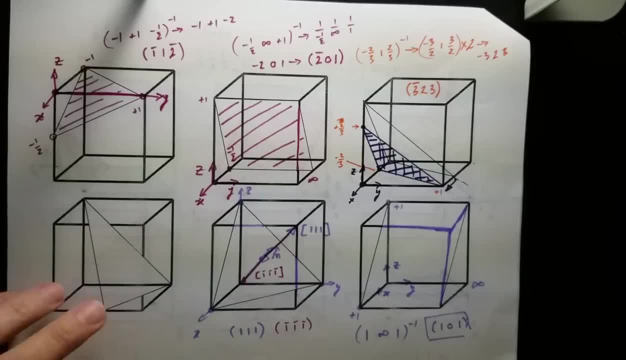 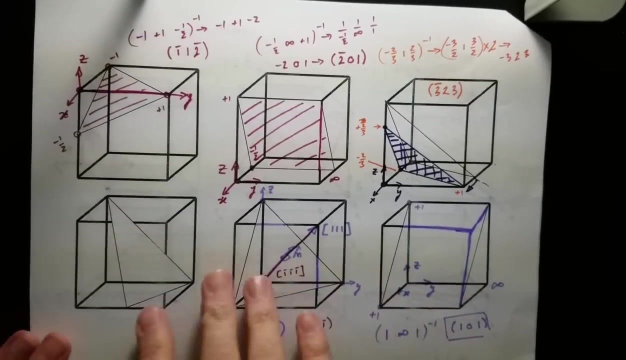 normal is going out or the normal is going in, so that that's something that's pretty handy. now, if you start going to geometries that are not cubic, then you have to start thinking a little bit different about it, but there's still ways to translate that, that basic principle, okay. so let's, let's go to this. 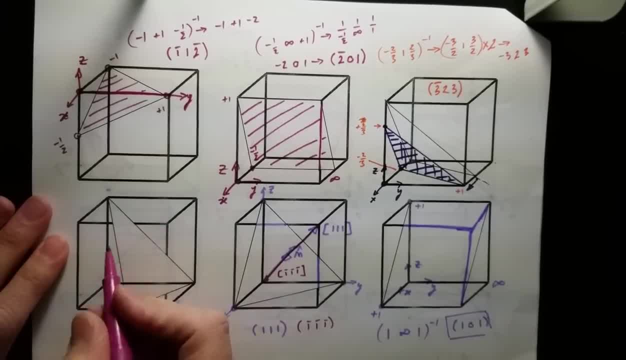 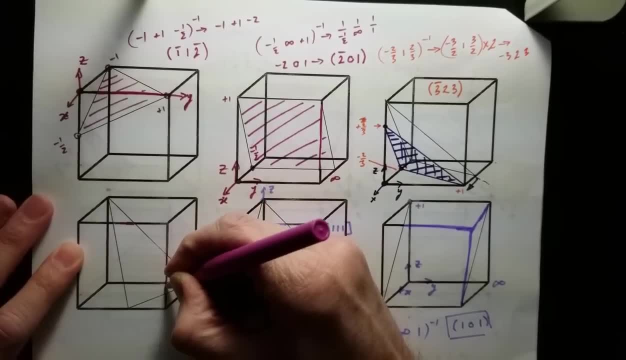 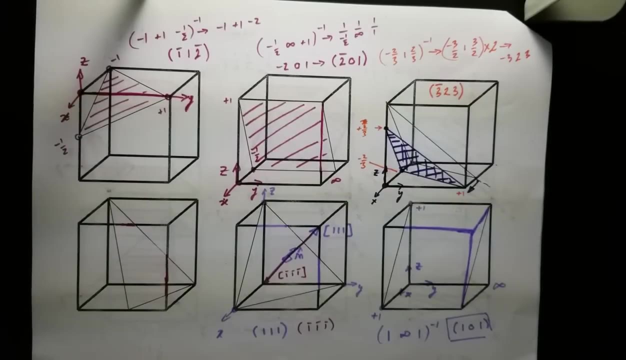 let's go to this last one, and I think this one, at least from my perspective, is one of the tougher ones to to do, so let me again fill in our gaps, and okay, so what are we going to do here? well, this, this looks like around two. 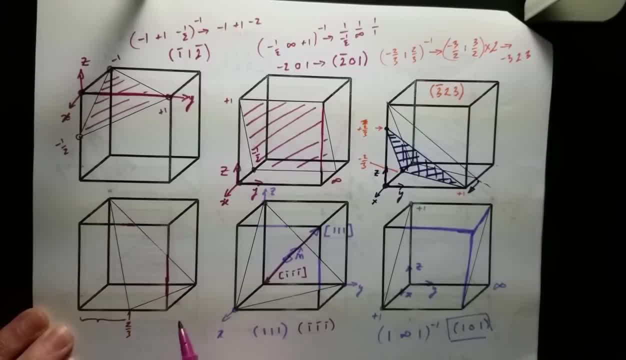 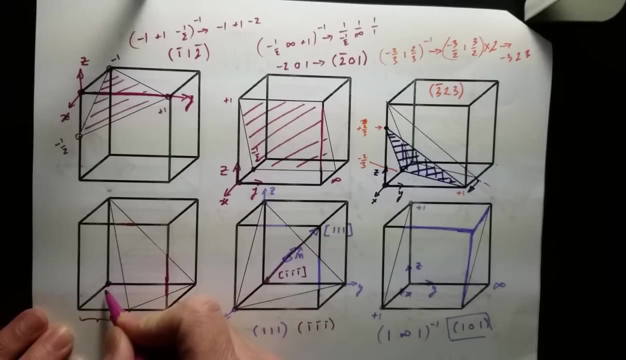 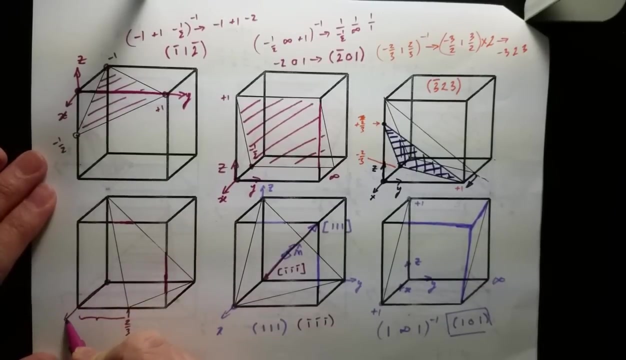 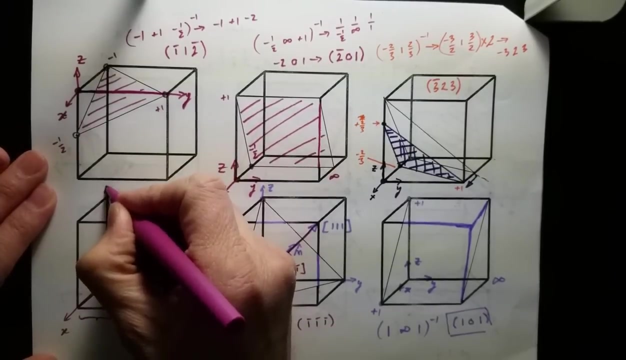 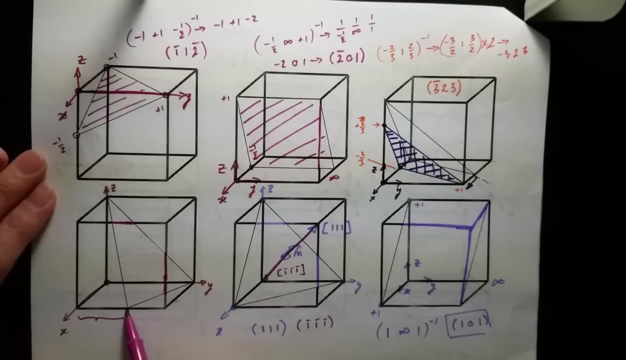 thirds of that distance. you know, I don't have any easy origin, but I think that possibly the easiest is to pick that back corner, and let's do that, let's find that as our back corner. so that's X, Y and Z, and now we're going to- I mean we could, you know, figure out where this intercepts by? 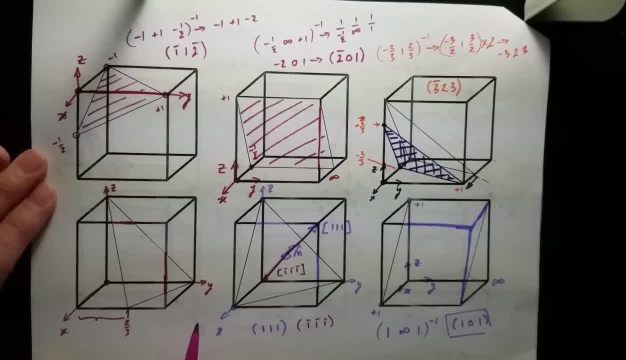 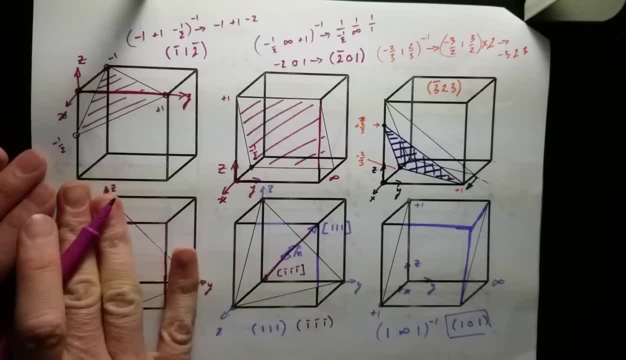 drawing it out. but I think what's going to be easier is for us to draw the same set of X in the same direction here. so let's just say Y is the third point and Z is the fourth point, so the first point here, so we can actually do a new. 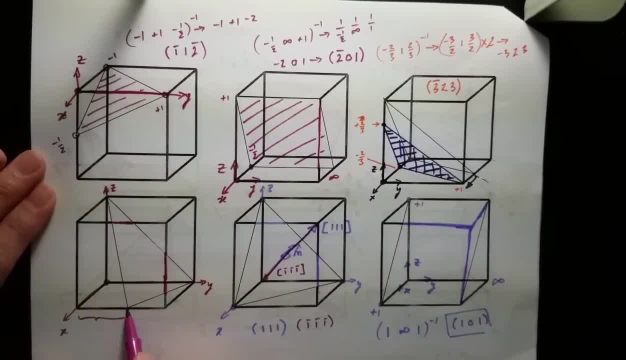 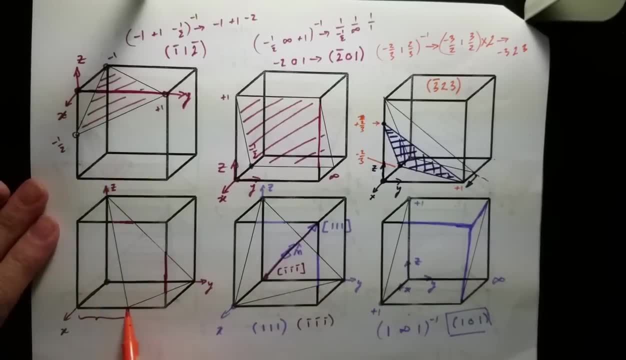 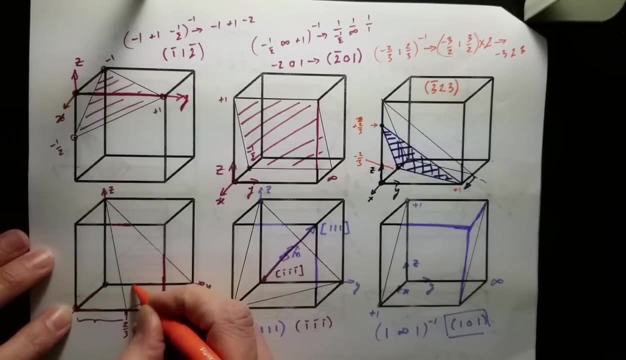 plane by shifting this, so basically getting a rigid shift by two thirds in the negative Y direction. so if we do that, then this becomes- let me pick a different color so we can see it better- This point shifts to here, The y point shifts two thirds, so it shifts here, and the Z point shifts two thirds as a whole.